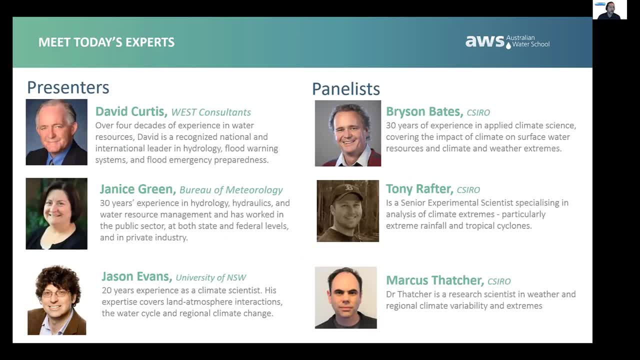 with you today. So with no further ado, let's introduce our presenter. We have got David Curtis from West Consultants, Janice Green from the Bureau, Jason Evans from the University of New South Wales, And then from CSIRO we have Bryson Bates, Tony Rafter. 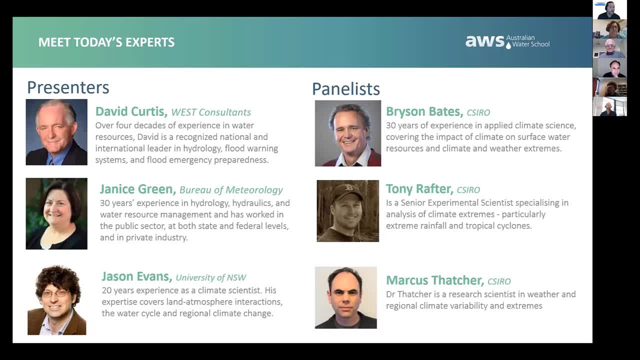 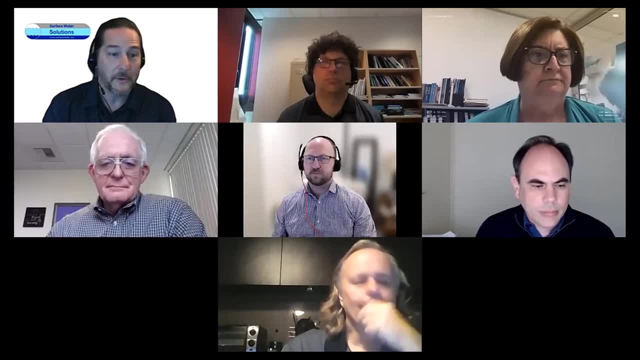 and Marcus Thatcher. So, with all you presenters and panelists coming on here, introduce yourself briefly and let us know where you're coming to us from. And let's start with you. David, You're on the West Coast of the US, I understand, or is that where you're coming to us from? 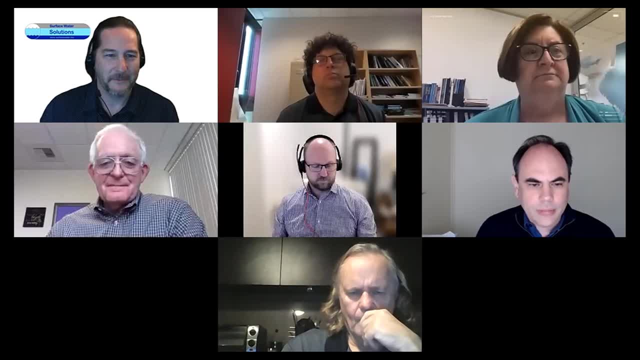 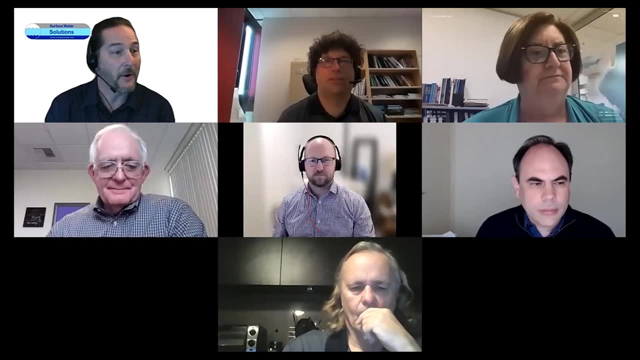 West Coast of the United States. correct, All righty, So in the late afternoon for you. Hi, David, Good to see you, Jason. and again this reads like, if you get into AR&R and just Google AR&R for Australian rainfall and runoff, climate change. 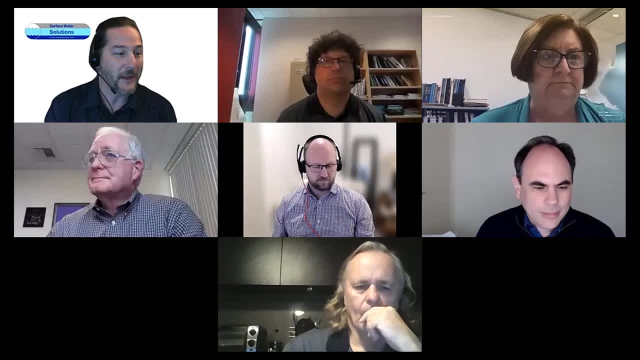 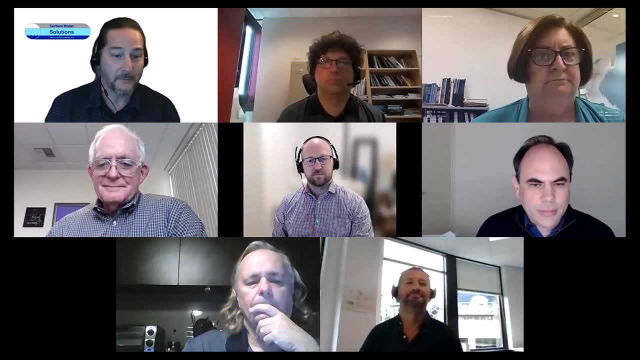 the author list. we've got some of the authors right here with us today And in the background, Clinton, feel free to turn on your camera as well. We've got some other experts on with you as well, Clinton, formerly with BOM and now with Tetra Tech. Good to see you on board as well, Jason. 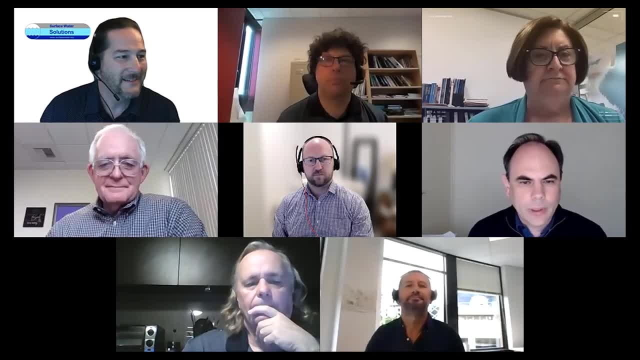 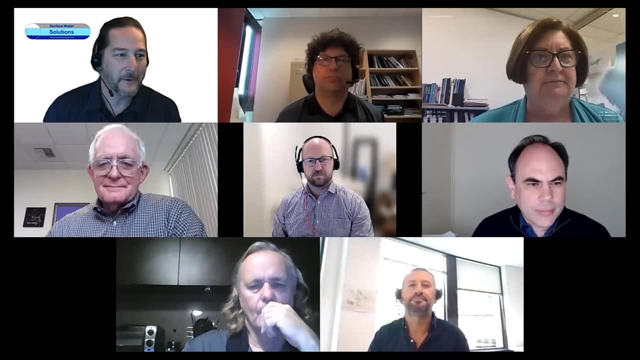 tell us where you're coming to us from. Hi everyone, So I'm coming to you from Sydney, Australia, at the University of New South Wales. Excellent, Good to see you there. Janice, where are you located? I'm located in sunny Canberra. I'm coming from the Bureau of Meteorology. 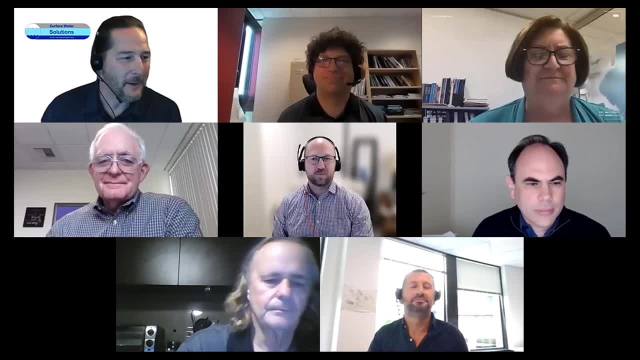 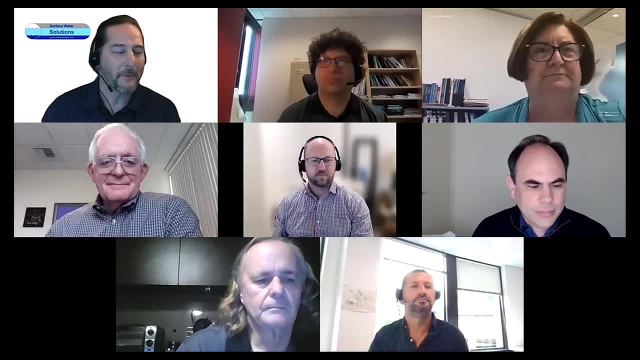 All right, I used to see a big BOM building in Melbourne, but we've got some in Canberra as well. Awesome to see you here. Then let's turn to our CSIRO. Am I pronouncing that right? I always say CSIRO, but let's start with Bryson. 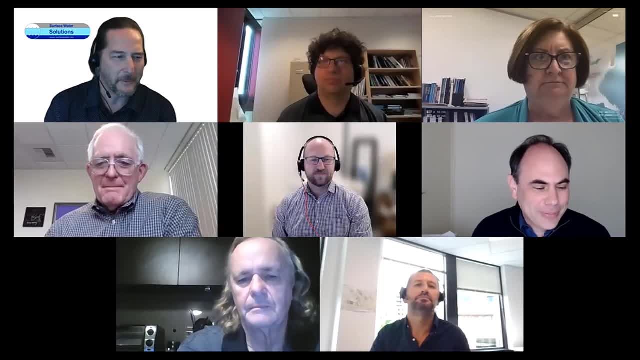 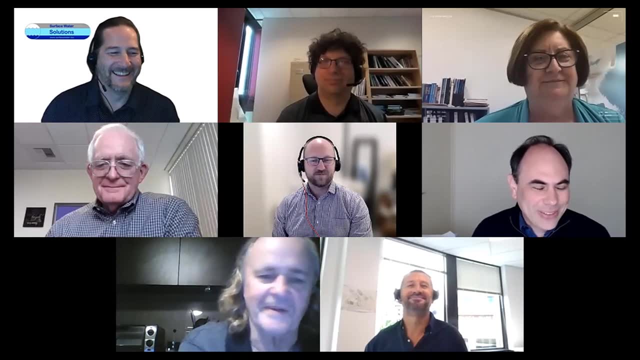 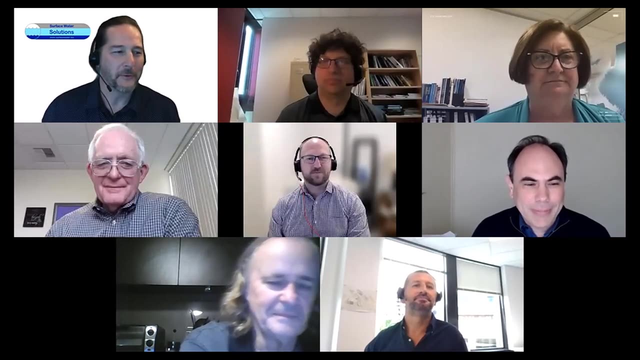 You can tell us where you're at today And tell me, am I pronouncing that correctly? I'm from Perth, Western Australia, And, yes, you are pronouncing it correctly. Some people say the whole acronym CSIRO, But yes, for those who don't know, that's a Commonwealth. 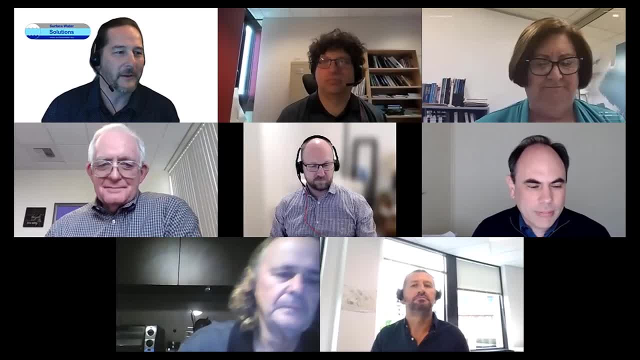 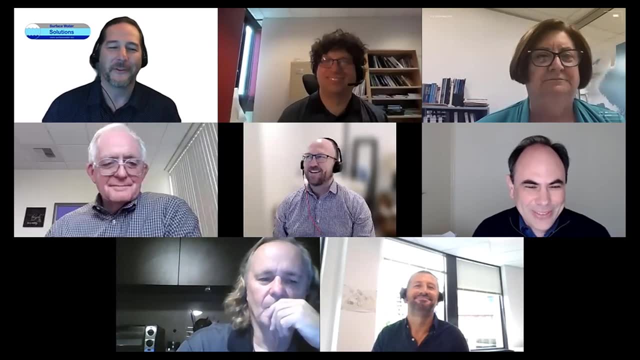 department for science, And that's something that actually I'll have. Tony, maybe you go next and tell us exactly what CSIRO stands for. I'm one of those attendees who are attending from around the world who have not heard of it in Australia. 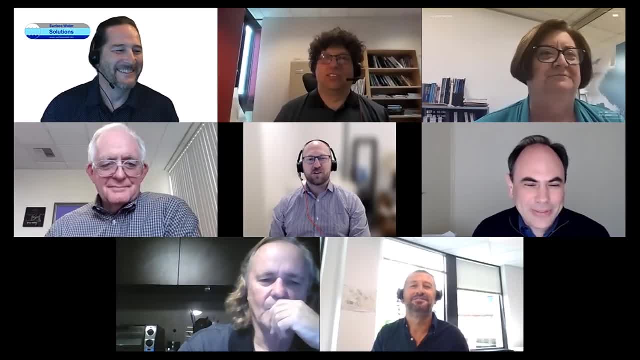 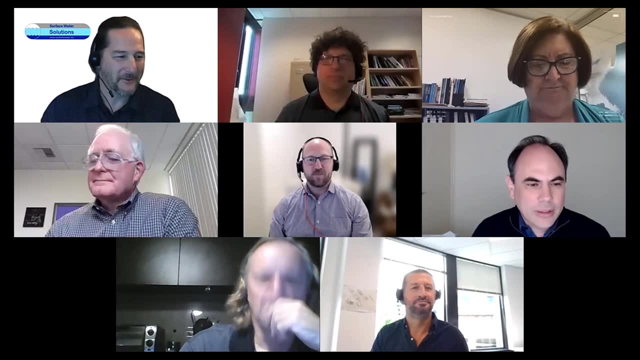 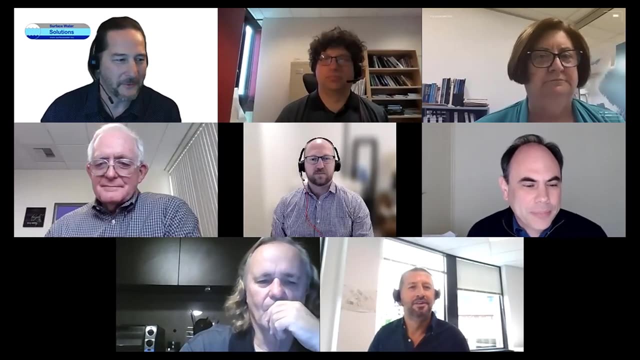 Commonwealth Scientific and Industrial Research Organization, So a government research agency. And I'm coming from Melbourne, Australia, Awesome. And Marcus, Yeah, I'm also from Melbourne, Australia, working at CSIRO- Excellent, Clinton, where are you coming to us from? 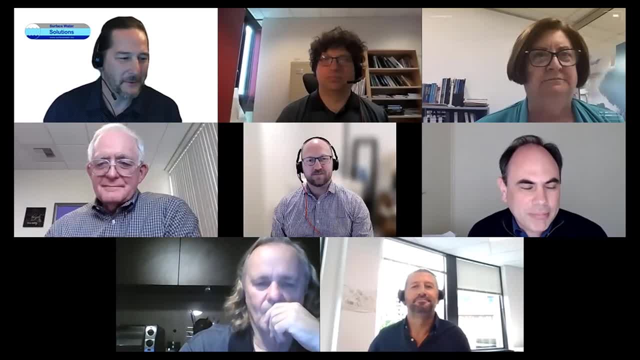 Good morning everyone. I'm from Sydney, Australia, Sydney, Australia. Well, good to have you on board. We also have the Australian Water School in the background helping out with your IT questions And making sure this runs smoothly. So I'll frame up one question And we'll have just a quick back. 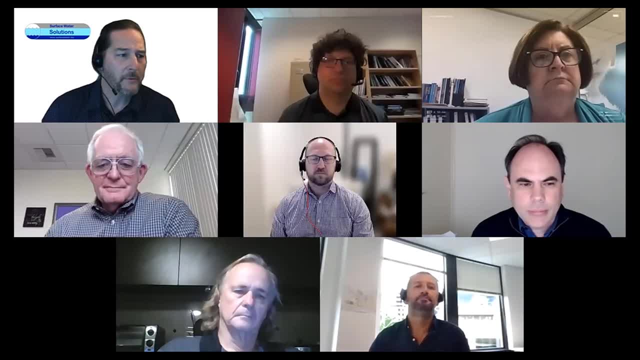 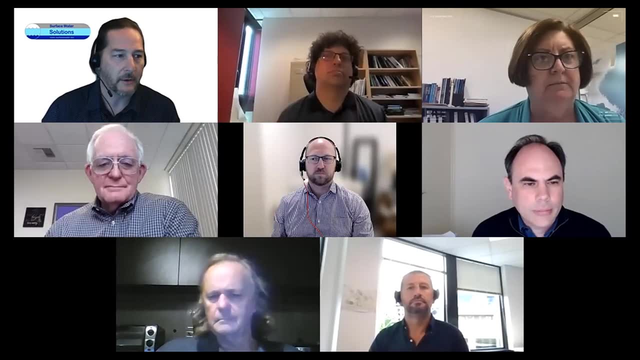 and forth among the panelists, And then we'll turn straight over to David. One of the reasons we selected this as a topic is that I'm an engineer And a lot of those attending previous AR&R webinars and other similar topics in the past through the Australian Water School again. 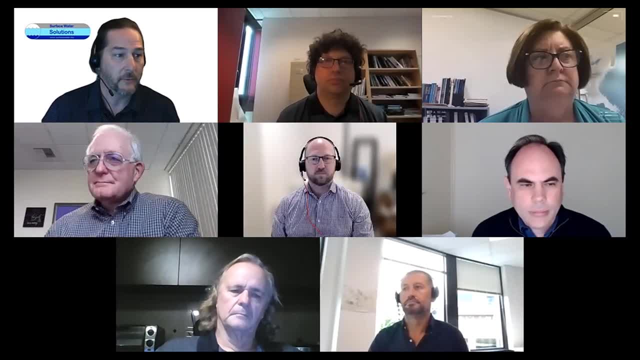 most are engineers. Many come from a background of trying to implement things from a practical standpoint. I get a lot of scopes of work from different agencies, whether they're from from council or from private mining companies, And it'll just say in my scope of work when I'm 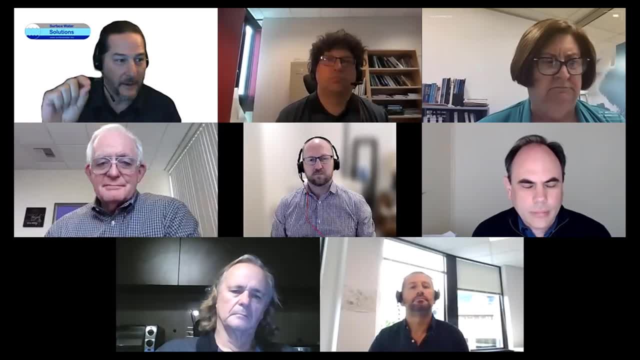 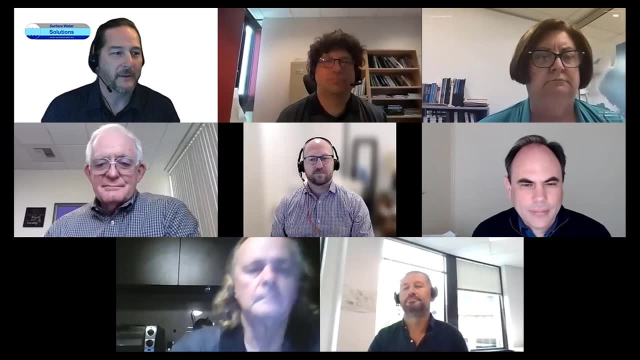 bidding on this and I'm saying I'm going to do this work for you. it'll say one line in there: incorporate climate change And that. that baffles me sometimes because I don't know, as a practicing engineer, how long is that going to take me? Can I just pull some number and say: 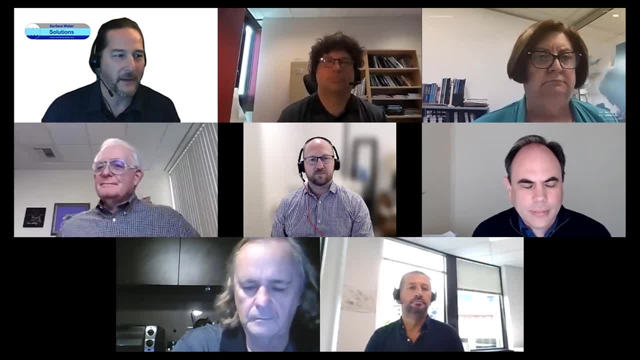 18%. I'm going to add this to my flow rate And, yes, I have accounted for climate change. Or do I need to do a lot more work? How do I bid on that And what do I do? So that's one question. 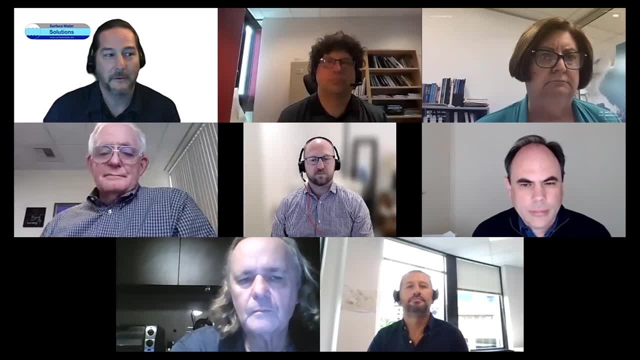 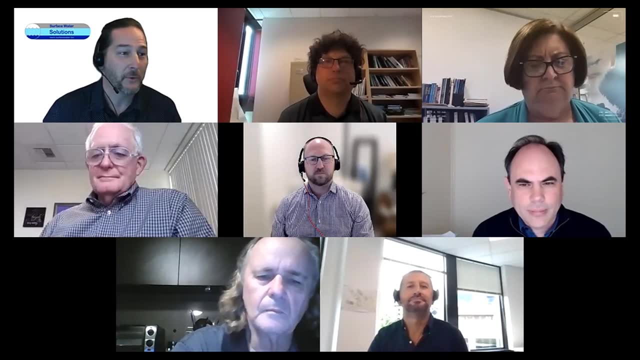 that I've had, And then lately, especially last week, I've been doing a lot of work on climate change, When Texas was freezing. I hear people on Facebook making comments like: wow, if it's this cold in Texas, then climate change must be going the other direction. So we're all good And let's try to. 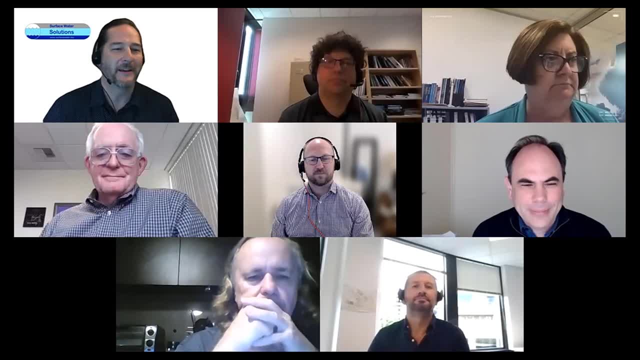 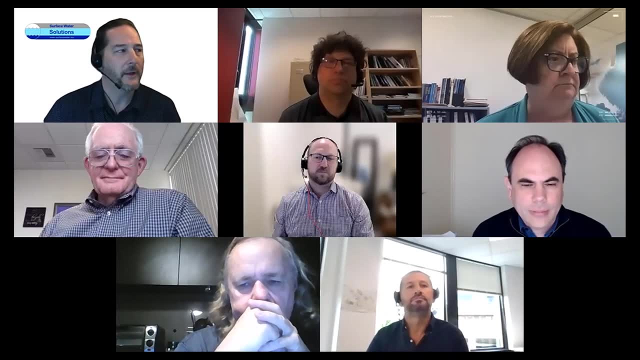 incorporate some science here and see why. why is that a comment? You know what? what can we say to, to somebody who might make a comment like that, And from a practical standpoint? a third question I'll pose here is when I see engineers looking at the climate change data and going to the science. 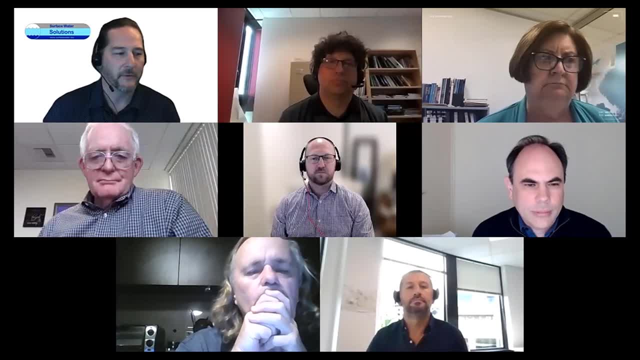 and they say: I want to look at the real science, you know, unbiased, I just want to see what's going on And I'm in an area I'm building a bridge and it's in an area where drought is projected. to increase, So rainfall is going to decrease. annual rainfall is going down. How come, when I incorporate climate change, I need to increase the size of my bridge? How come, for this three hour duration, I'm getting higher rainfall intensities where, over time, it's going down? 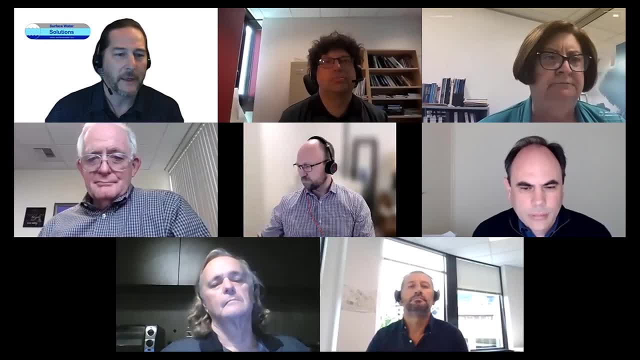 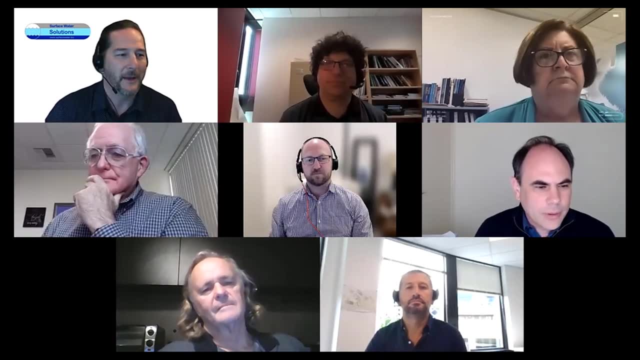 Now you're gonna see a lot of the figures behind this, But I just wanted to throw that out there. We'll hear from the presenters very quickly, But those attending from CSIRO have you had people ask similar questions to you in the past, So maybe we'll start with Bryson. Has that comment come up? 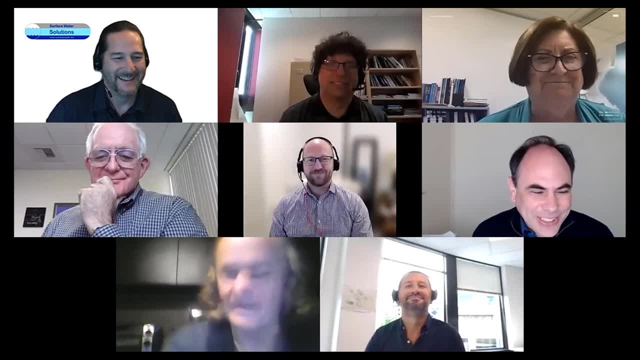 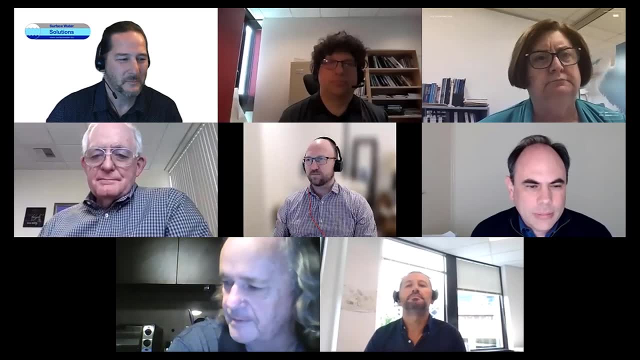 to you, Yes, over many decades, but I think in here I'm an engineer by background, not a climate scientist, But I think people tend to forget that the climate system is highly nonlinear and very complex. And when you speak of global warming and you start thinking: 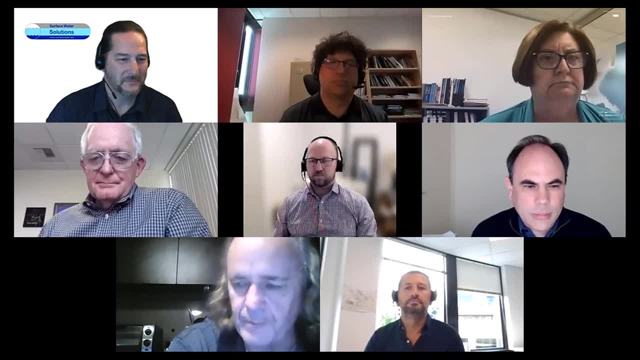 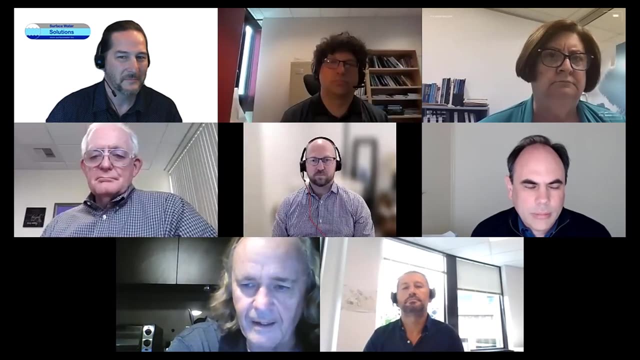 you know about melting ice sheets, particularly in places like Greenland, and the impact of that extra fresh water on what's called the Atlantic, overturning circulation, and what impact that has on the Gulf Stream. In fact, when you think about it, it means that weather might eventually. 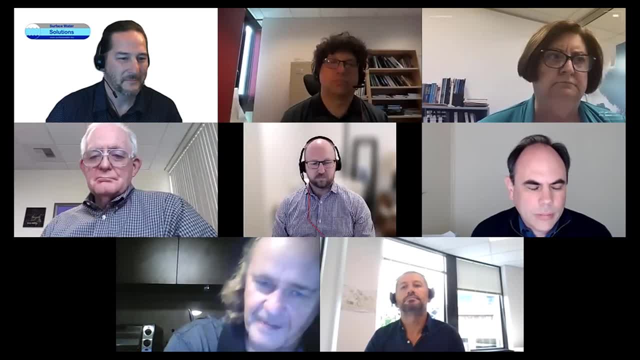 get colder because you know the slowing down, slowing down the circulation, overturning circulation, slows down the Gulf Stream, So you don't get that warm water coming from the Gulf Stream, The coast, anymore. Yeah, so you can actually get cold weather, but I better hand over to the 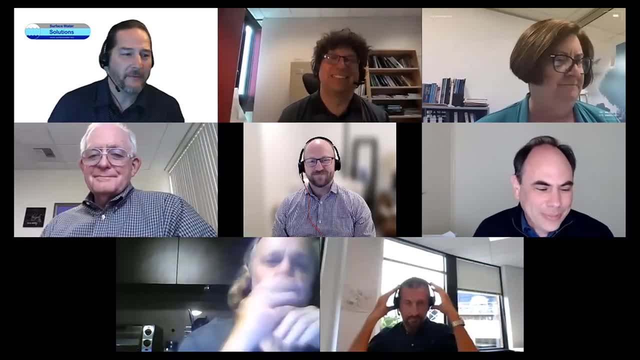 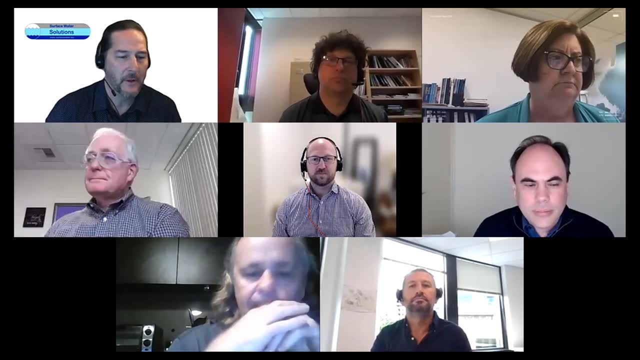 climate scientists before I go much further. Yeah, no, thanks, And that frames things up very well, Because those kinds of questions and discussions, we'll see the slides and the science behind that now And we'll see again also that question as to those, particularly in Australia as a case. 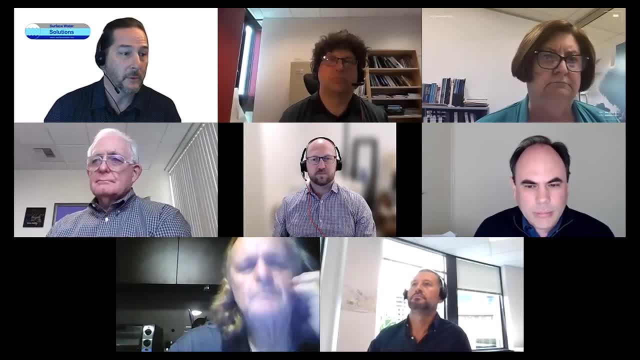 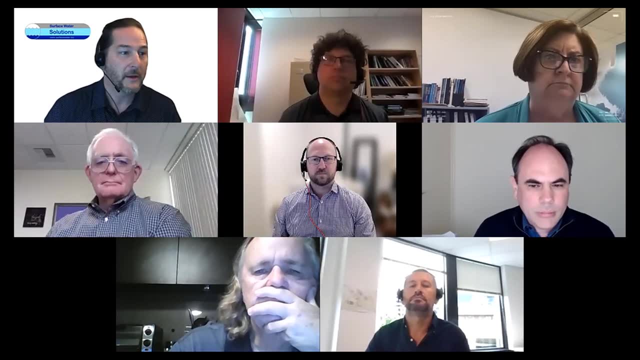 study which I think will be of interest to global attendees as well. today, You know, here's one specific area, one continent, where you'll see some examples Of how things globally can affect one part of the continent And those in Australia who are guided. 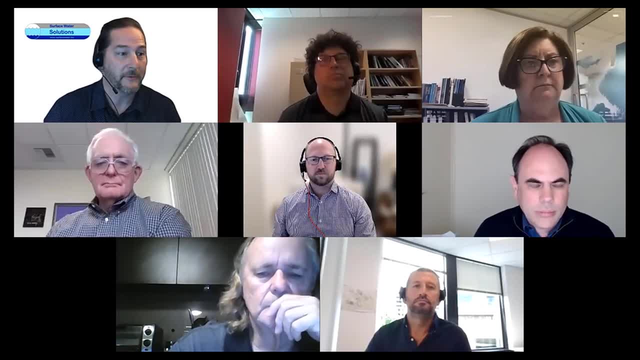 in the water field and the water sector by the Australian rainfall and runoff guidelines. have that question now. Okay, I look at the guidelines and we'll see some of these sources. What do I do with these? They're very general, but how can we specifically apply these to our 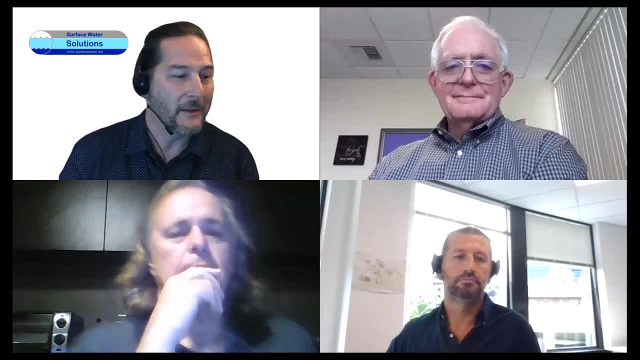 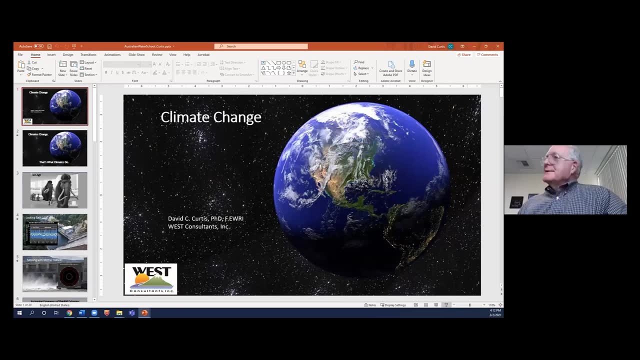 projects. So from the global focus first. David, let's have you come on. I'll turn straight over to you for your presentation, Looking forward to hearing from it. Thanks for coming on and thanks for your support. Okay, thanks everyone. It's great to be here. I'm going to talk for the 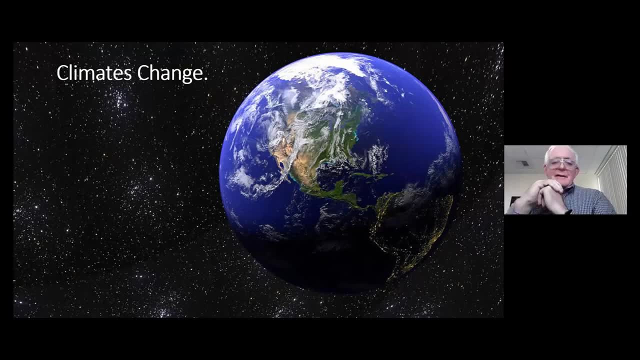 next few minutes about climate change. Now I've changed the slide a little bit and the title is no longer climate change, It's climates change. It's a simple declarative statement, Because that's what climates do: They change, And they've done so for a very, very long time, In fact. 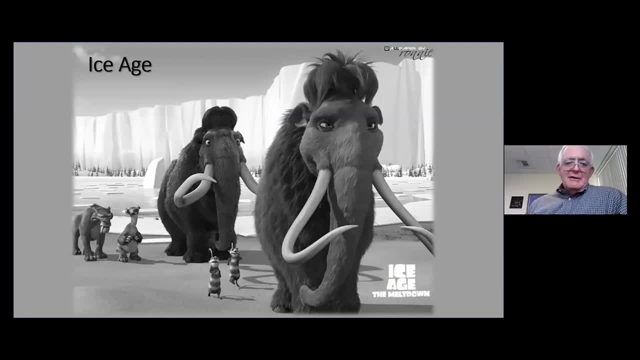 we know this because we have some extremely reliable documentary evidence that at one point in our Earth's history the Earth was covered by epic sheets of ice, sometimes kilometers thick. Today not so much. So obviously something happened between the ice ages and today in the climate system that doesn't support the generation of these ice sheets. So 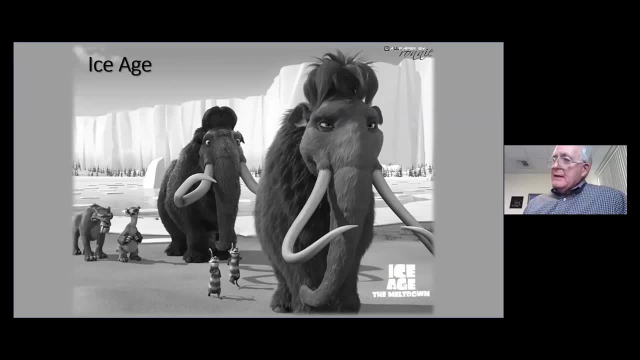 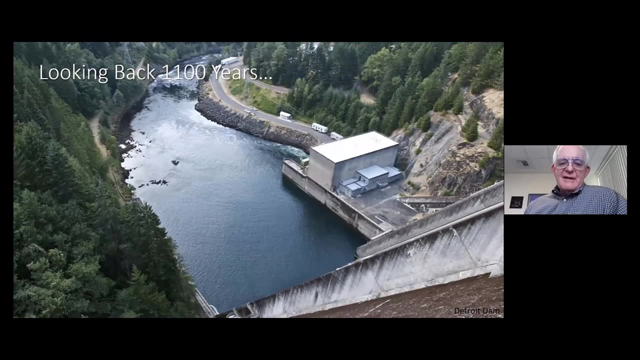 fundamentally, I think we all understand that climate changes, But as an engineer, that's a pretty long timescale for me to worry about. So let's shorten that timescale up a little bit and get the data back to the Earth, and let's start from the ice age. So if you look at the 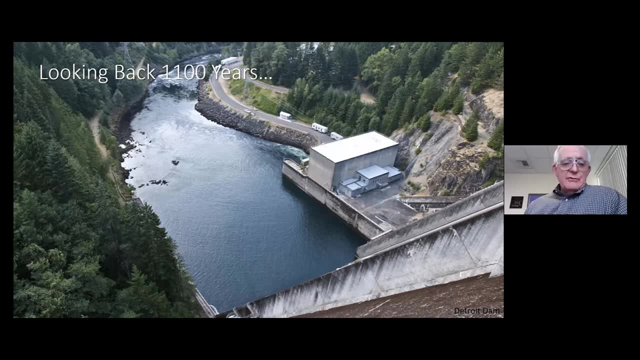 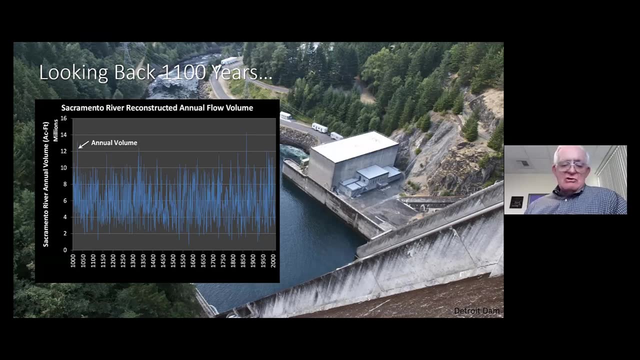 rock age. this is the age when the ice ages, the rock ages and the ice ages. they look back a thousand years or so. We can do that. we don't have any observational systems that go back a thousand years, but we do have some things that we can use as surrogates, like tree rings. So with 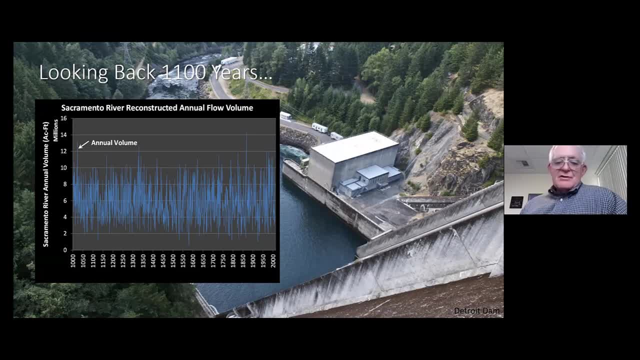 the judicious use of tree ring data we can actually reconstruct annual flow volumes in the river system, in this case the Sacramento River. Now this trace of annual volumes dating back a have here in California Kind of lurches back and forth like a drunken sailor on shore leave. 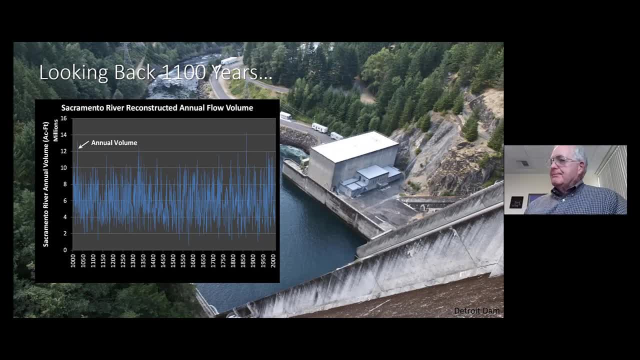 from extreme wet to extreme dry, with not a lot in between. But even a thousand years is a scale that's a little hard to kind of imagine and wrap our minds around. So let's kind of shorten it up and look at a trailing 30-year average of those annual volumes, And here you can see this 30-year. 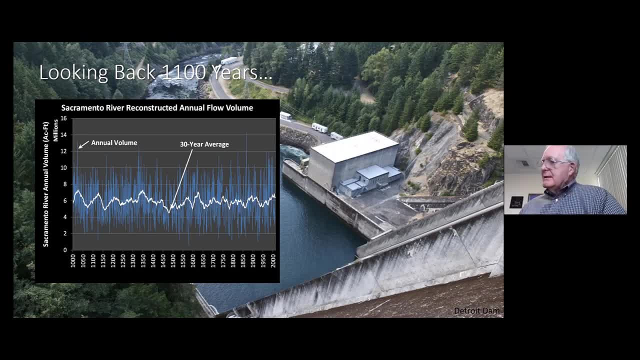 trailing average varies a lot And and it basically well, it indicates that, in the case of California, a plus or minus 50 percent change in rainfall coming into the state over, say, a 30,, 40,, 50 or 100 year period. That's a big change And the fact that we've seen this change and 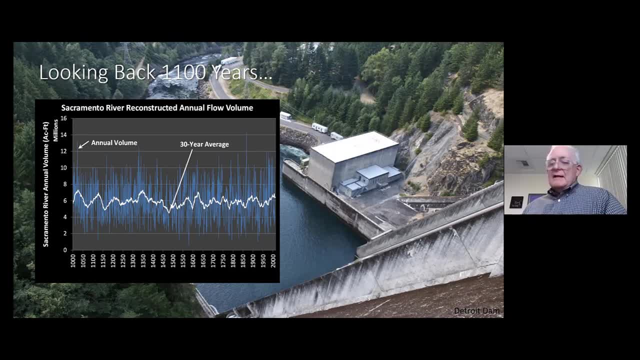 occurs over a thousand years indicates that that's that natural variable variability is a very strong signal in California and likely in other parts of the country as well, in other parts of the world. One of the surprising things is, if you look at the difference in time, 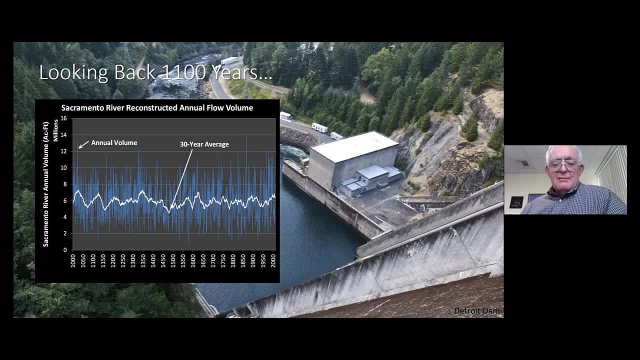 between some of these peaks and valleys you can change from an extreme wet period to an extreme dry period in a matter of a few decades. In fact, that transition time is well within the capital budgeting programs of a lot of water infrastructure planning horizons No one is actually planning for. 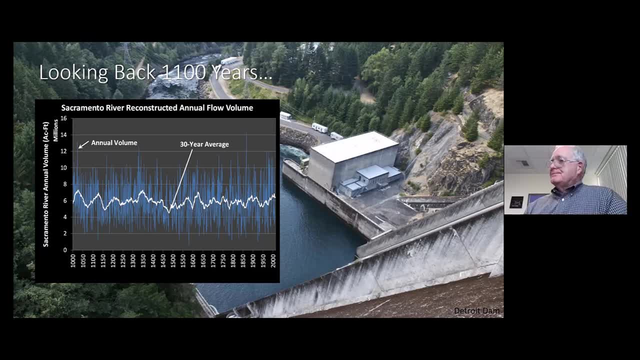 that today We're still planning for a static climate. Now in California we always consider ourselves to be perpetually dry, but if you look at the 2007 peak in our hydroclimate locally and go back a thousand years, that 2007 peak is in the top five wet periods for the last 1100 years. 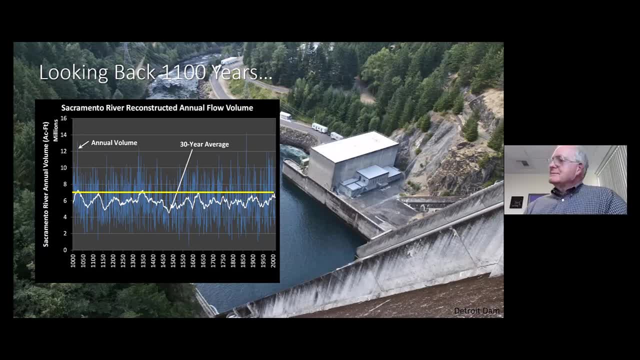 And when you're in the top of that peak, what direction can you go? Go down, And it looks like we're probably already a decade and a half into our next downturn of a multi-decadal period of dryness before the next wet period comes into play. So this is part of the natural way of things in a 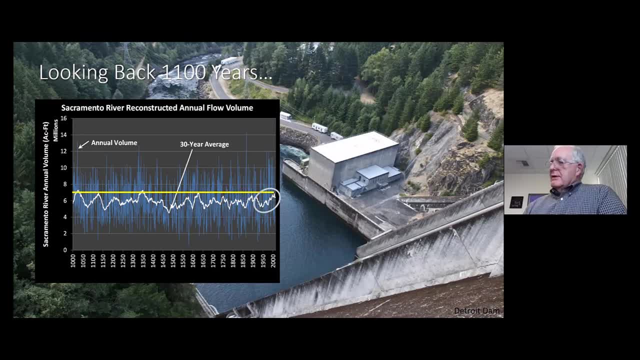 lot of areas in the world. One of the shortcomings that we have is our observational record. It covers a very, very long period of dryness. It covers a very, very long period of dryness. It covers a very, very short period of time And in this case you can see there's a strong upward. 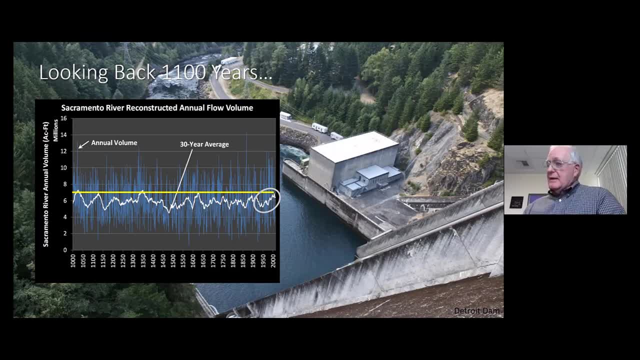 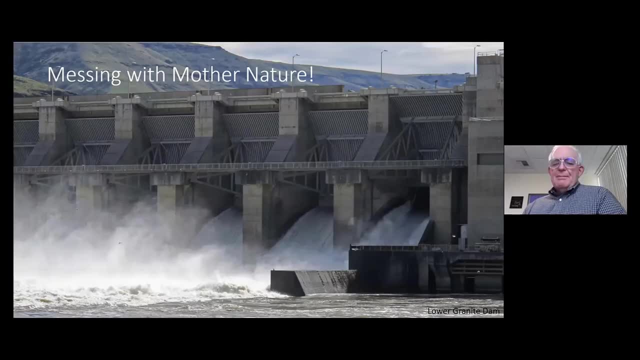 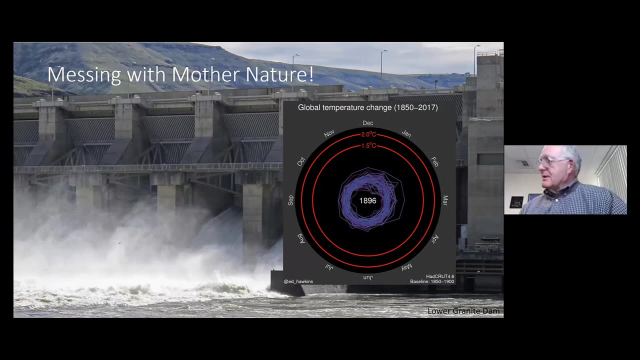 bias in the direction of water supply in California during that period, which actually severely colors some of our decisions. So on top of this natural signal of change, we've been messing with Mother Nature a little bit by tossing a whole lot of stuff up into the atmosphere that 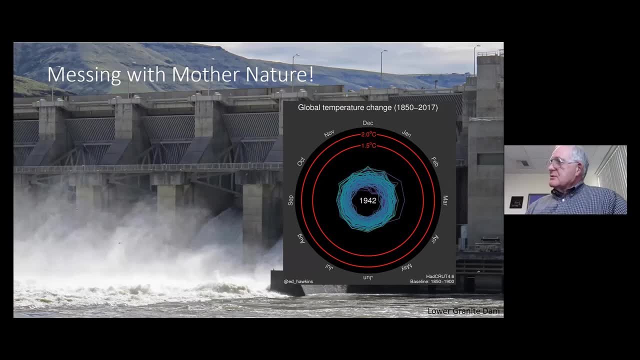 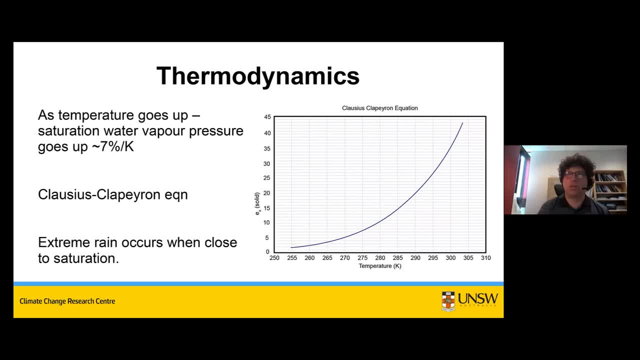 and it's a non-linear relationship. you can see it shown over here and it means that the amount of water at saturation in the atmosphere goes up by something like about seven percent per degree Celsius or per Kelvin as the temperature increases. When we have extreme rainfall, the atmosphere is. 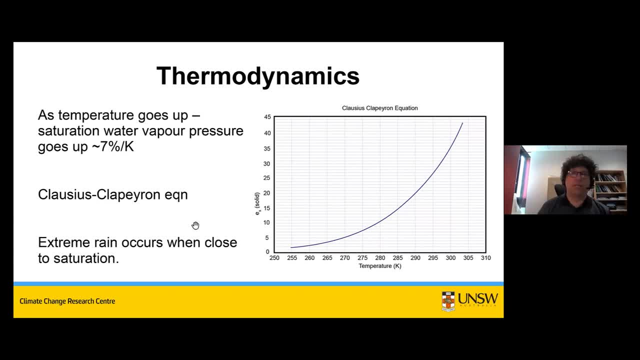 generally saturated or very close to saturated. so we can expect that the amount of moisture available for that rainfall is going up as something like seven percent per Kelvin, and that's a really fundamental thermodynamical property of the atmosphere. but of course, as we heat the atmosphere, that's not the only thing that changes. We also have to think about things like changes in. 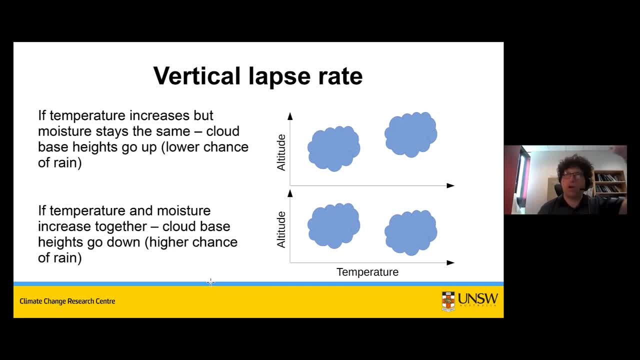 the vertical lapse rate of the atmosphere, so how the temperature is changing with height in the atmosphere, and that can change in complicated ways. but if we take sort of two examples here, if we have an increase in the temperature and we have an increase in the temperature and we have an 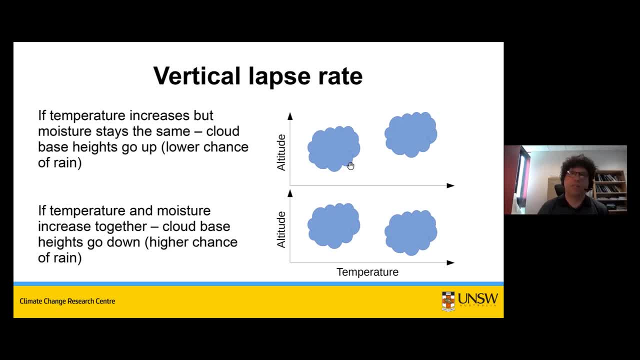 increase in the temperature but the moisture is staying the same in the atmosphere, then essentially what that does is it forces our cloud base heights to go up higher in the atmosphere, which essentially lowers our chance of rain. right it takes, it's a bit harder to make the clouds form. 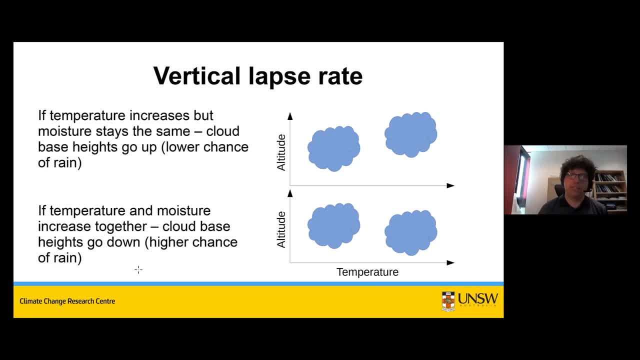 to start with. On the other hand, if both go up together, the temperature and the moisture both go up together, then that actually lowers our cloud bases, so which makes it a bit easier to form the clouds and gives us a bit of a higher chance of rain. Now, these two situations, this 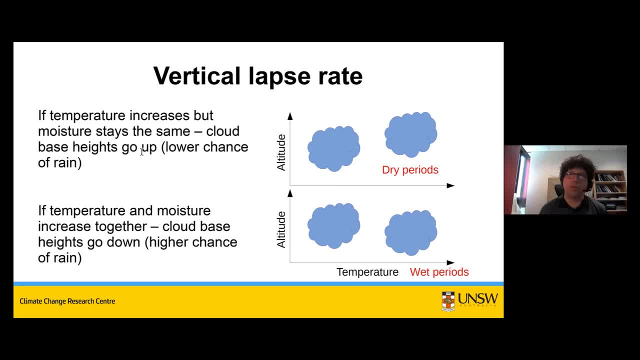 first one is kind of indicative of what we have in dry periods. right, we have low levels of moisture in the atmosphere. but if our temperatures go up with climate change and our moisture levels stay low, then in fact we get a situation like this top one, where our cloud bases go up in the atmosphere. 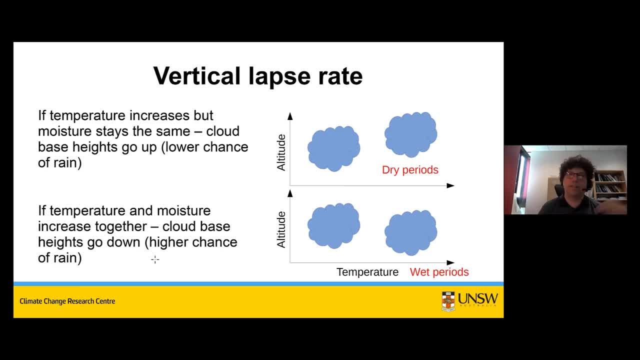 and it lowers our chance of rain. On the other hand, this lower example is what we'd have, what we might expect, during wet periods, when our atmosphere is close to saturation. anyway, what we end up having is cloud bases getting lower. This starts to change the temperature and the 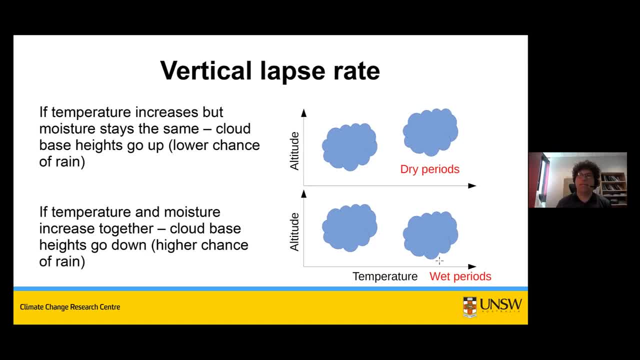 humidity of the atmosphere, and this is to help us understand why we have situations where we can get more rain in wet periods but then have longer dry periods in between, because both of these things happen when we warm our atmosphere because of the changes in height in the atmosphere. 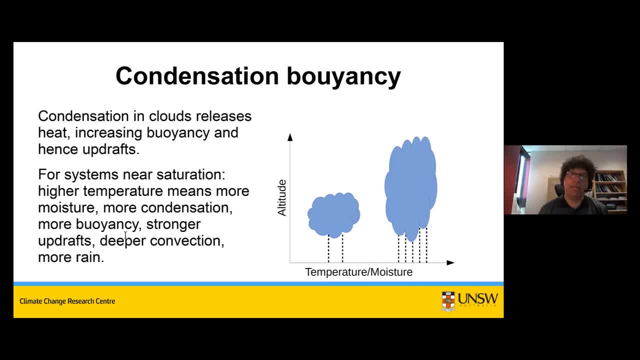 We also have changes in the amount of condensation buoyancy we get inside clouds. okay, so as we condense the water vapor in clouds, condensing to raindrops, we're releasing heat, which increases the buoyancy of the air in the in the cloud, and that will 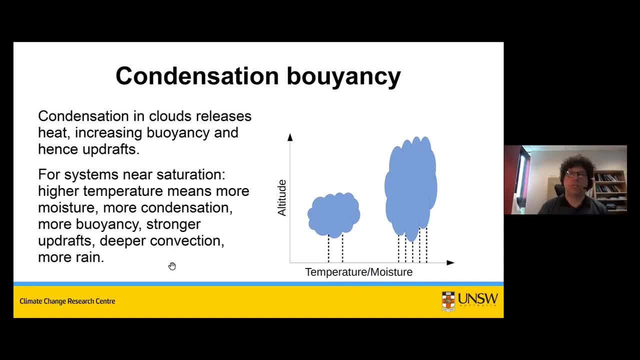 increase the updrafts inside the clouds. so for systems with a near saturation, higher temperature means we have more moisture because of the classes clapper on relationship. so that means once we form these clouds inside the clouds, we can condense more moisture out, give the cloud more buoyancy. 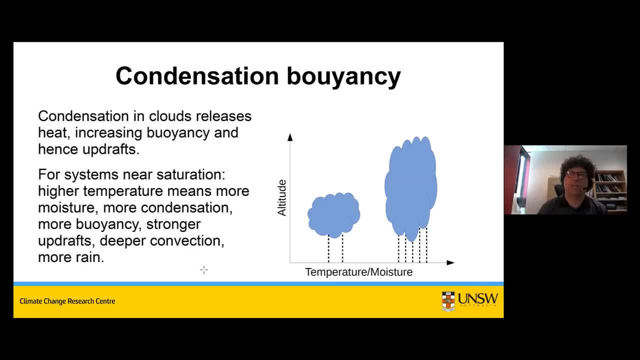 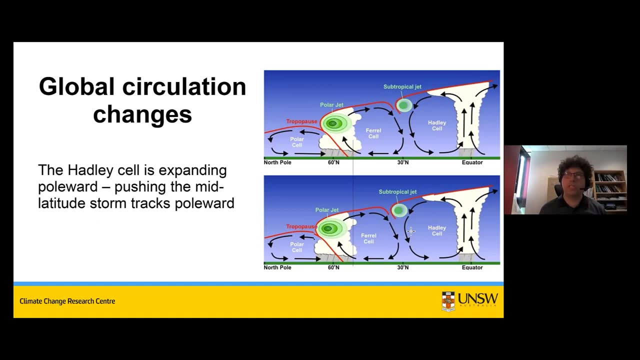 so we produce stronger updrafts, we get deeper convection, and that can give us more rain as well. okay, so this is another thing that happens in the atmosphere as we're warming it, and then we can also look at much larger scales in the atmosphere and look at the global circulation. that's 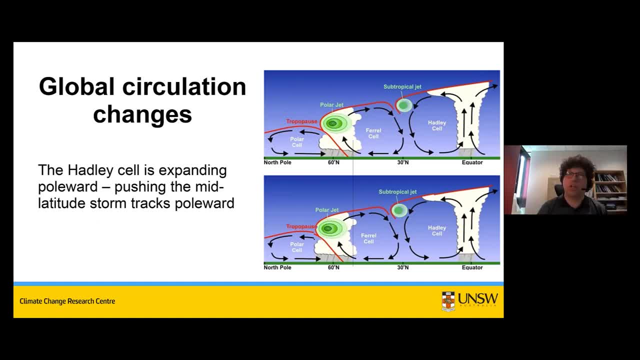 happening. here. we're looking at vertical cross sections of the global atmosphere from a pole to the equator, and we really in the atmosphere in general, the circulation is dominated by this tropical driven Hadley cell circulation, and then we have these what's often called the Farrar cell circulation next to that and then a polar cell near the pole, now one of 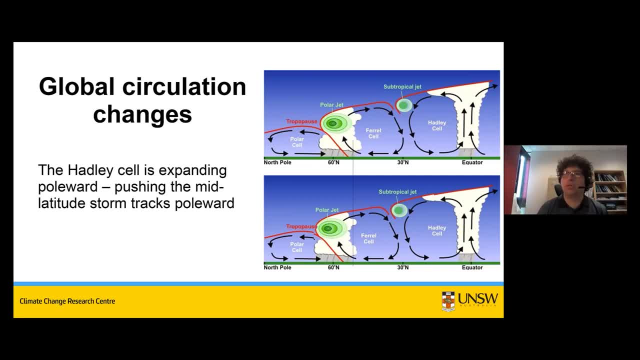 the things we see with climate change is the strengthening of this tropical circulation. So this Hadley cell, which often leads to an expansion poleward of the Hadley cell and that shifts these other cells poleward and moves this main storm tracks in the mid-latitudes towards the pole. 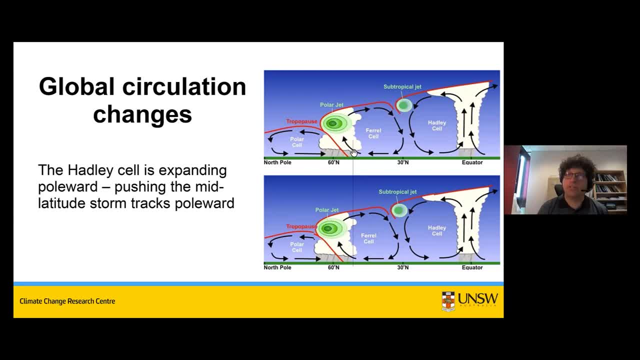 So, if you can just make out this line here, here we have a situation where this part of this area here is actually in the storm track at this time, But then, as we warm the atmosphere and increase the tropical circulation, we're no longer in the storm track at this location. 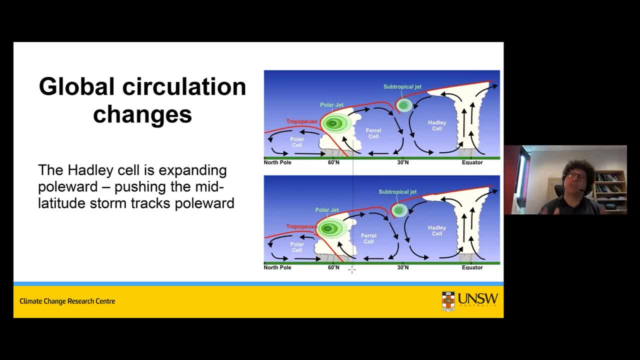 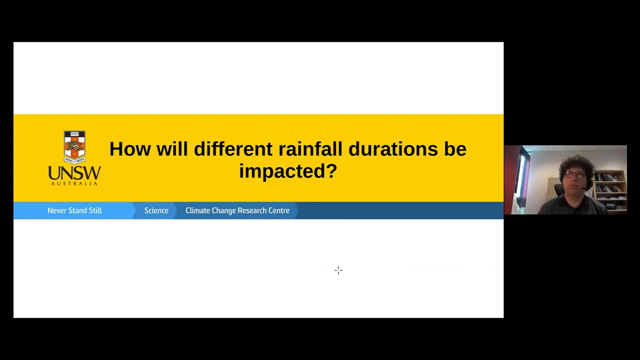 So these changes in global circulation can have really big impacts on particular locations in the globe, And it's often around the movement of the main mid-latitude storm tracks. That's a really brief look at a few of the main mechanisms that are going to be impacting our rainfall as we warm the atmosphere. 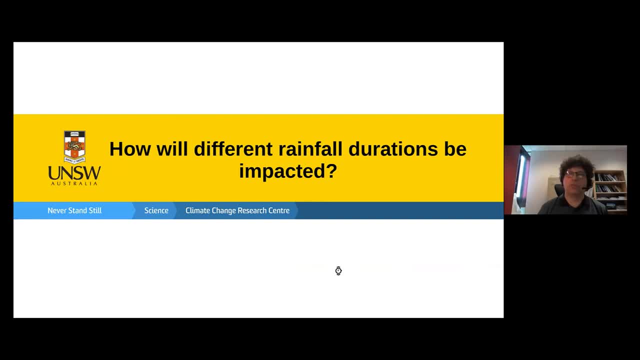 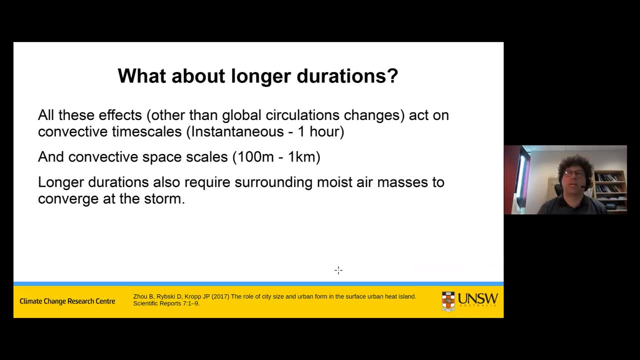 And now let's think about what that might mean for Different durations of rainfall. So most of the effects I talked about, other than the changes in global circulation, they really act on pretty short timescales, So convection timescales right. 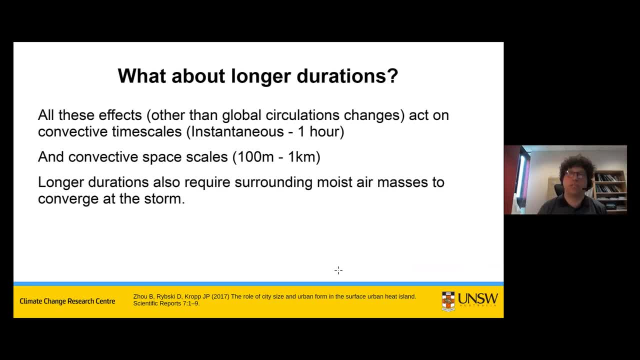 The timescales of actually creating these convective cells in the atmosphere, And you can think of this as broadly, anywhere from sort of instantaneous through to maybe an hour, right. So it's sort of these minutes timescales, And they also happen on fairly small space scales. 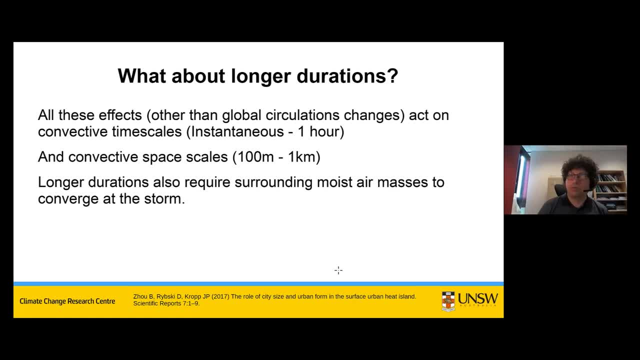 So these convective space scales may be on the order of hundreds of Metres to kilometre kind of scales. Okay, So if we want models that actually are going to capture these phenomena and how they're changing, we need to be looking at these kind of space and timescales. 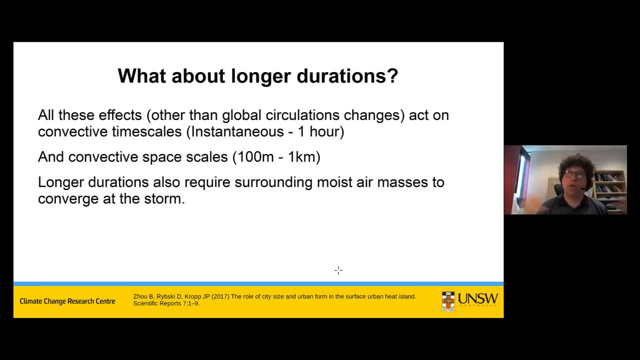 And, as David just mentioned earlier, if you're looking at global climate models, they're quite a long way from these space and timescales, So it's difficult for them to be able to capture all these kind of changes that I've mentioned now for longer duration. 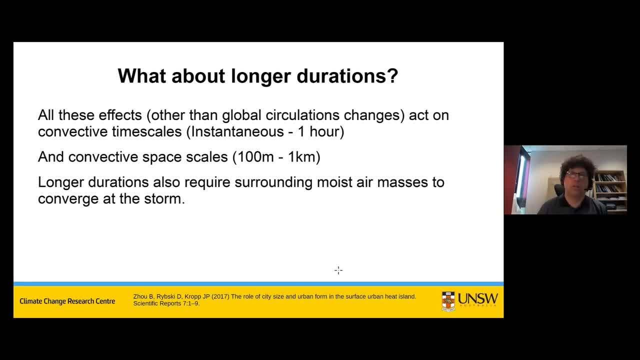 Precipitation, So we're thinking about longer than an hour or so. then we also have to think about the surrounding air masses for the region and whether they're moist or dry. So if we want to have longer duration rainfall extremes, those surrounding air masses need to be moist so that as they converge into the storm, they're bringing lots of moisture with them, which can then be rained out within these convective clouds. 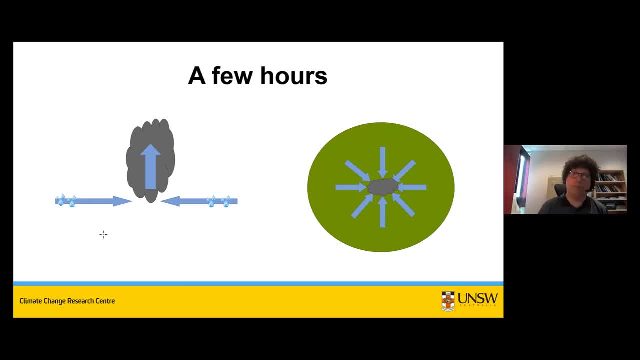 Okay, So so this is the typical sort of idealised picture That we might have. So we were forming a cloud, We've got buoyant air in here, We've got updrafts driving this up. This low level air has to be replaced by air from around. 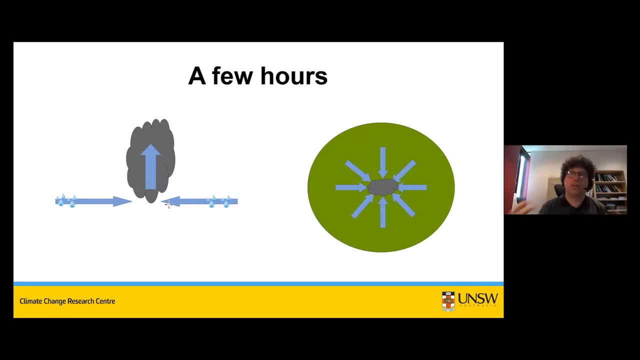 And in order for this to give us a heavy rainfall event, then this air masses that are converging have to be moist as well, bringing lots of moisture with them. And here we've just got an idealised picture. If we're looking down from above, of course, those air masses can be converging from any direction, all around the storm. 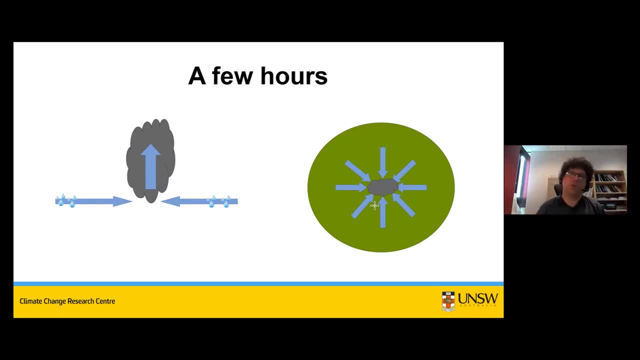 So for a few hours you need this kind of thing. So we've got all these things that might change, or many of them enhance, convection where the convection is occurring, But for a few hours. we also need the air a bit further away to also be moist so that when it converges in it's adding that extra moisture to it as well. So we start thinking about longer timescales, out to 12 hours. Then, of course, there's a much bigger catchment area, if you like, for the storm, So a bigger part of it, So a bigger part of the atmosphere, has to be moist, because that's the area that the storm is going to have air masses converging into the storm from. 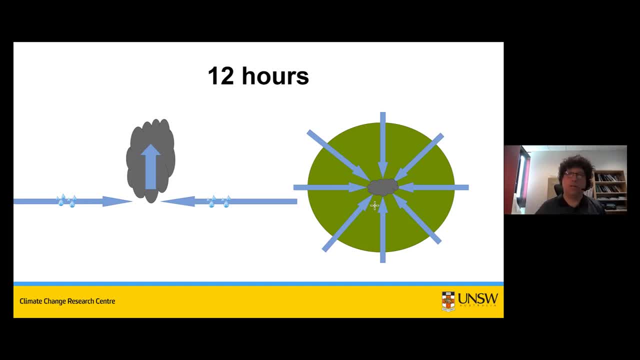 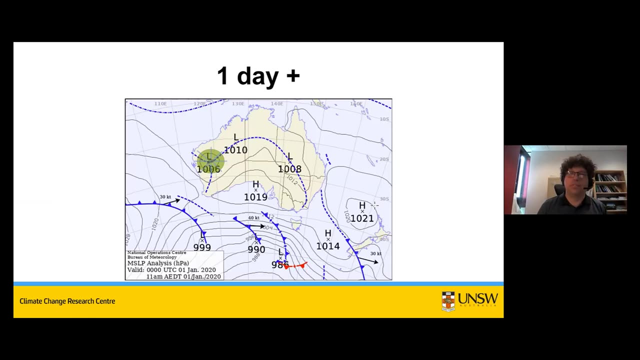 So if we want to have heavy precipitation over a longer period, we need to have a bigger area of the atmosphere being close to saturation, with lots of moisture in it. If we then think about even longer durations than that, then we need to start thinking about lots of other larger scales. 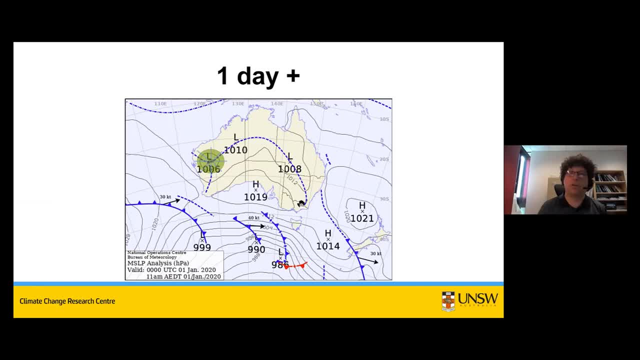 So it's the same thing with the pale aspects of the atmosphere, all this synoptics that are going on, the movement of the high and low pressures, the warm and cold front movement. So it's more than just having moist air around the area we're looking at. 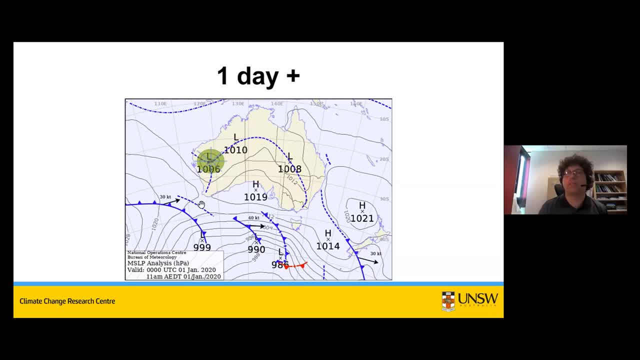 It's also how it interacts with all these other synoptic factors going on in the large areas as well. So when we think about these longer duration extremes, we have to be thinking on these sort of synoptic and larger scale space scales as well. 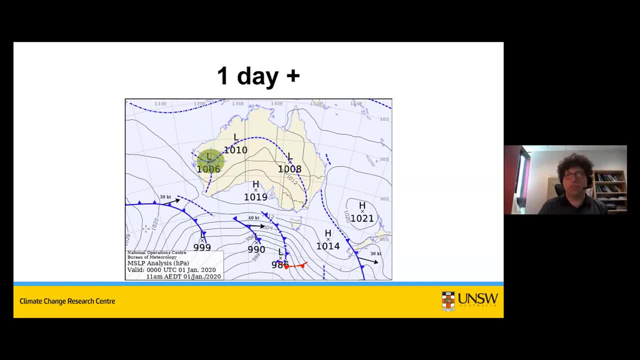 And it turns out- it's not always like that, But in many cases on average, when we're looking at these larger things and we have a lot of these phenomena, synoptic scale phenomena- interacting and to produce these daily and longer extremes, a lot of the effects kind of average out. 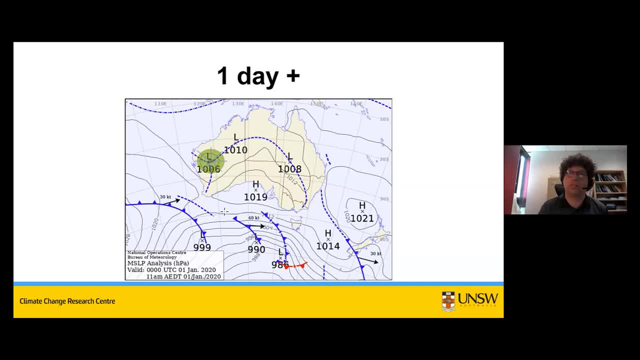 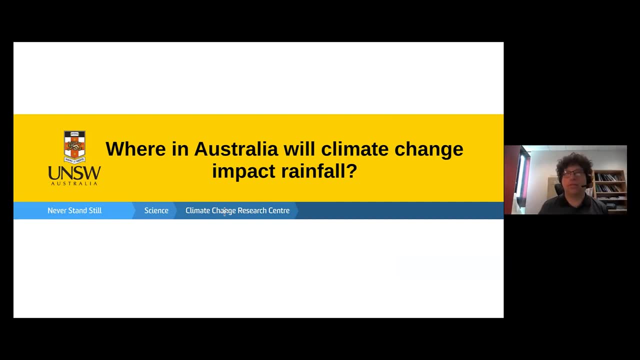 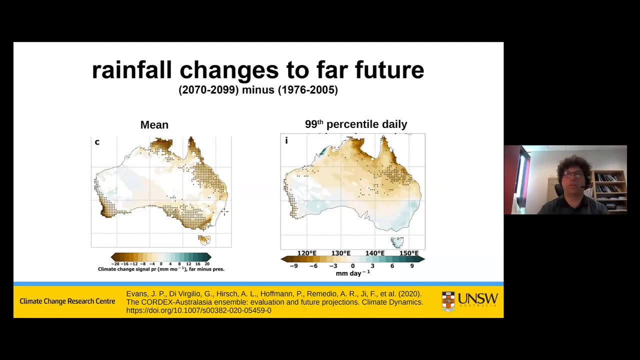 And what we actually observe is often quite close to the Clausius-Clapeyron increase with temperature. Okay, so, with all those things in mind, I'm going to have a quick look at what some of the climate changes have been projected for Australia, and we'll also have a look at some of these effects elsewhere as well. 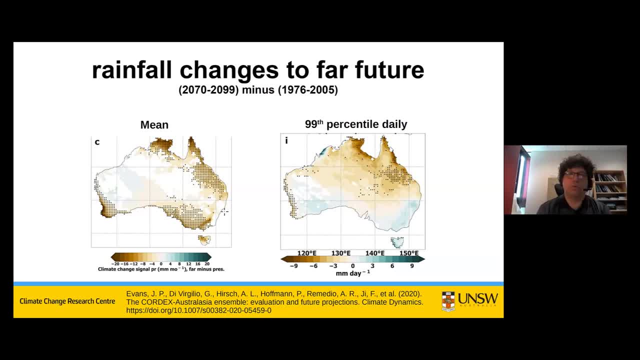 So here I'm just comparing what's projected for change in the mean rainfall. This is out towards the end of the 21st century and compare that to the 99th percentile daily, which in many places is about the heaviest rain day per year in many places. 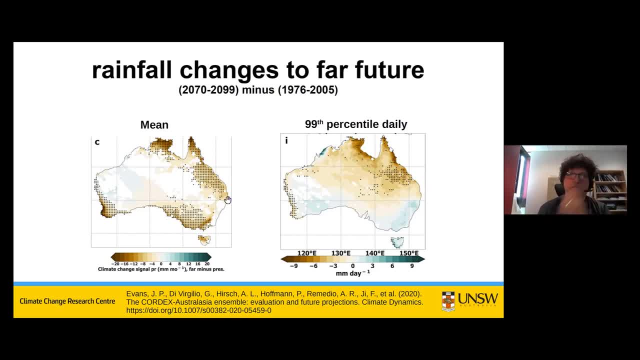 It's not exactly, But what I really want you to show you with this is that, well, first, in the mean, Australia is largely projected to become drier And these places where you see stippling are the places where the model ensemble agrees that there's significant drying occurring in those locations of Australia. 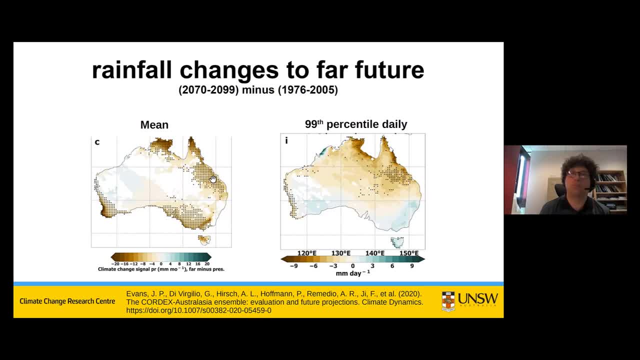 So that's the southwest, the southeast and the northeast and some north as well. When we compare what's happening in the mean to what's projected to happen in the extreme, here you see some real differences. So In the northeast and north the mean and the extreme rainfall are both decreasing. they're going together. but in the south, southern part of Australia we see opposite changes. where the mean is projected to decrease, we're getting drier, but these extreme rainfall events are projected to increase in magnitude, to become heavier. 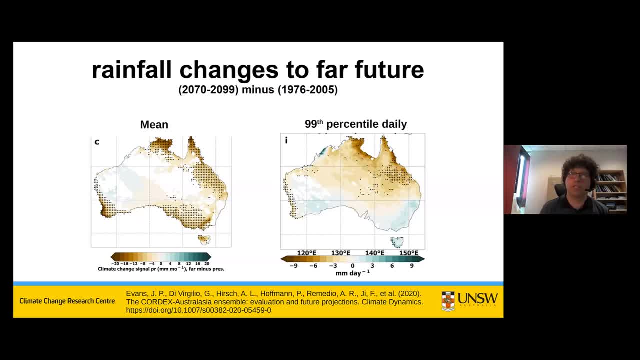 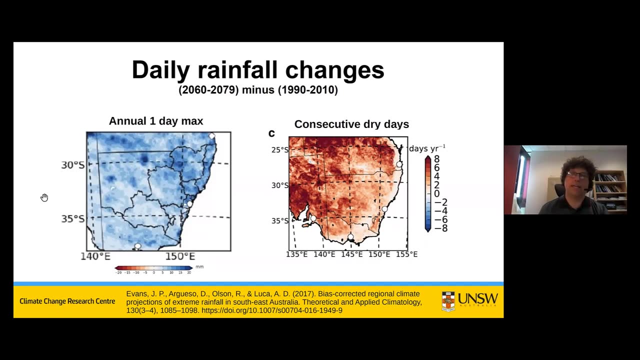 And this is something that you see in many places around the world in the projections- actually not everywhere, but in many places you have Declining mean rainfall or no change in mean rainfall, but an increase in these extremes. and Here I'm just going to zoom in on the southeast Australia again. here on the left I'm just showing what's happening to the annual one day maximum rainfall magnitude And you can see, essentially you're seeing increases everywhere. 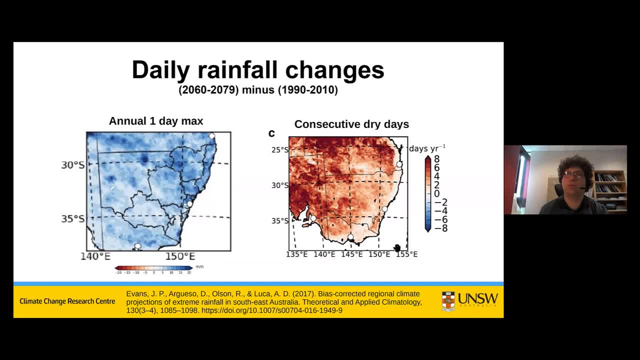 And here on the right we're looking at how the number of consecutive dry days is changing at the same time. So you can see Significant increases in the length of these dry periods at the same time as we're seeing Increases in the magnitude of these heavy rainfall events when they occur. 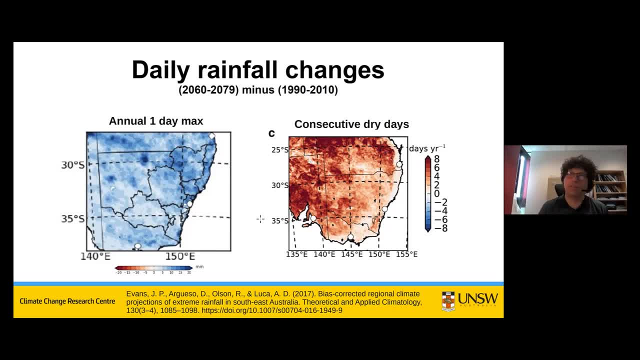 And this is something that we should probably expect. one of the things that I showed earlier, of course, is we expect different changes in The cloud base Heights under dry conditions versus wet conditions as we warm the climate, Which leads to these opposite Changes occurring. 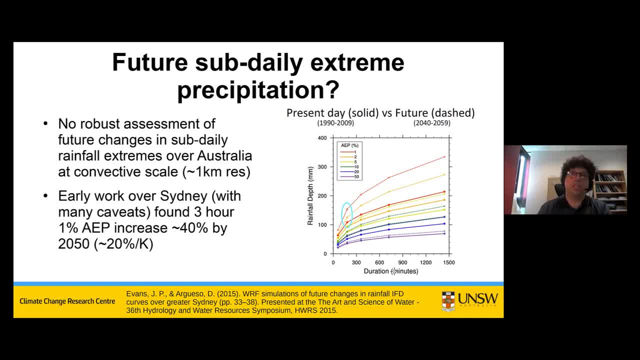 If we think about future sub-daily extreme precipitation. I want to start by saying that at the moment we don't really have a robust assessment of changes in sub-daily rainfall extremes over Australia at convective scale. so I'm talking about about kilometre resolution type scales. We did do some 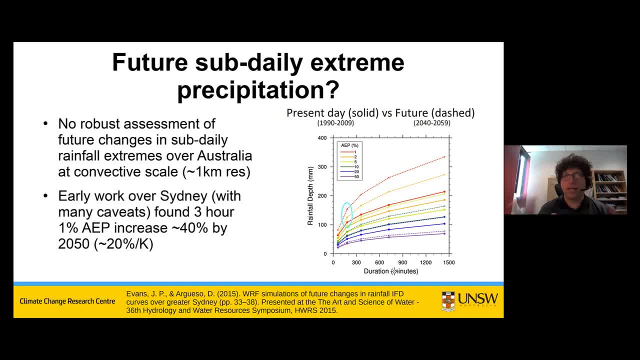 work looking at this over Greater Sydney and there's lots of caveats around this. but what we did find in this early work is an example here. for the three hour one percent AEP we see an increase of about 40 percent out to 2050. So in that period we see an increase of 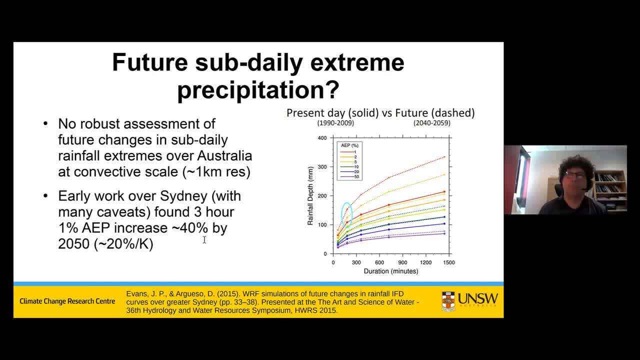 about two degrees. so that was an increase of about 20 percent per kelvin, which is a lot higher than the Clausius-Clapeyron relationship, which would suggest about seven percent per kelvin increase. And it's a lot higher because we have also, as well as Clausius-Clapeyron, we have all 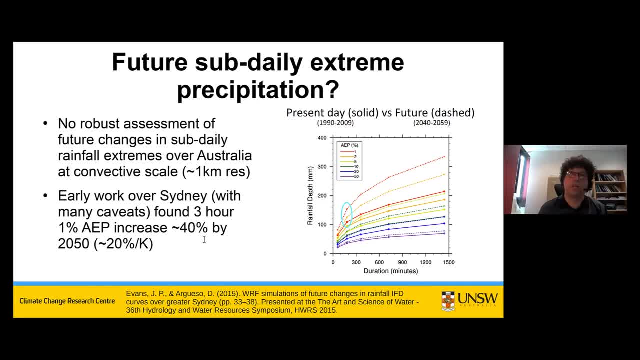 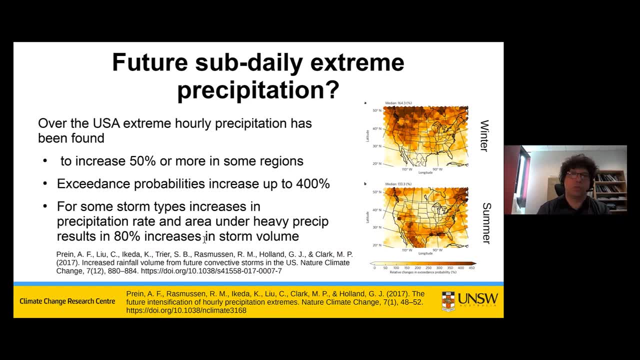 these other changes in the atmosphere that also occur particularly at these shorter time scales. Thank you. So these kind of studies have been done more elsewhere in the world. There's a bunch that have looked at particularly over Europe and North America. So here's some examples that have looked. 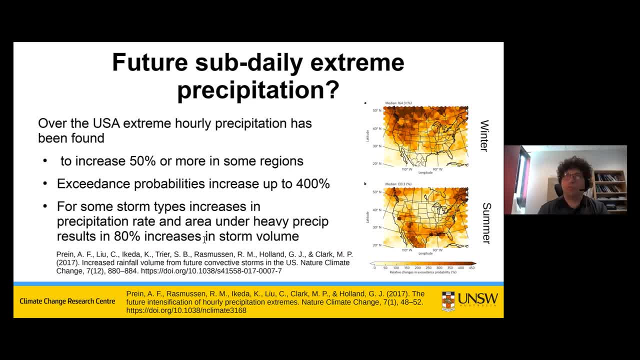 over the USA using convective space and time scales. Here we're focusing just on hourly precipitation results, and what they found in these studies was that the hourly extreme rainfall was increasing. annual extreme rainfall was increasing 50 percent or more in some regions across the USA. 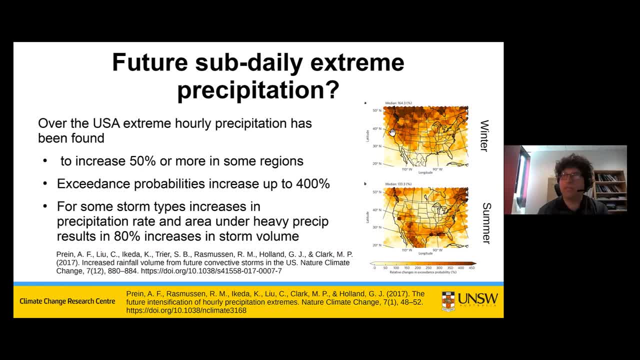 exceedance probabilities were showing relative increases up to 400 percent and that's what we're showing in this figure here from their paper. You know you can see it's different locations in winter and summer, but in many locations these relative increases are very high, So this can be. 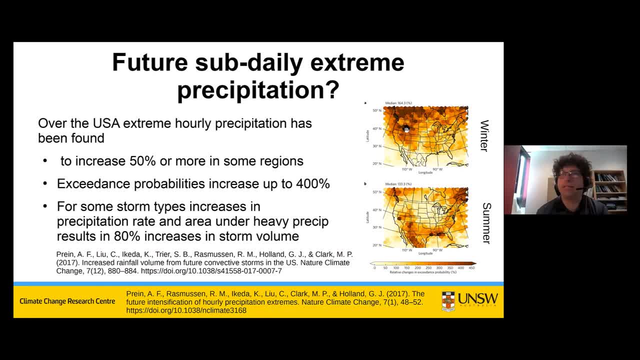 thought of as a sort of one in 100 year event, becoming like a one in 25 year event, so occurring much more frequently. And another interesting thing they did in this study is that they found, for many storm types, not only did they find that they found that they found that, they found that they 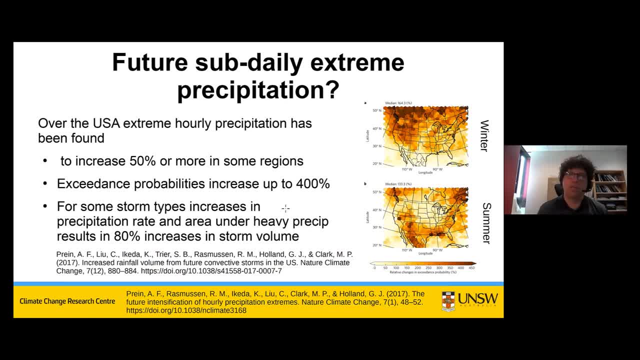 only are you seeing increases in the precipitation rate, but you're also seeing increases in the area under which is receiving the heavy precipitation, And when you put those things together, you're seeing increases in the storm volume produced by these storms on the order of 80 percent. 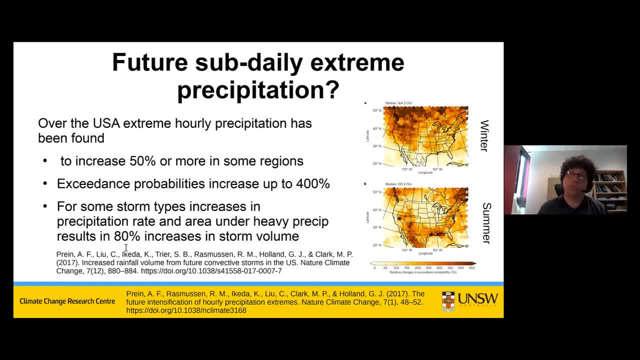 Okay, so that's, that's the volume of water that would go towards producing floods. Okay, so it's quite a bit more than just looking at the change in precipitation rate at one point in the storm. The combination of that with the changing storm area becomes really. 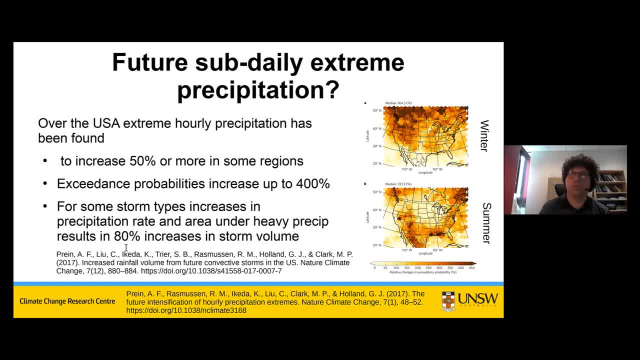 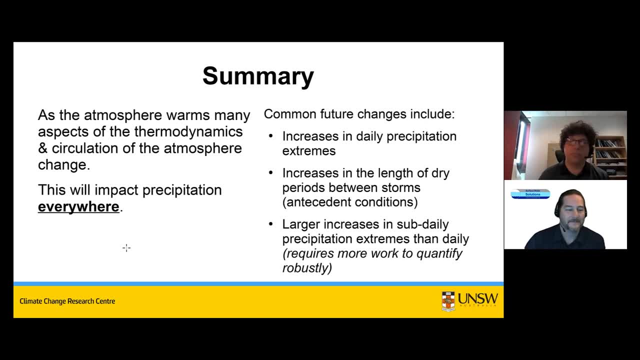 important when we're thinking about the actual volume produced by these storms. Okay, so I'll give a quick summary Then. basically, as the atmosphere warms, there's many atmosphere aspects of the thermodynamics and circulation of the atmosphere that have to change, And this means 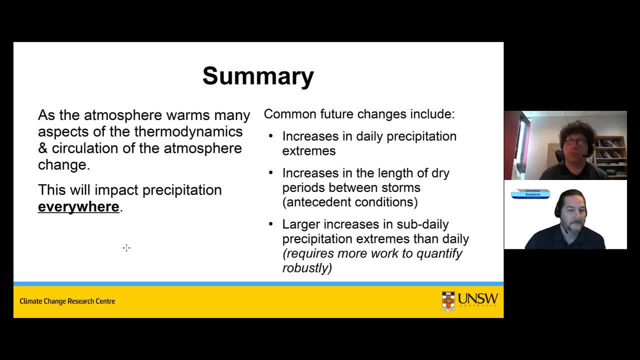 that climate change will impact precipitation everywhere. There's nowhere that won't be impacted, And some really common changes that we see are: we see increases in daily precipitation extremes, So that's really important. You know it's not a really bad thing to do it, but it's a 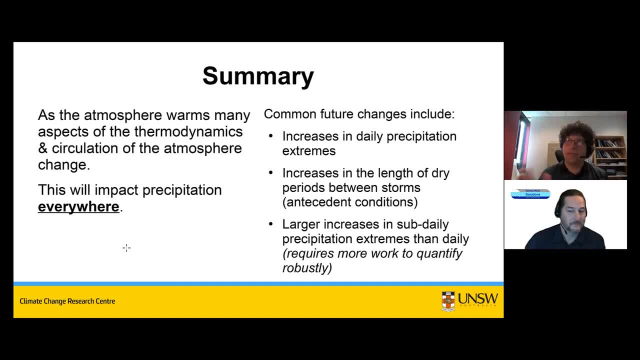 I think David also showed that those increases are often around the Clausius-Clapeyron factor, about 7% per degree. We also see increases in length of dry periods between storms, And this, of course, would be very important for thinking about antecedent conditions. 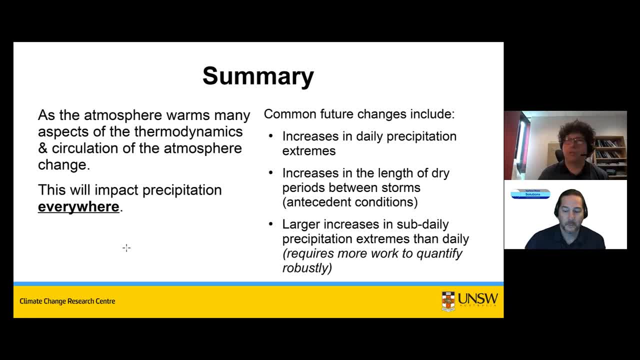 for when we do get the heavy rainfall And we often see larger increases in subdaily precipitation extremes than in daily precipitation extremes. And just with the caveat that this is an ongoing research question and there's a lot more work to be done to be able to have. 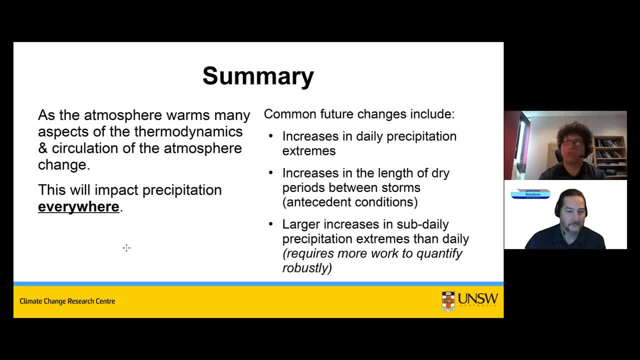 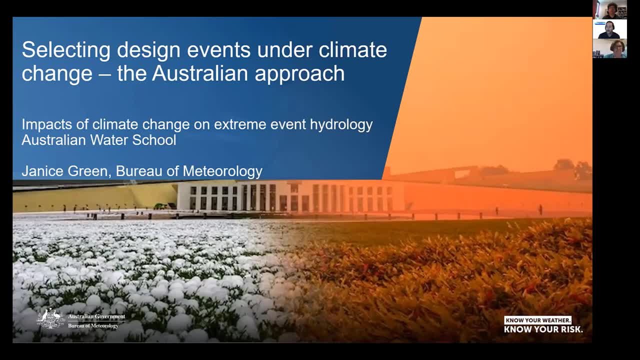 something really robust around the changes of these short-duration extremes, Excellent. Well, thanks for that, Jason. Just wanted to hit one quick comment here from Franciscus saying that shouldn't we be leaving these decisions on climate change to the hydrological experts, like we see here on today? 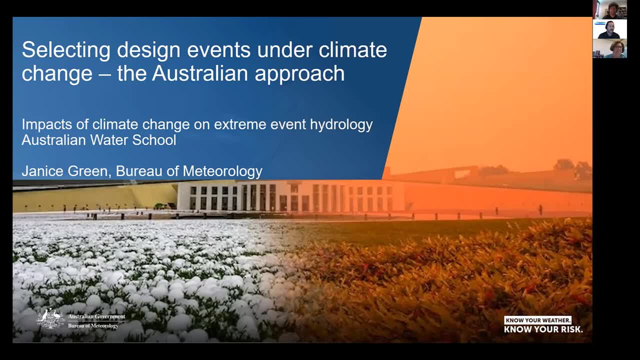 and not to engineers and modelers. And yes, absolutely. This is why we've got Janice on here today helping us with the guidance. I don't want to make these decisions. I don't, you know. this is something. 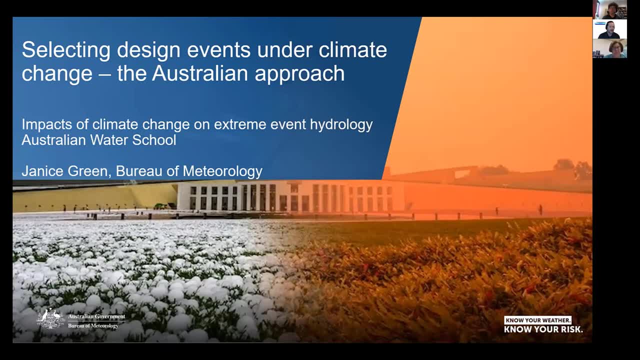 that I want others who have studied this for their whole careers to make those decisions. I want to turn to the guidelines and say, all right, tell me what to do as an engineer. You know I don't want to pick that number. 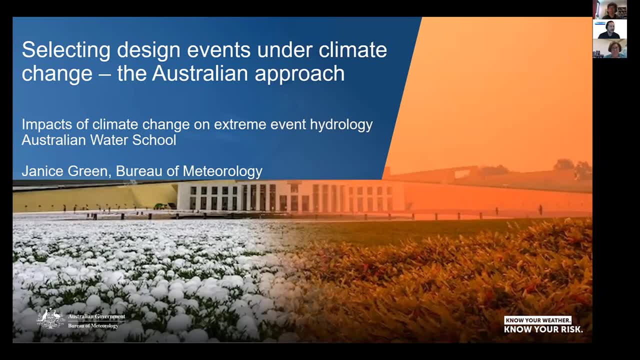 I want somebody else to tell me what that number should be. Let's look into the guidance and see what we've got here for Australia specifically and again, keep those questions coming in the background and we'll open it up to a live Q&A session after Janice's presentation. 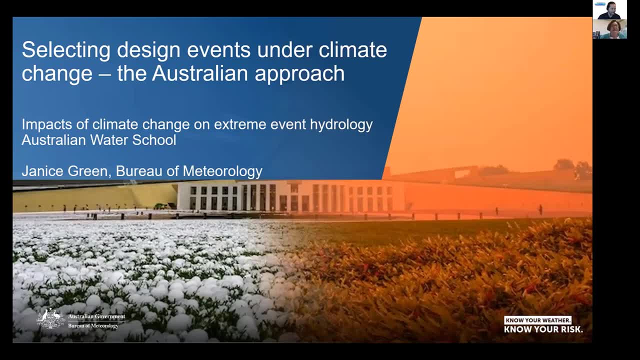 So over to you, Janice, if I can see your screen just fine. And yes, what I want to do is just talk about that. these decisions have already been made and are included in contained in Australian Rainfall and Runoff. 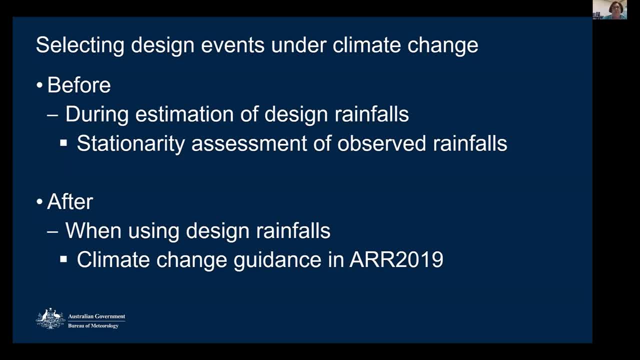 What I want to do first is just talk about the answers to a question that we receive most frequently in the IFD mailbox at the BOM, and that is: do the new design rainforests incorporate climate change? And I want to answer that in terms of looking at before. 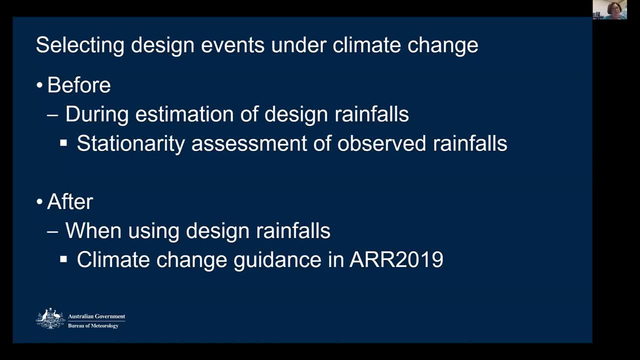 so, before we started estimating the design rainforests, the design rainforests, the design rainforests, the stationarity assessment of observed rainforests we undertook. and then after, which gets more to the question of how does a hydrologist 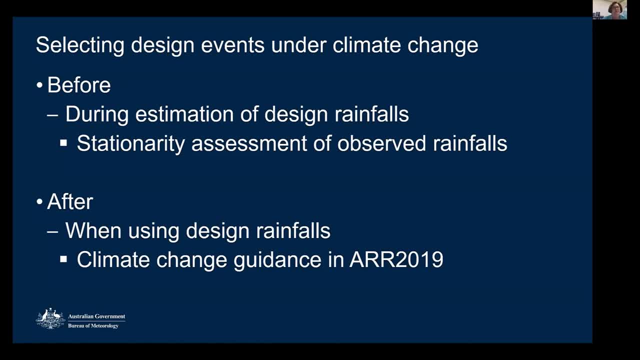 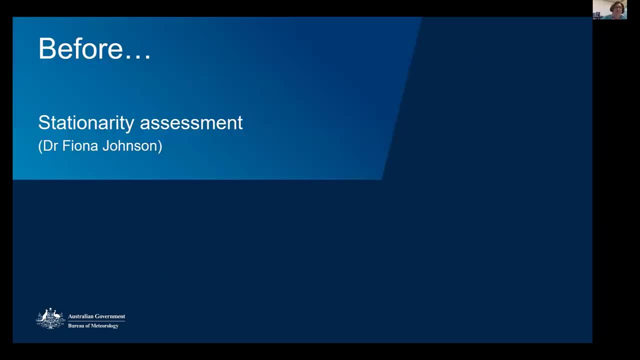 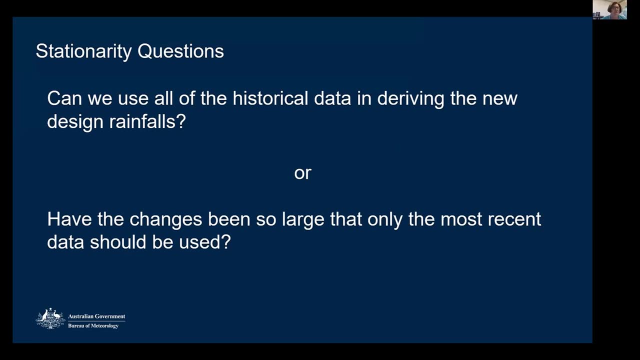 how does an engineer include climate change or the possible impacts of climate change in their design rainforests? And I just want to acknowledge that the work that I'm presenting was undertaken by Dr Fiona Johnson, who's currently at UNSW, worked for the BOM on this work. 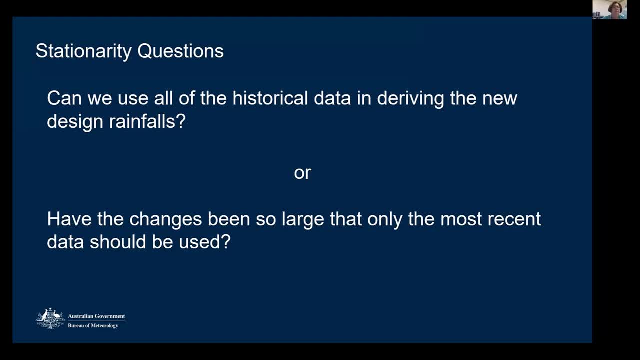 And what we wanted to answer right at the beginning of the design rainforest project was: can we use all of the historic data in deriving the new design rainforests, Or have there been changes so large that only the most recent data should be used? 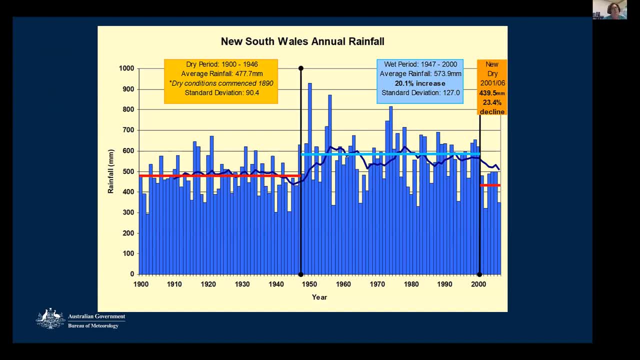 And that's exemplified by this graph which shows- and it's a little bit dated, but it's what we were looking at back in 2008,- is we've had some very obvious dry periods, very obvious wet periods and, as we're all aware, 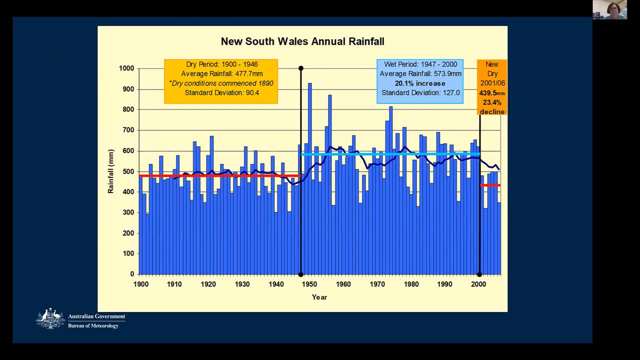 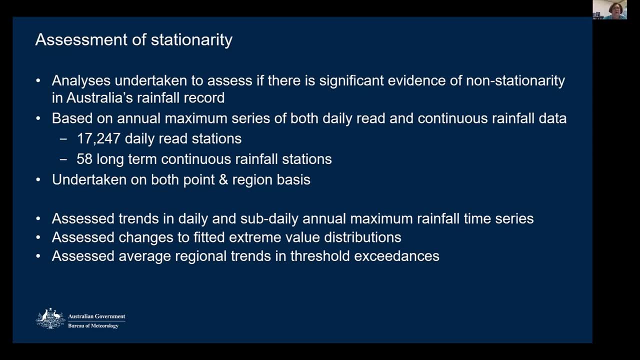 most recently we've had some very we've moved back into very dry periods. So, in terms of how we looked at this, we did a range of studies, some which we developed ourselves and some which also adopted the approaches that NOAA adopted in the US. 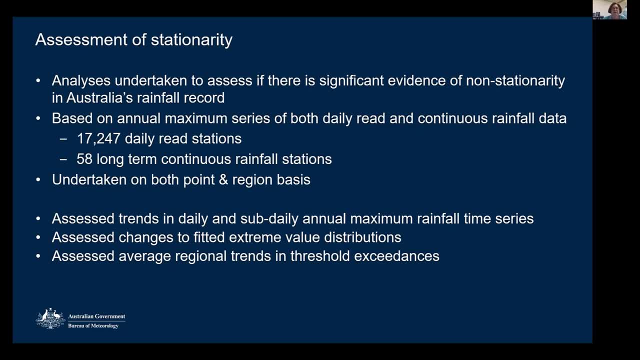 for when they undertook a similar study And we used the annual maximum for just over 17,000 daily red stations. because of the paucity of continuous we used, we used 58, but they were the long-term continuous rainfall stations and we undertook the analysis both. 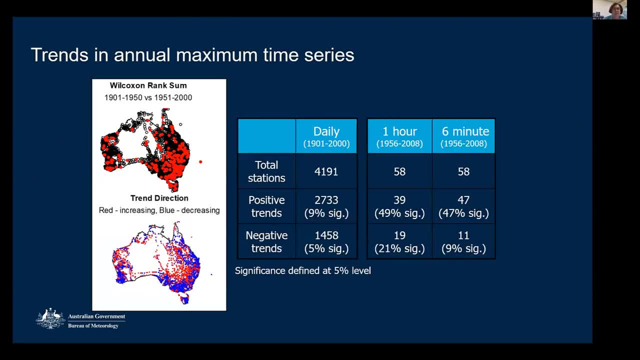 on a point and a region basis. We looked at trends in annual maximum time series across Australia and you can see there that we sort of saw. what we saw was there were positive trends and there were negative trends, but they were basically both for an hour and for six minutes. 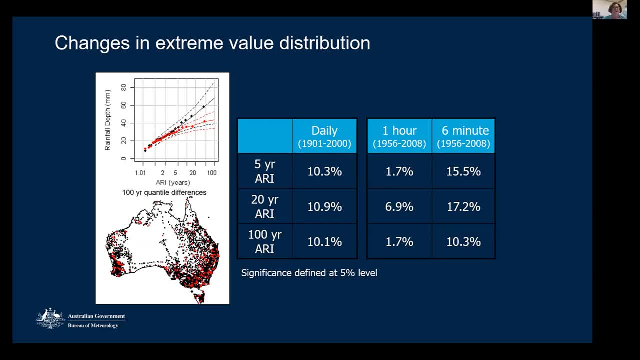 They were about the same. When we looked at, you know, changes to the fitted extreme value distribution, again, we saw whether we were looking at daily data, one-hour, six-minute data, five-year ARI, 100-year ARI. 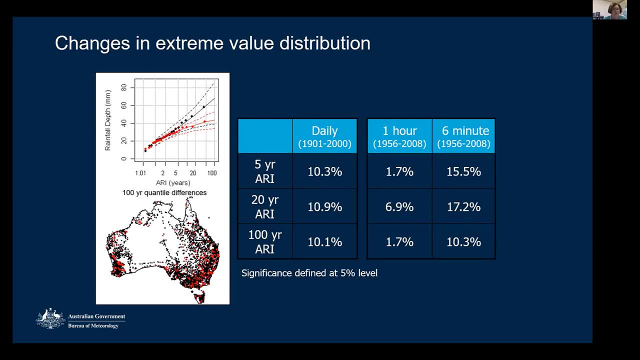 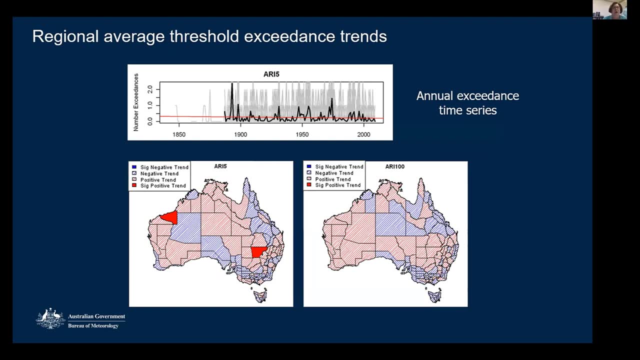 again, we were getting very similar differences in terms of the changes, Looking, as I said, at the regional values rather than just at site. so, pooling data again, what we saw was that we had some significant trends, we had some negative trends. 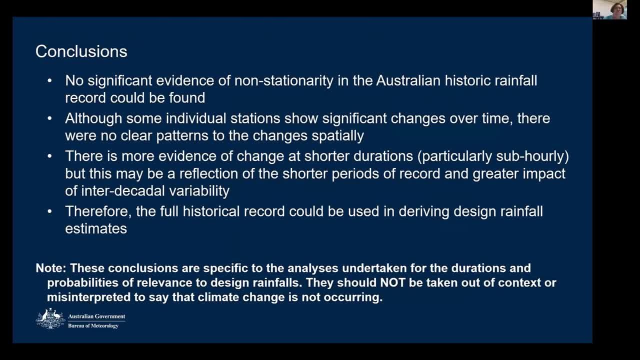 and some positive trends. so, in conclusion, what we found was there was no significant evidence of non-stationarity in the Australian historic record, although some individual stations show significant changes over time When you look at that spatially and you look at it at the regional basis. 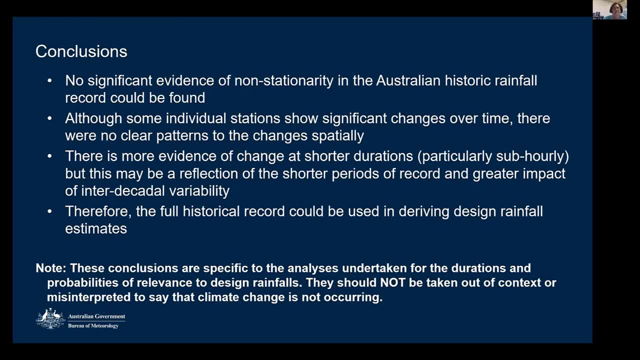 there was no clear patterns. There's slightly more evidence of change at shorter durations, particularly sub-alley, but this may just be a reflection of the shorter periods of record for the sub-daily rainfall data, which have a greater impact, a more greatly impacted on inter-decadal variability. 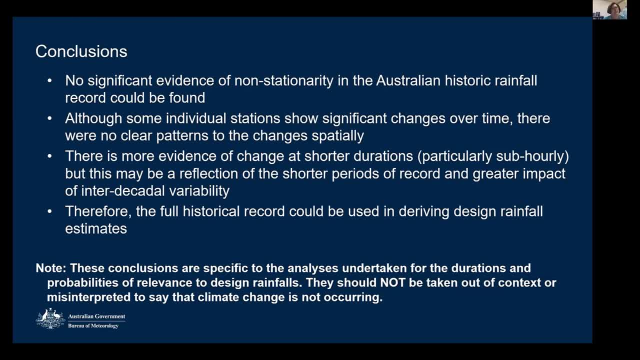 So the decision we were confident in was that we could use the full historical record when deriving design rainfall estimates And, interestingly enough, this is the same conclusions that the US came to when they undertook similar analyses. I just want to make a point here that what we found for this particular study 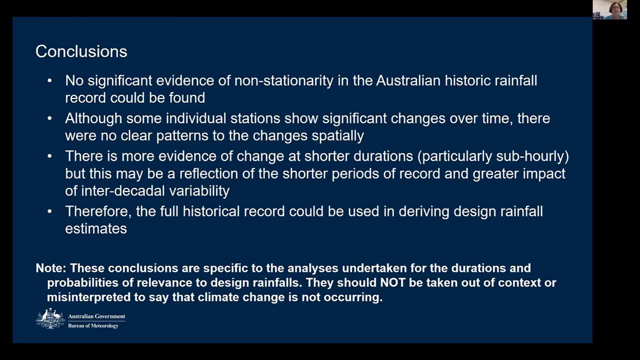 was for the very specific purpose for which the rainfall data were going to be used and for the durations and probabilities of relevance to design rainfalls. What we found here shouldn't be taken out of context and it doesn't negate what both David and Jason have been saying in their presentation. 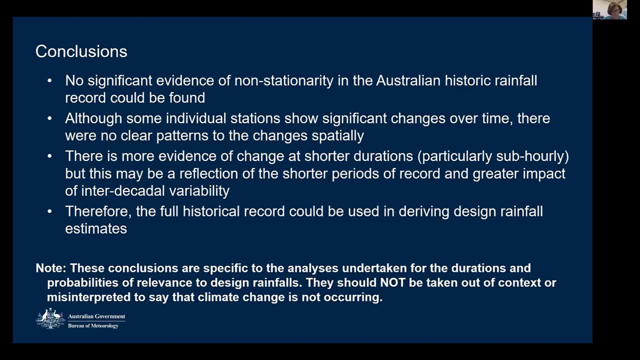 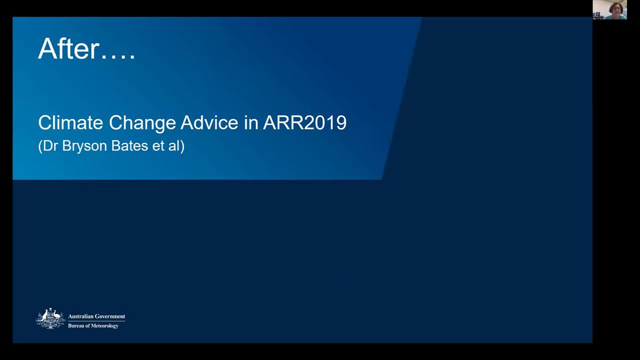 So I just need to make that clear so that people don't use these results inappropriately. We move now onto after- after we've spent our years designing the design, rainfalls. how do we incorporate climate change when we're looking at designing infrastructure? 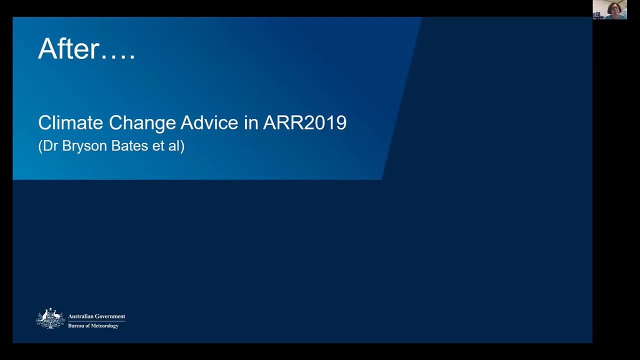 and particularly infrastructure, which we want to, which has a design life of longer than 20 years. And again, what I'm presenting here is the climate change advice it's provided in the Australian Rainfall Runoff and which is largely the work of Dr Bryson Bates and others. 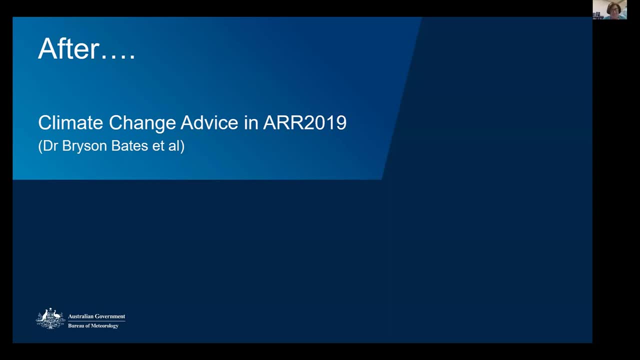 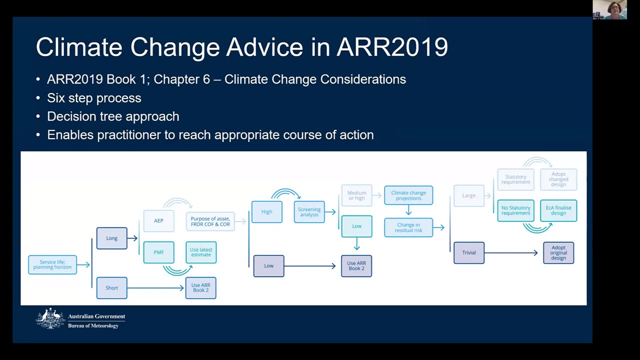 And Bryson is part of our brains trust today. The climate change advice in ALNR 2019 is very systematic. You can find it in book one, chapter 16.. It's a six step process. It's a decision, It's a voluntary approach. 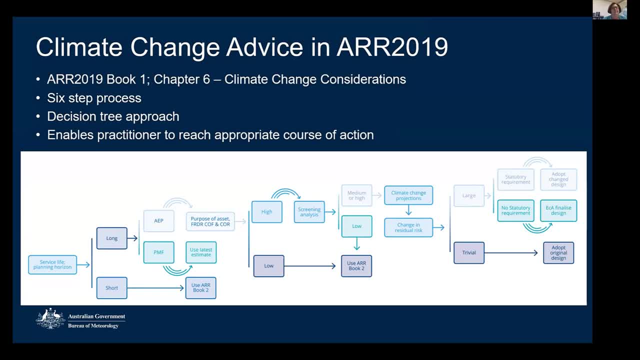 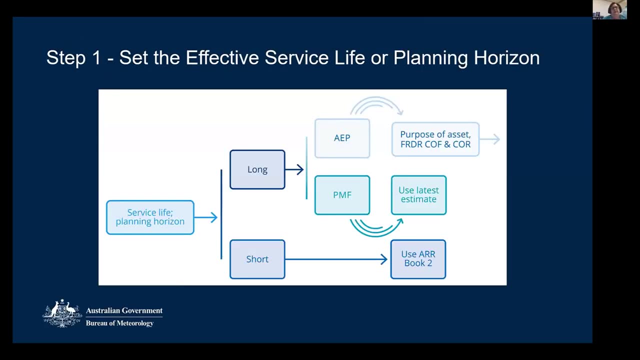 So it's basically a risk assessment which enables practitioners to make a decision as to what they should adopt when considering climate change with design rainfalls. The first step is look at the effective life of the structure. Like I said, if the structure is only going to be in service for less than 20 years, then 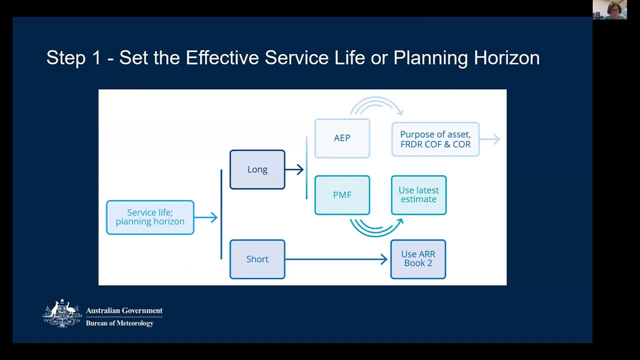 you just use the design rainfalls Which are in book two, chapter three of ALNR, If it's longer. you then look at the design standard Again. if the design standard is the PNF- the probable maximum flood- then you adopt the most up-to-date estimate of the probable maximum precipitation. 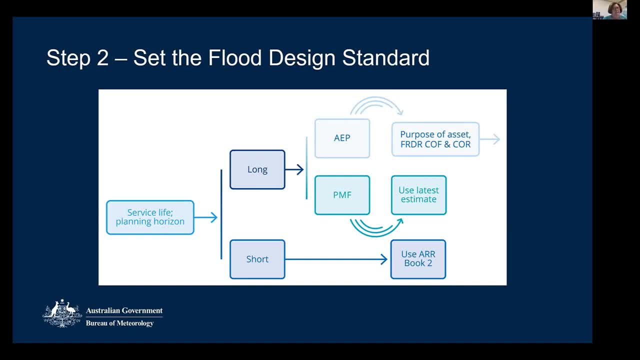 If it's the design standard isn't in the PNF, then you look at the purpose and nature of the asset And, in particular, if the design standard isn't in the PNF, then you look at the purpose and nature of the asset. 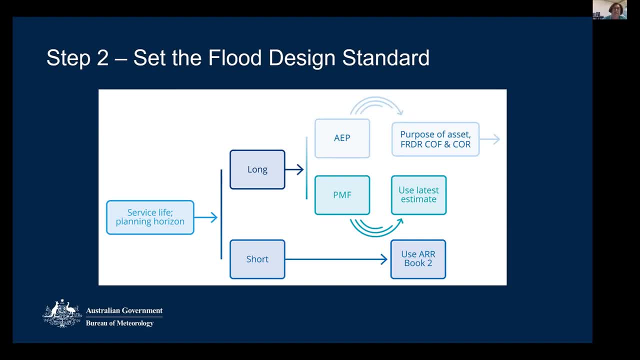 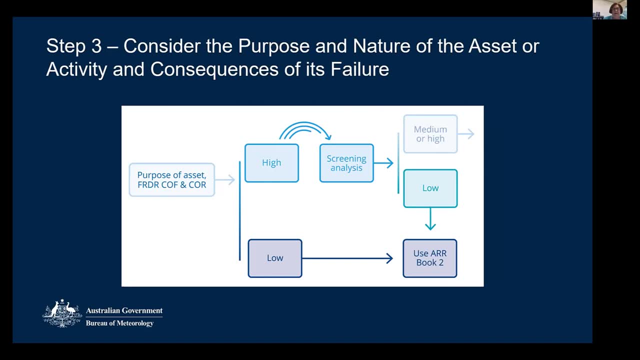 From that you're looking at the consequences of its failure. So we then move to step three, And what we're looking at is: what's the consequences of failure If they're low again, you just use ARR- The design rainfalls in ARR. 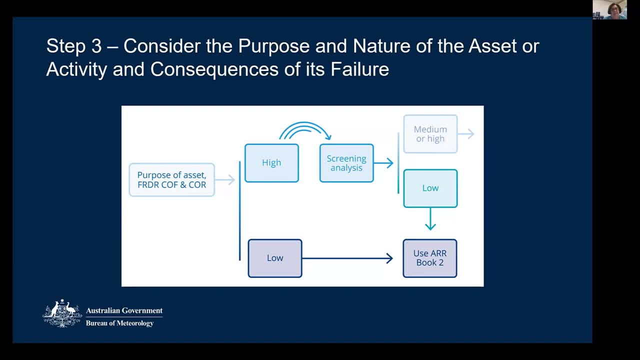 If the cost of retrofitting the structure for impacts of climate change is low, again you use the design rainfalls in ARR. But if it's high, then the next step is to move to a screening analysis. So step four: you look at what your design AEP is. 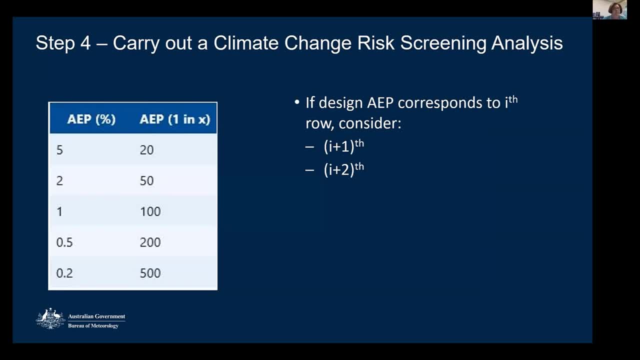 So if, for example, your design AEP is the 1% or the one in 100 AEP, you assess the impacts of the one in 200 and then the one in 500 in order to make just a screening analysis of whether. 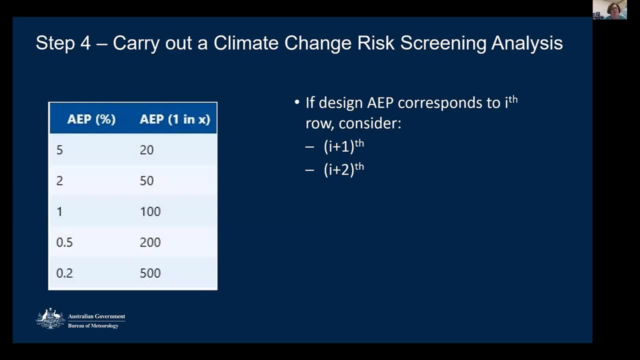 if the design, the one in 100 design- rainfall became more extreme and became more like the one in 200 or the one in 500, what would be the impact of consequences of failure? the cost of retrofitting If that was going to be high. then you move to the considering the climate change projections in step five. 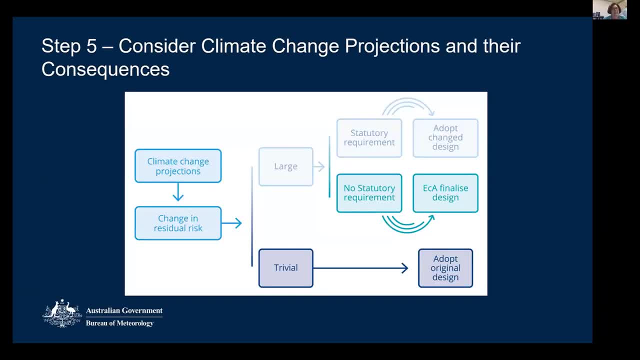 And that, again, if the The climate change projections indicate that the impacts is and the residual risk is going to be trivial, You adopted original design. Now, how do you look at the impacts of climate change, As Trey was saying? fortunately, there's been a lot of work done by this, by experts in this field and, in particular, in this case, CSIRO, who've developed the climate futures tool. 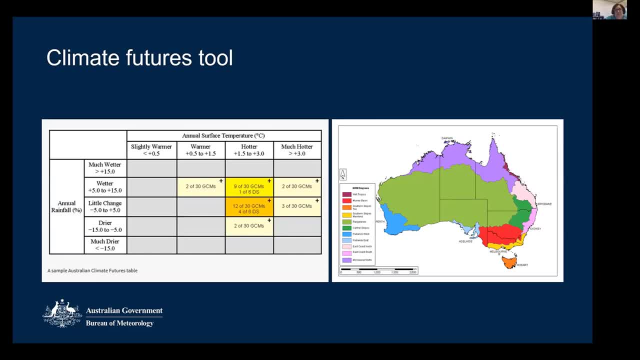 Which looks at for each of the natural resource management areas or clusters across Australia and which provides information on projected changes for GCMs, for global climate models for 14,, 20 year periods and for for RCPs or representative concentration pathways, And this allows you to identify what will be the potential impacts. 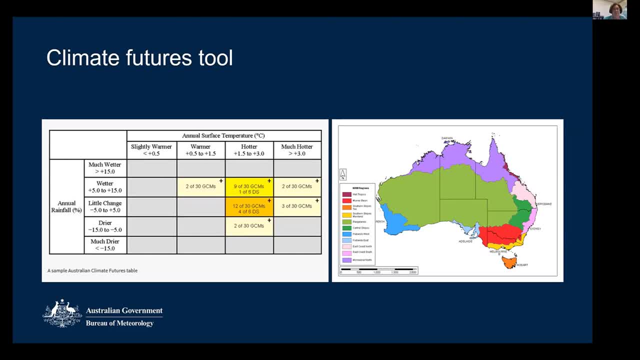 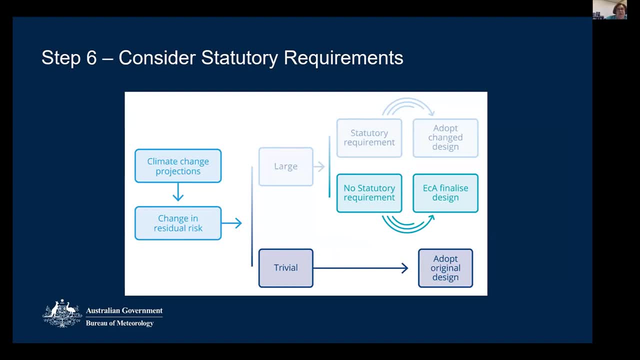 Of climate change on the particular region you're working in. If you do find that there's going to be a large impact for of climate change, there's the next step shows that there's a couple of approaches. The first is that the particular area where you're working in may have statutory requirements which specify what you need to adopt if the change due to climate change. 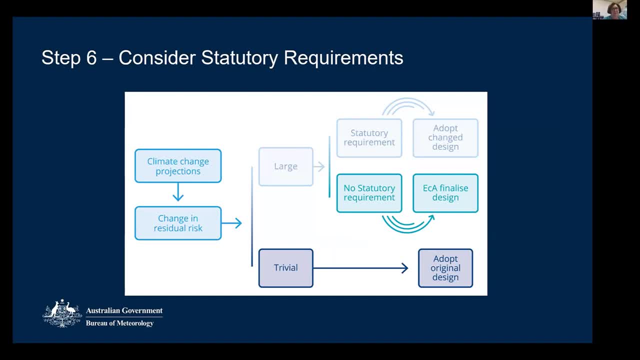 Or the risk due to climate change. Or the risk due to climate change, It's large. if not, it becomes an economic analysis and you're looking at what is the best economic in terms of a benefit cost decision. And this is the response that Bryson gave to one of the questions in the in the Q&A: that in the end, it becomes an economic decision. 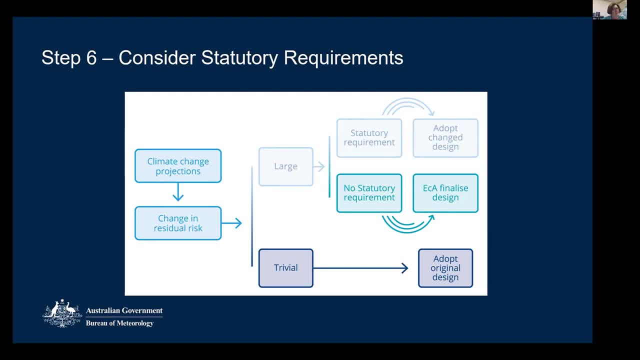 Now, obviously, the the decision tree approach is very, very salutary and very worthwhile. I'm not sure if you have any questions about the decision tree and the decision tree in its entirety, but if you have any questions about it, feel free to ask the questions in the Q&A. 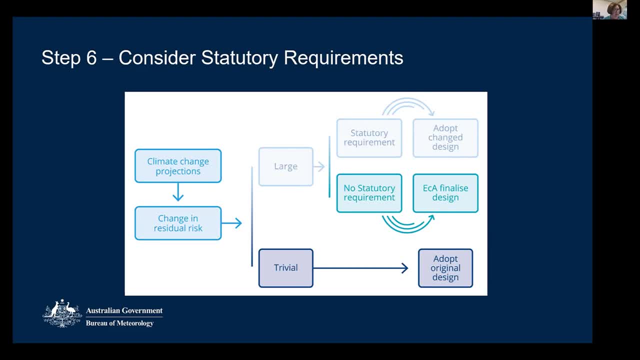 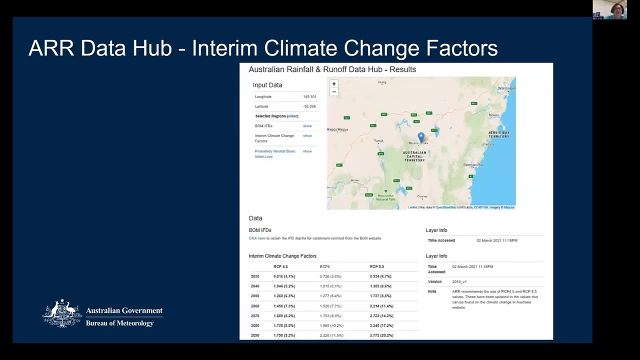 And then we may move on to the next question. I'm hoping that we have time for one more question. If you don't have any questions about climate change, we're not going to go through so that you are making an informed decision. But as hydrologists, as engineers, we do like to have things prepackaged and, as part of our data hub, slightly modified or slightly more detailed versions of the calculations that are undertaken from the climate futures tool are included in the data hub. 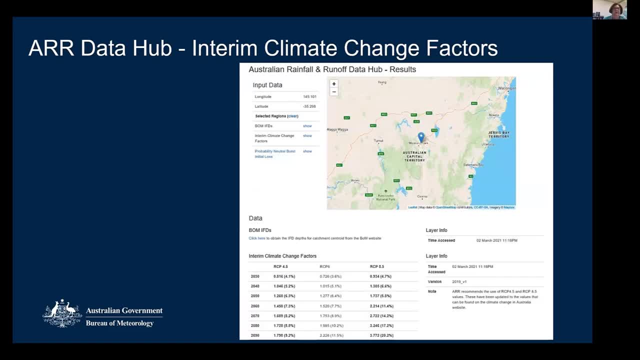 So, in addition to getting the information you need, such as the Bureau, design rainforests, climate change, climate change, climate change and climate change, we've also got the challenges of climate change or slightly more detailed versions of the calculations. 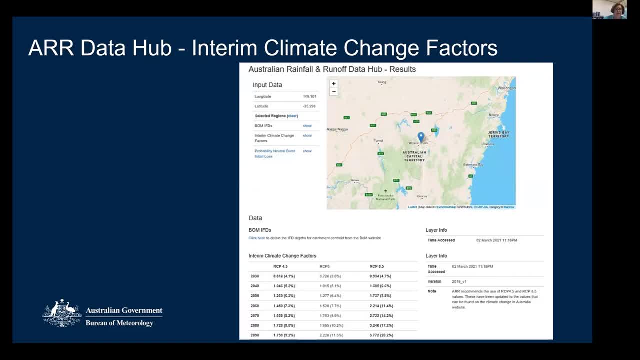 that are undertaken from the Climate Futures Tool are included in the ARR Data Hub. So, in addition to getting the information you need, such as the Bureau Design, Rainfalls and losses and temporal patterns, you also can get the interim climate change factors as part of the assessment. 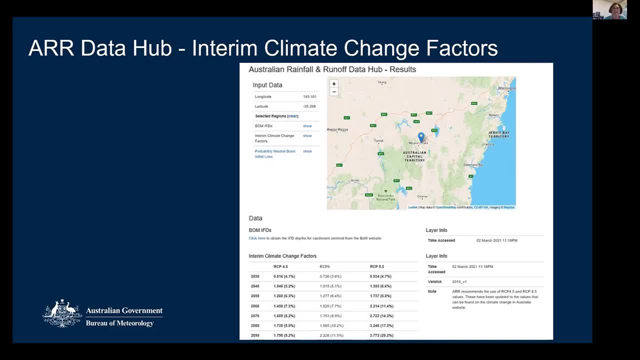 And the purpose of this is it provides you with the lower or the RCP 4.5 and the upper- RCP 8.5- climate change factors, which you can then use to determine the effects of both and then again make an economic decision as to which to adopt. 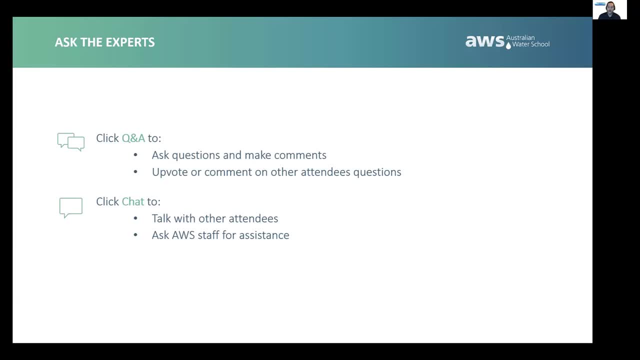 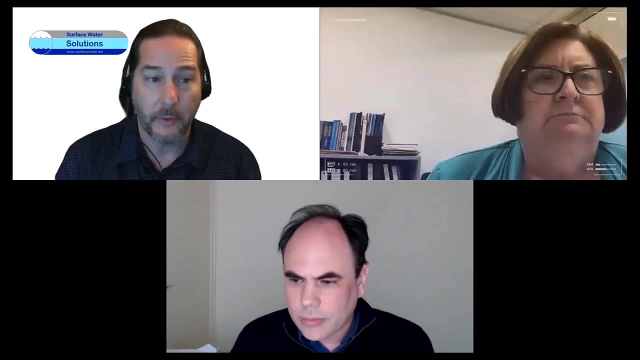 Thank you, Excellent Thanks, Janice. And at this point let's go ahead and have everybody turn their Turn their videos on, or their video feeds and their audio. And I do want to just highlight one quick question. This will be a yes or no question for you, Janice. 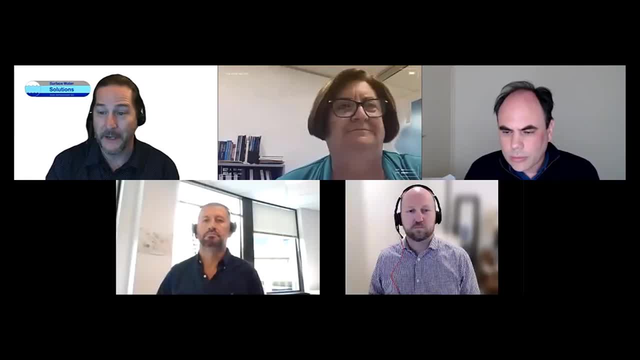 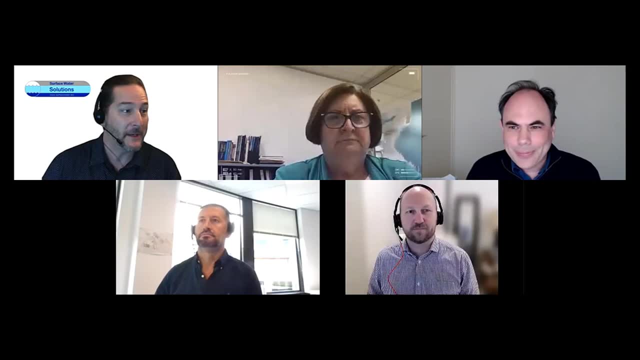 because the question that you actually answered earlier on the Q&A line had the most upvotes out of any of them. Almost 20 people in our attendees out there said they wanted to know for the PMP and PMF if I'm designing for that, do I need to ramp it up? 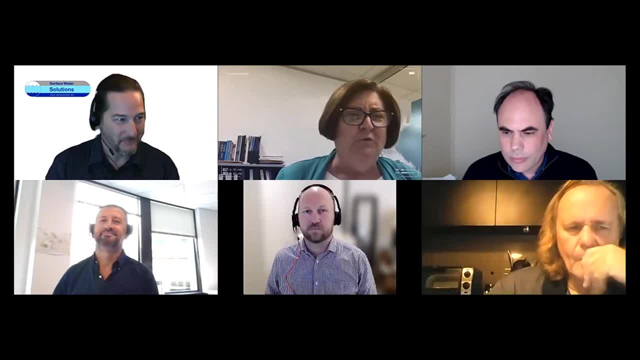 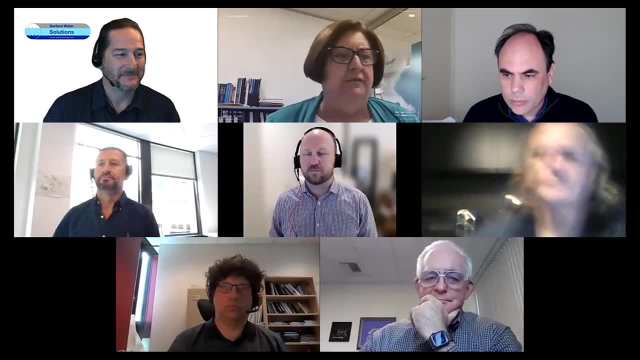 Yes or no? The short answer is no. No, I saw that one. It's a qualified no. As I put into the chat, there's not been a lot of work done. There's a report that you can find on the Bureau web page. 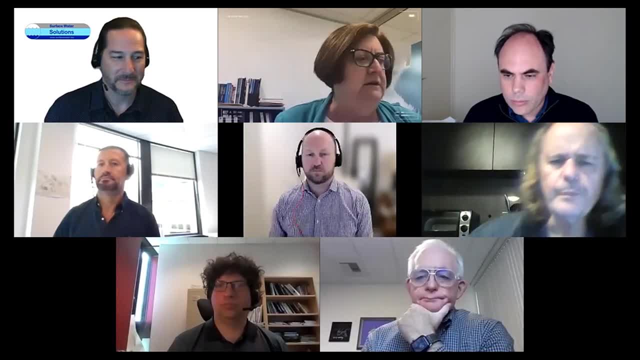 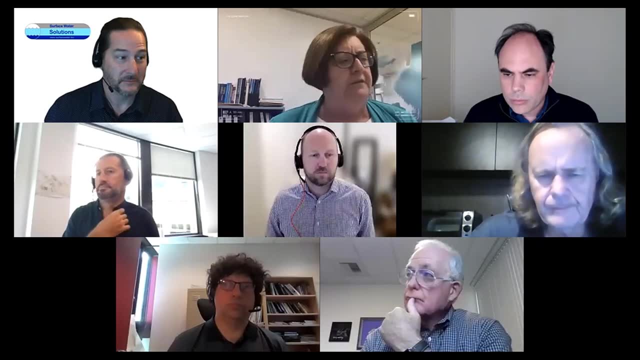 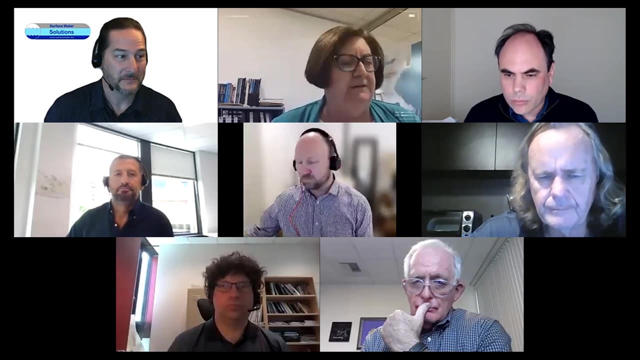 of a study that was done in 2009 on climate change and problem maximum precipitation. Not unexpectedly, what was found was that the study concluded that you can't confirm that PMP estimates will definitely increase under a climate, a changing climate. Part of the reason is, you know, we're still trying. 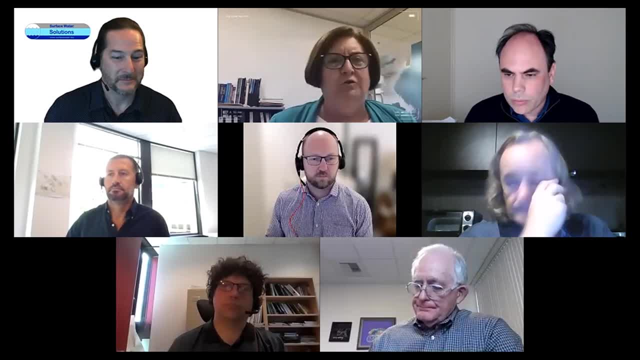 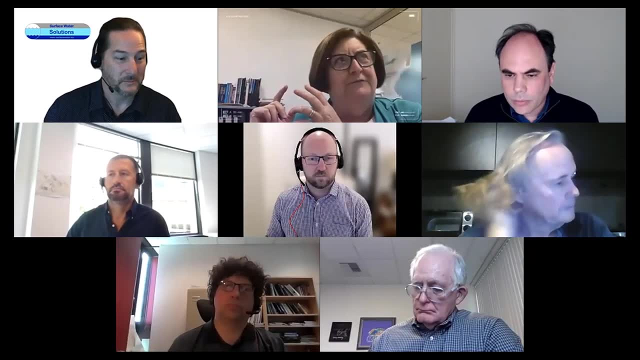 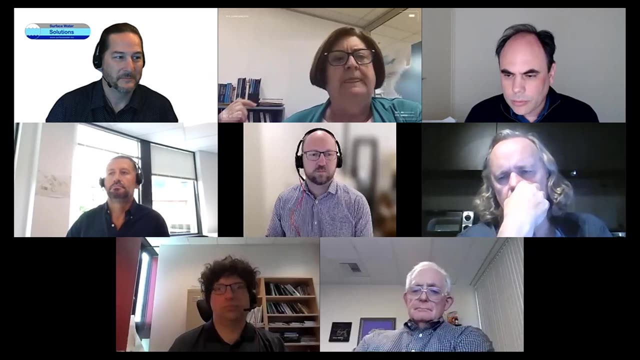 to get a handle on the impacts of climate change on your normal, if you like, design rainforests. Until we get that, we, you know we have limited opportunity to understand the impacts on that most extreme problem: maximum precipitation, But again in keeping with the advice in ARNR. 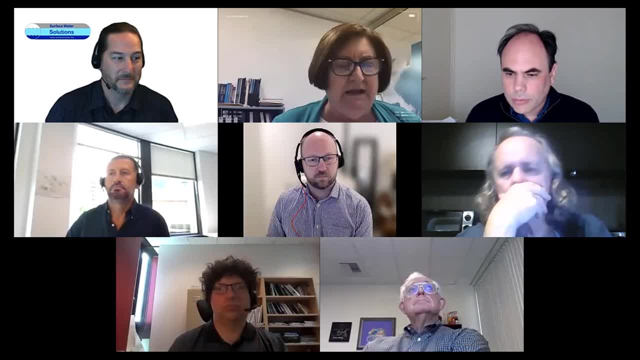 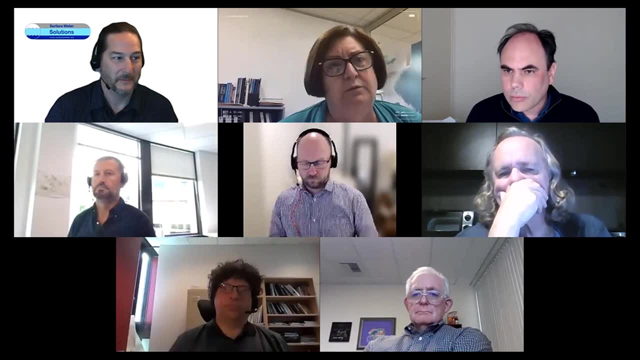 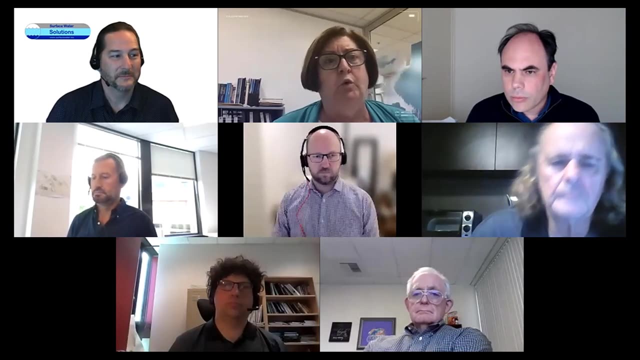 the advice that's being provided. you know today, if you think, if there are concerns about it, undertake a sensitivity analysis To see what the effects are And also to look at the cost of increasing your design, to all, retrofitting your dam, which is never cheap. 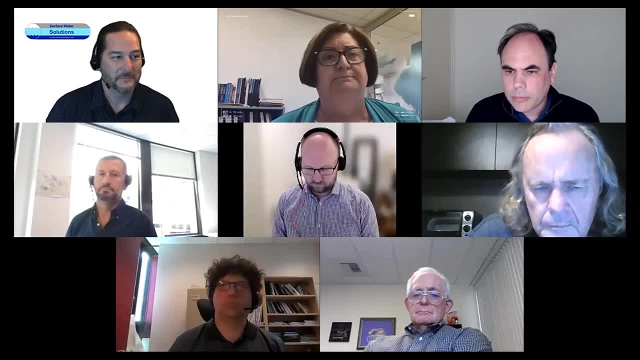 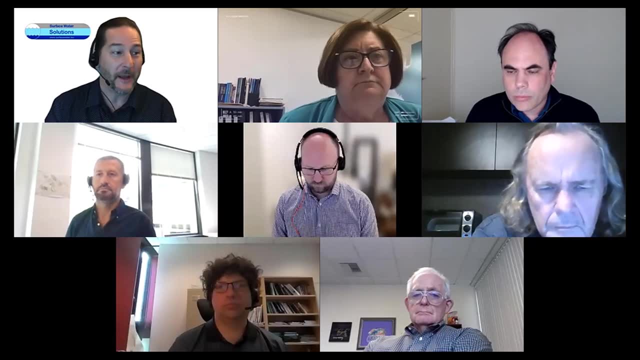 if there were going to be increases in PMP estimates, Thanks, And that's again. this is where, with a panel like this, I've seen Janet speak at a number of conferences in the past when we used to do these things live. 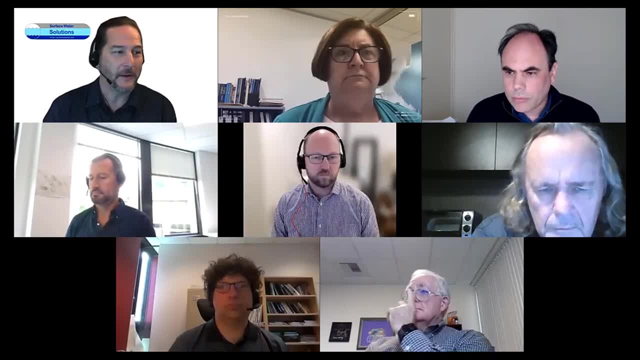 It's awesome to have these kind of forums where we can all get together. Afterwards, you know, we'd have the chance to have some banter back and forth and you'll go up to the presenter and ask your own specific questions. 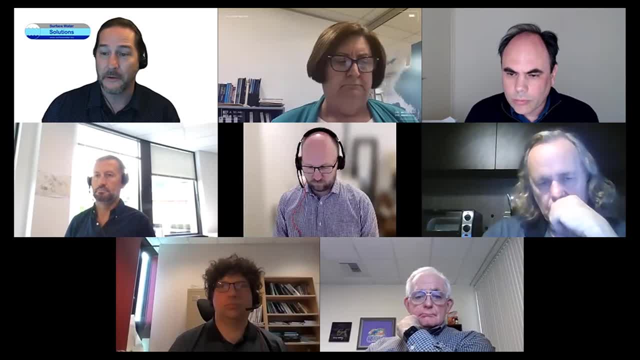 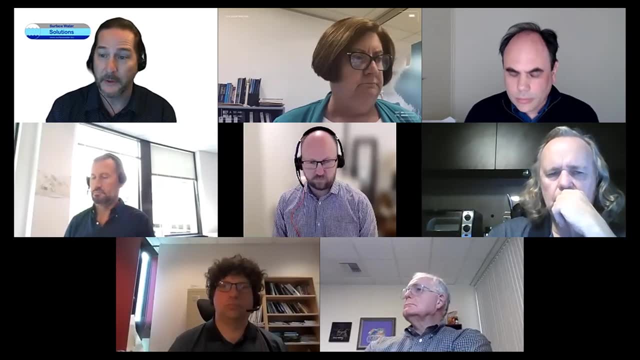 So with this forum, it gives you the chance, as attendees, to put in, you know, to upvote questions and say, yeah, I'd like to hear more about that. We do want to hear from the speakers, from the panelists who have been frantically answering questions. 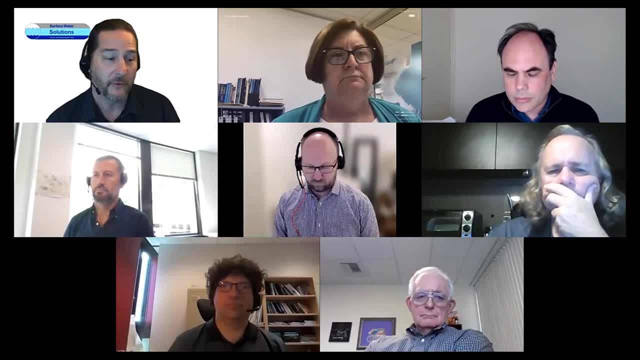 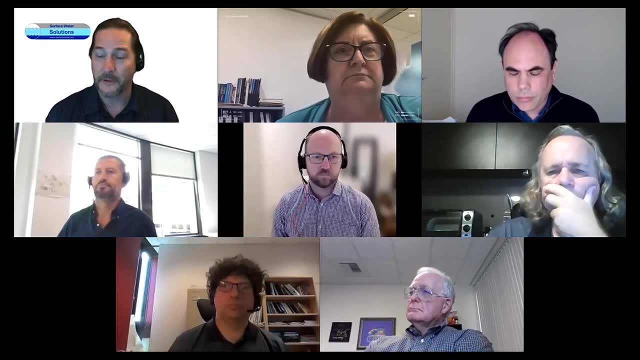 during this entire session, And maybe what we'll do first is just have each of you address one question that you've had on the Q&A line, maybe focusing on those that have been upvoted the most, And let's go to our CSIRO attendees first. 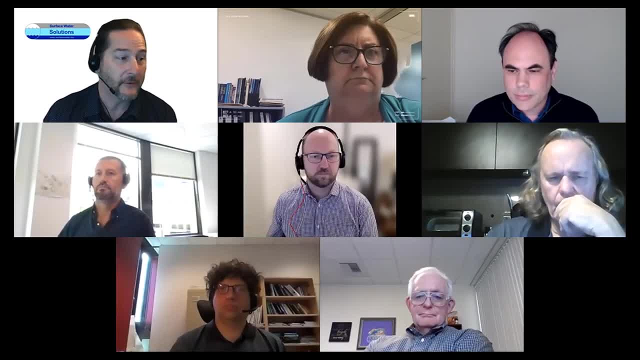 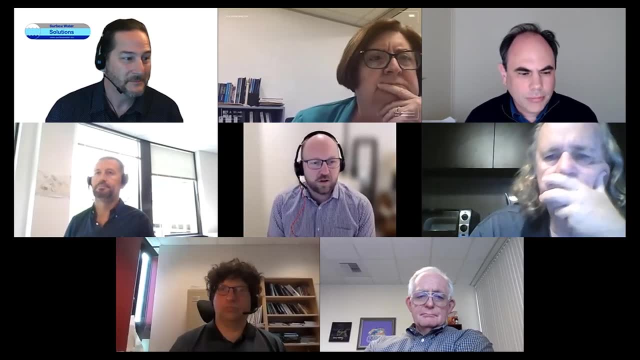 Let's go to the CSIRO attendees. Let's start with Tony. Is there anything that you've answered there that you want to highlight? Any of the questions that you would like to highlight for the rest of the attendees? Thanks, Craig. Perhaps I'll start with a question from Mark Lavelle. 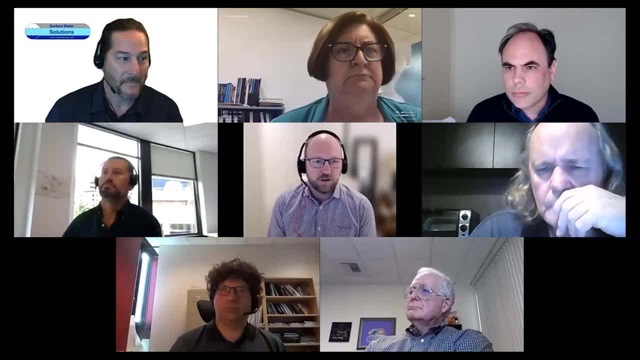 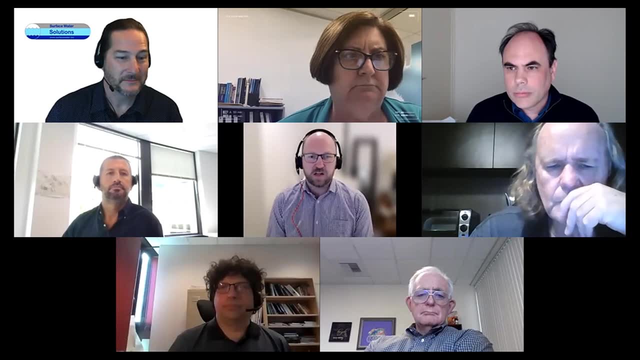 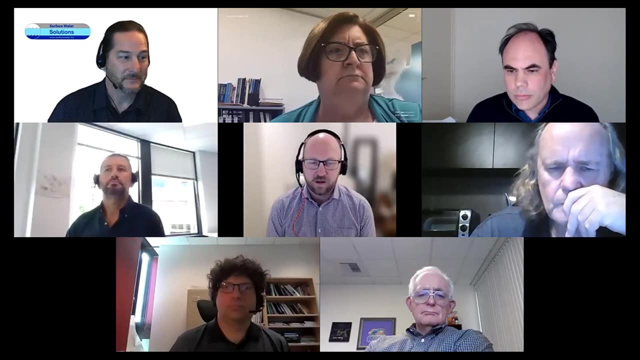 who's? I'm just answering this in the text at the moment. He's asking about why the ARR guidelines always apply an increase to precipitation, even in areas where the main precipitation is projected to decrease. He's also asked about regions where maximum precipitation decreases. 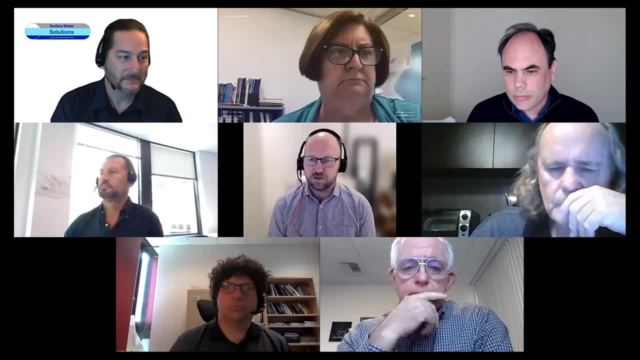 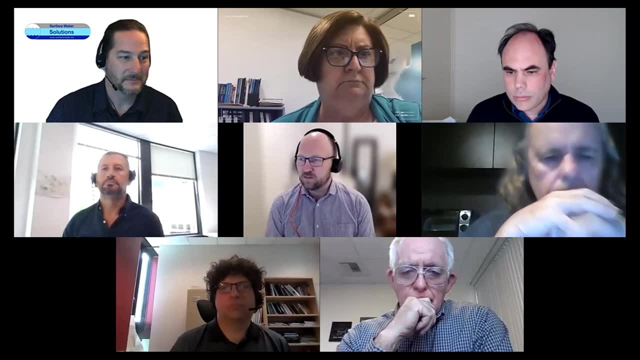 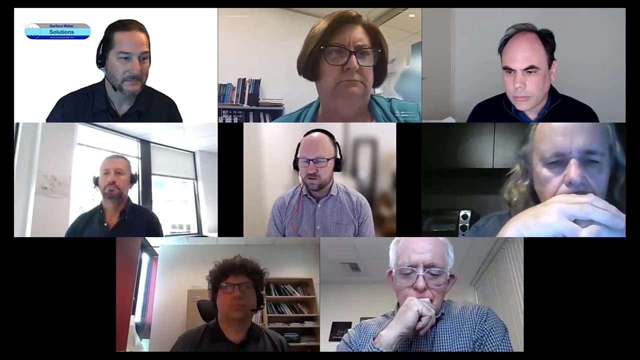 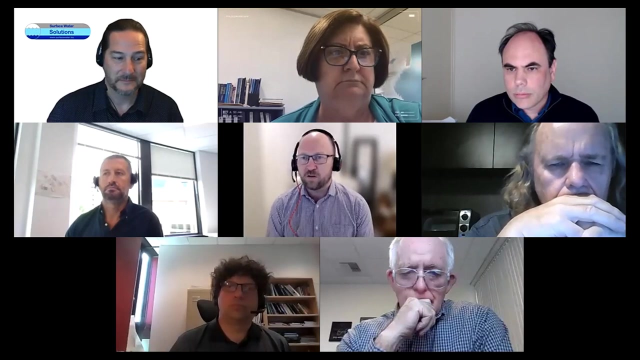 But in the most recent climate projections for Australia we found that most regions in Australia have a reduction in mean rainfall, but the daily maximum, the annual maximum daily rainfall, goes up all across Australia. So essentially the guidance for an increase in extreme rainfall is based on that kind of information. 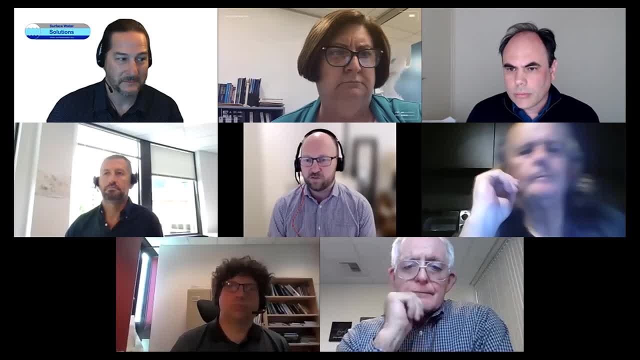 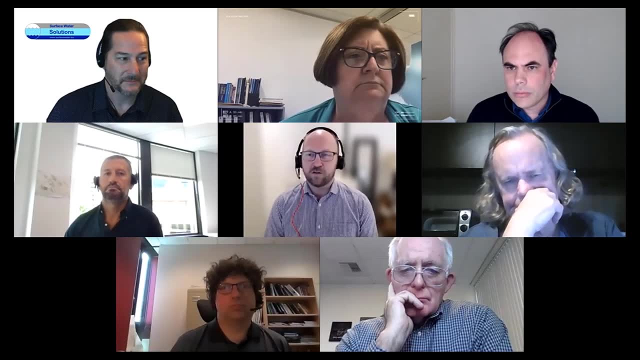 that even in regions where we expect mean rainfall to go down, extreme rainfall is expected to go up, And that's why the recommendation is to increase the design rainfall everywhere. Yeah, No thanks, And that's again. this is one of these questions. 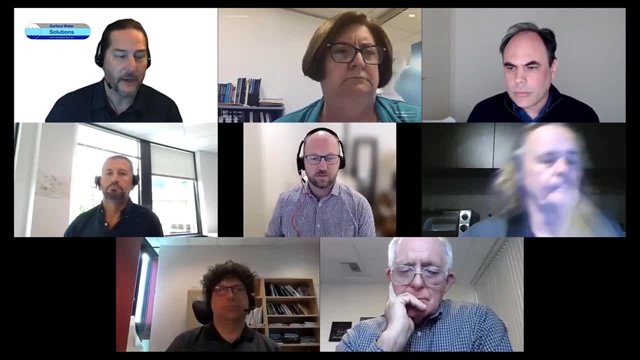 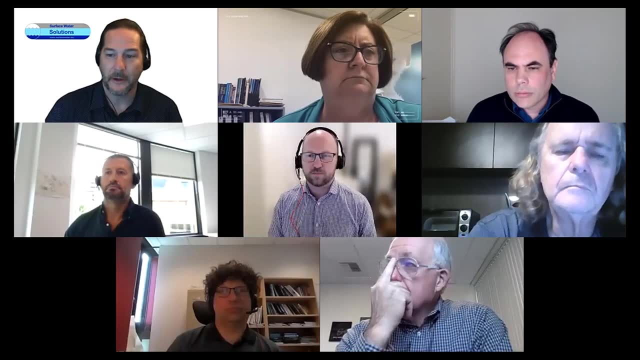 for the practitioners- And seeing today's presentation- thanks so much for all those slides- It helps to show that there is a reason behind that and we can back it up with some of the records and some of the analyses that have been done. 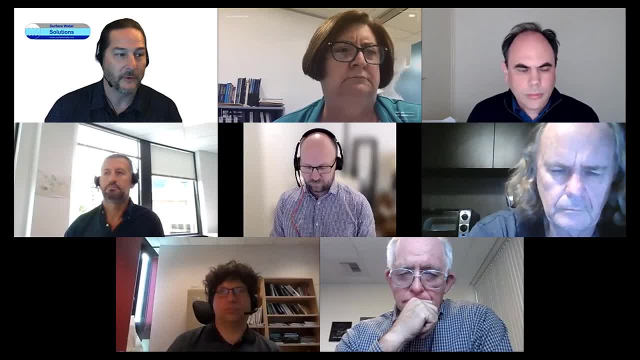 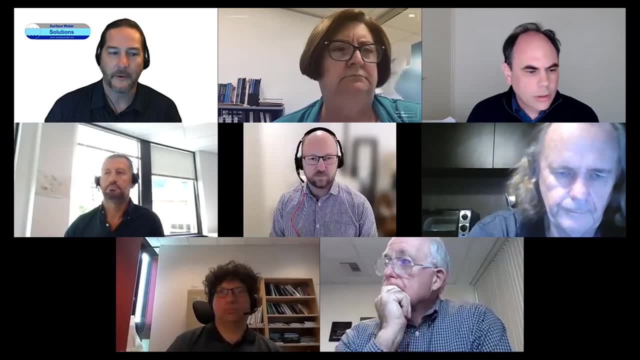 And there is some solid science behind those decisions. It's not just a random thing we're picking out of the air. Marcus, over to you. Is there anything you wanted to highlight from the questions that you've answered? So I'm just struggling to keep up with the questions. 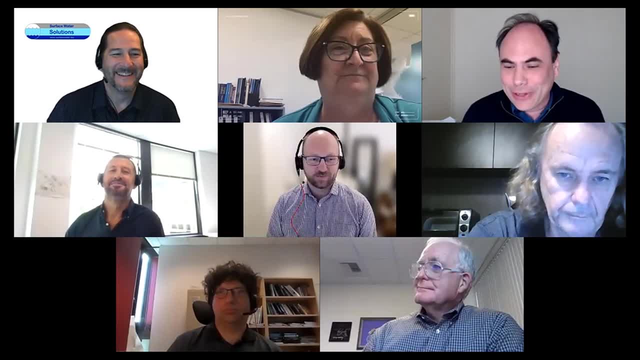 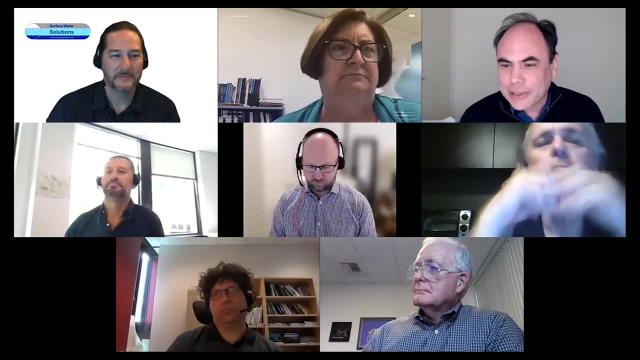 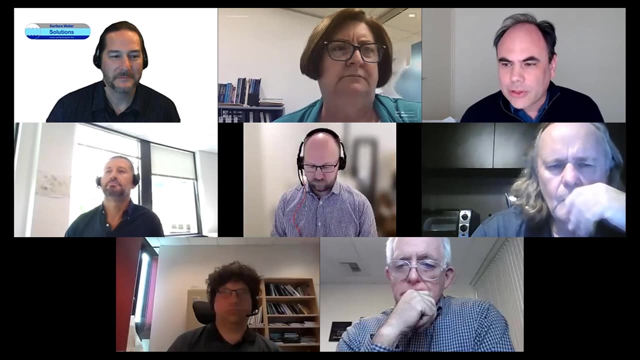 Exactly. I'll mention some that I've got to so far. Apologies to the audience for not getting through them as quick. So one of them, a question from- and I apologize for pronouncing your name wrong- Amaran Rindo Rindo, who was asking about the best method and software. 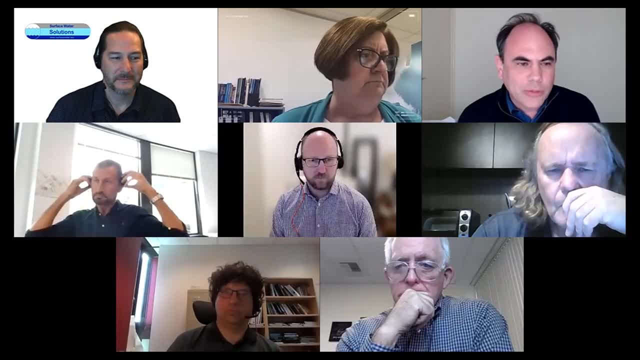 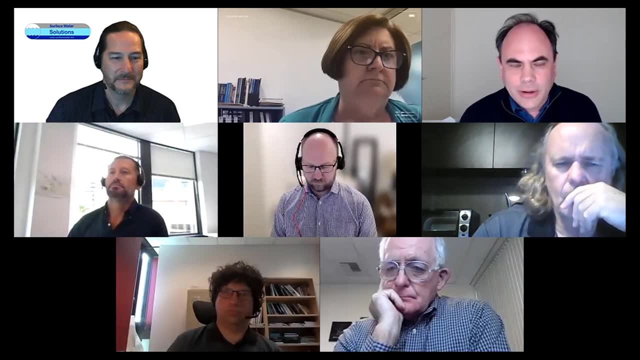 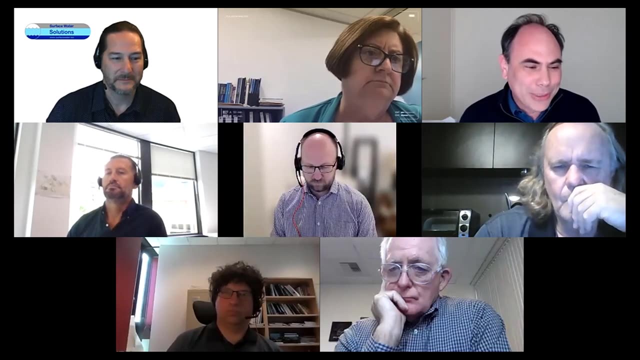 for calculating the effect of climate change on precipitation, extreme rainfall and its effect on dams, And I guess, just in general terms, it's often. I guess we often recommend using a few different methods, because it's difficult to have a perfect method. 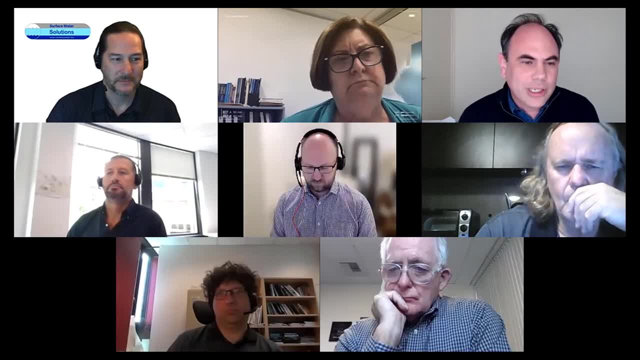 particularly when it comes to climate change, or one perfect data set. So often there'll be national climate projection data sets which have been curated so that there's some reasonably good quality. For example, in Australia there's the climate change in Australia website. 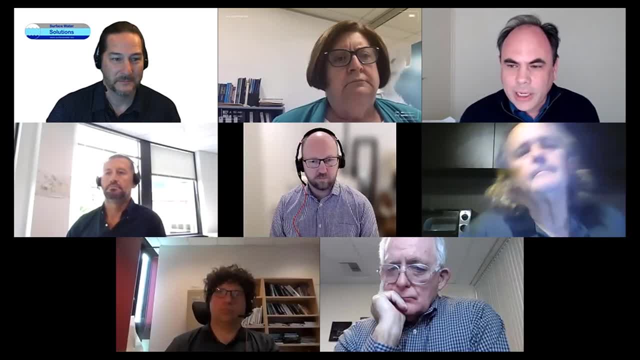 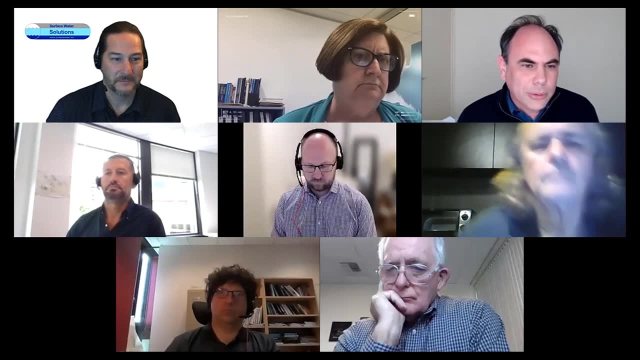 It's a good source to get some information about that And that can give you a good idea of some of the range in these predictions, as well as the consistent trends across all the models. And then there was also a question on its effect on dams. 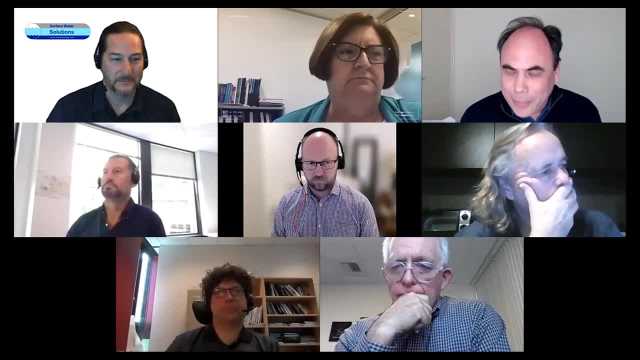 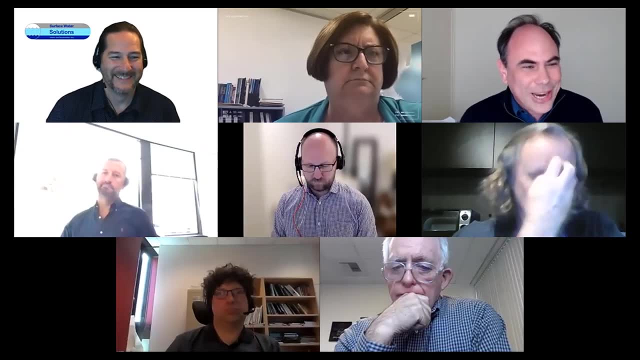 And I guess my fellow panelists may have a question on this. but when it gets down to that level of detail, I think I agree with the sentiment before about letting engineers design the dams and things. It's very much a co-design, like the climate scientists can help. 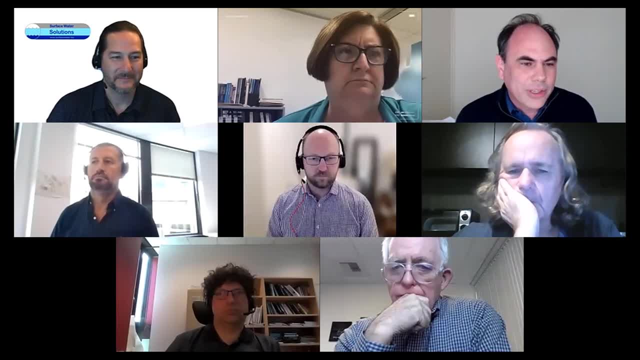 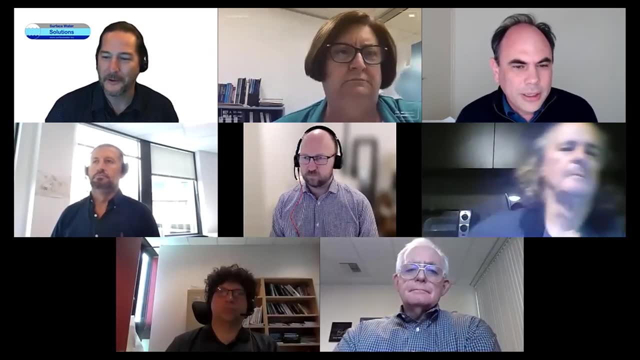 but they can't answer that question by themselves. They can only work with the engineers to combine that information Sounds good. I appreciate that answer, Bryson. I've seen you answering a few of these To highlight. Yes, I think there are a couple of things. 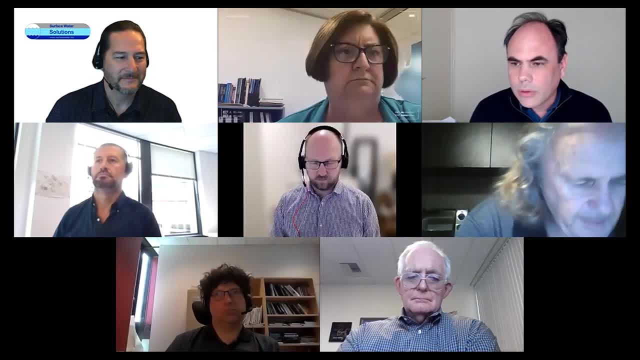 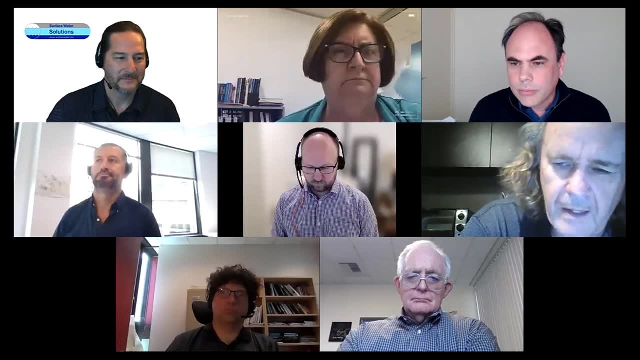 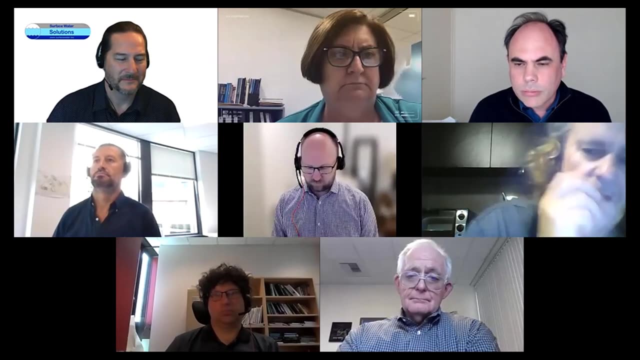 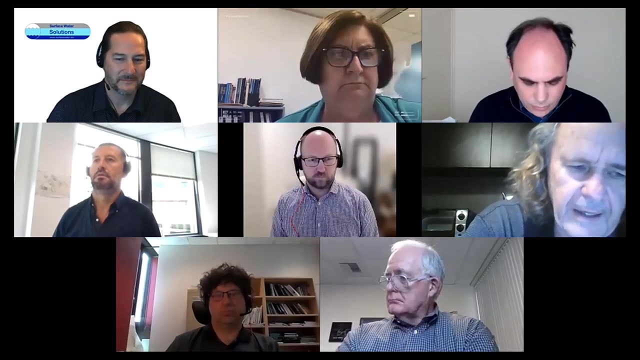 One is: there seems to be quite a few people who have very good questions, but I would recommend, in terms of what approaches to use and so on. And, look, I really would recommend they have a look at the IPCC working group to reports to get an idea of what scientific literature is out there. 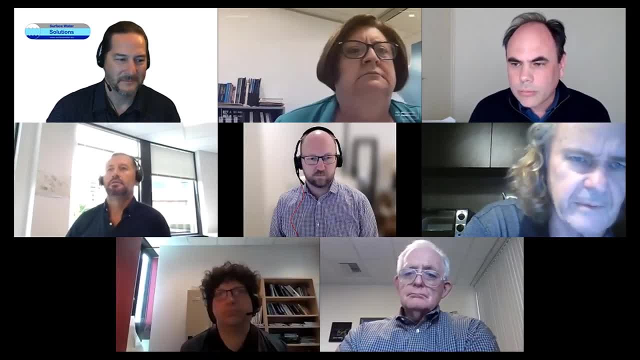 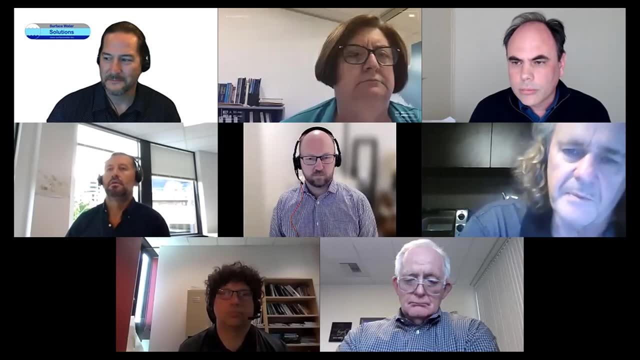 on their particular subject and to dig a little bit deeper and actually read those papers, see what people models people are using, How they're approaching their problems, and so on. I think that's the only way at the present time that you'll be able to move forward. 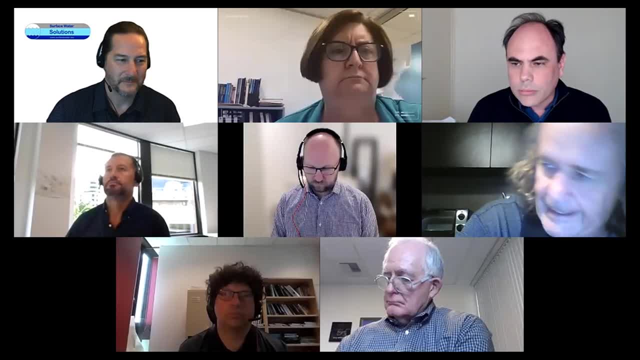 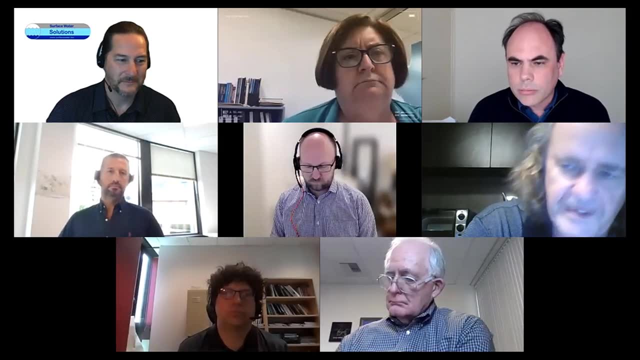 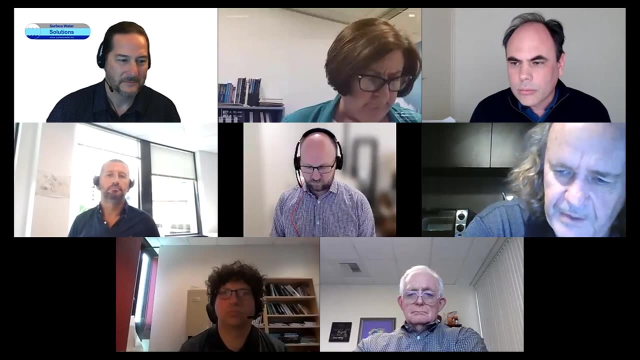 unless you have access to like a university library and can do some research in terms of finding out what information is out there. in general, A lot of people are very focused on the engineering component of the problem But, as Janice mentioned, I responded to someone saying: 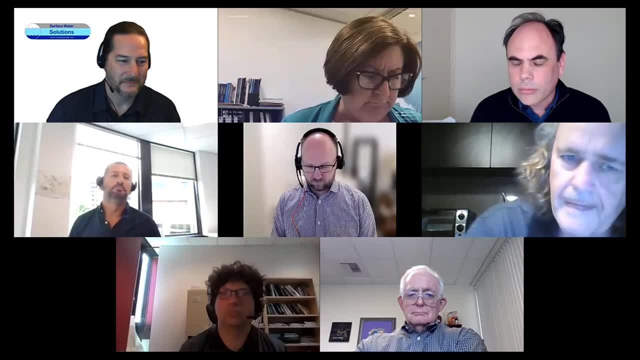 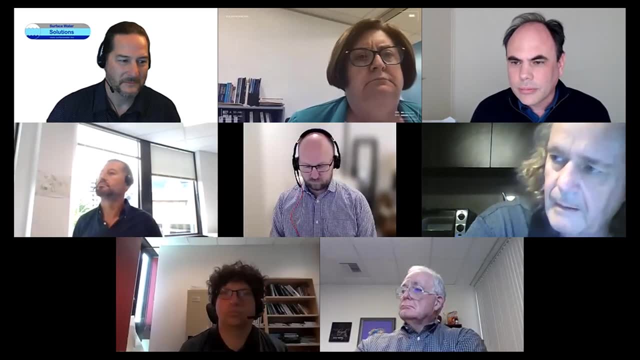 well, at the end, there's an economic decision to be made. in terms of the climate change information you have- what the projected impacts are, how much is it going to cost to protect against those impacts and what are going to be the benefits? 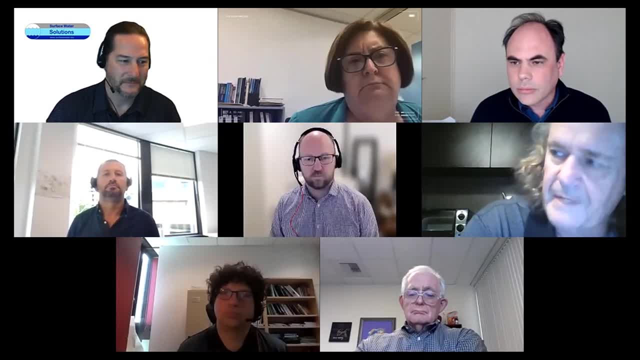 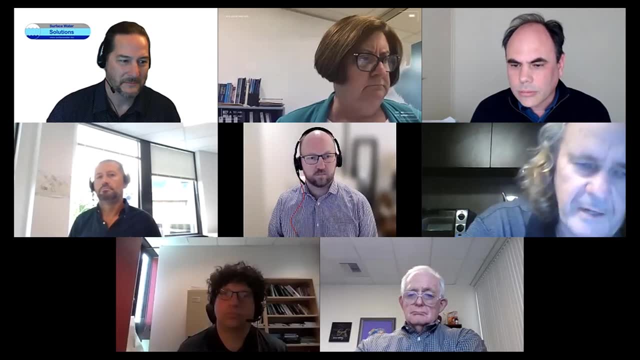 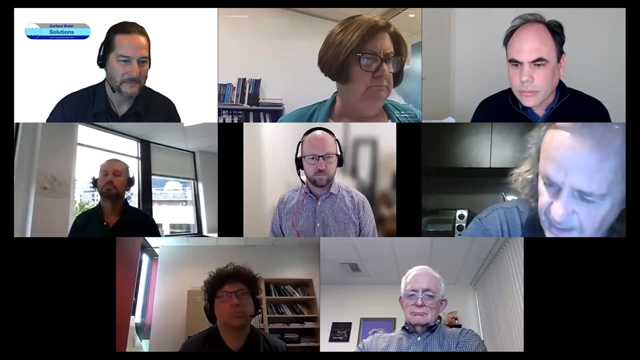 And at the end of the day there is: that's an economic decision, I mean, in terms of engineering, we are responsible for protecting human life, and that's different. But I remember a philosophy once told to me some 20 odd years ago. 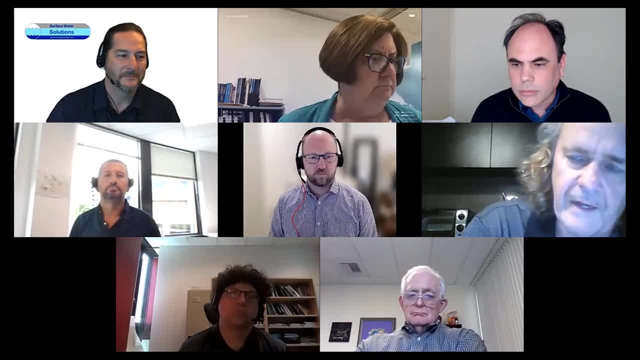 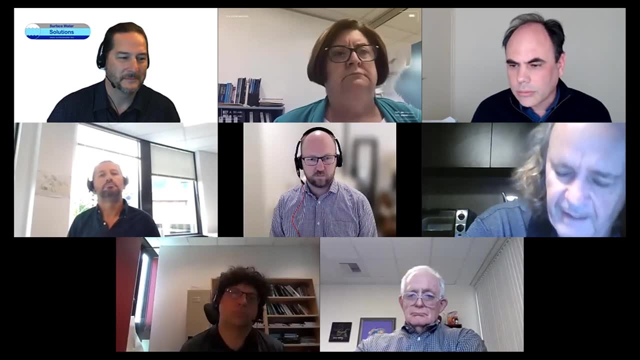 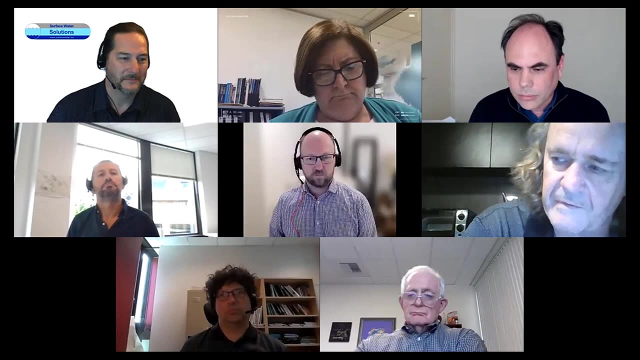 by a fellow engineer that, instead of designing things to be fail safe, we should be designing them to fail safely, And I think that's something we should be really starting to think of in terms of incorporating climate change into designs, because if we start looking at very extreme rainfalls- 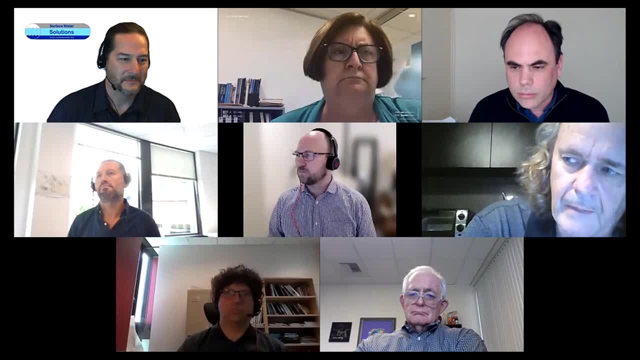 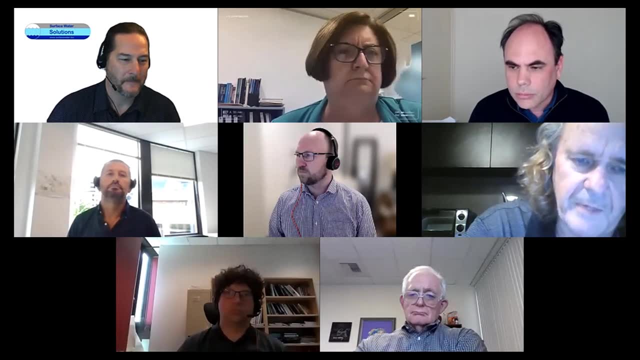 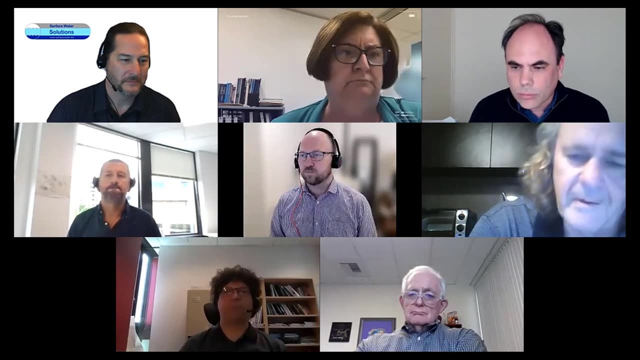 there's a lot of possibilities there. We're going to have very expensive infrastructures and there might be simpler ways of addressing the problem, particularly in terms of staging, retrofitting. So if we start out with a design that can be augmented over time and with a reasonable economic cost, 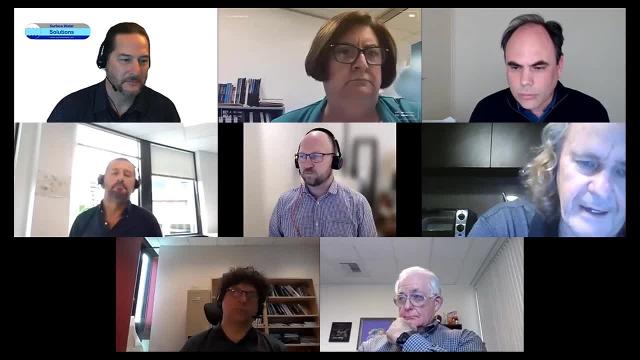 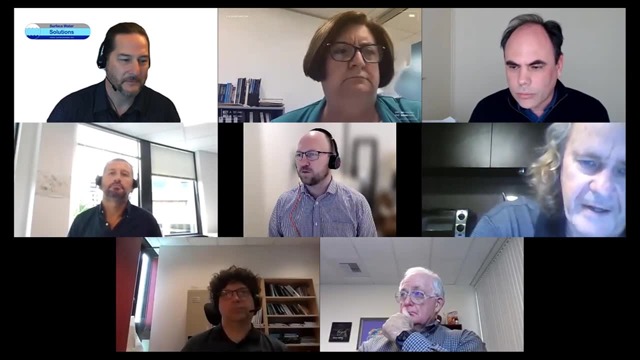 then I really do think we start to need to engage with economists who can talk to engineers on this particular topic, Because at the end of the day, you're going to have to convince someone that the dollars you intend to spend are going to be worthwhile. 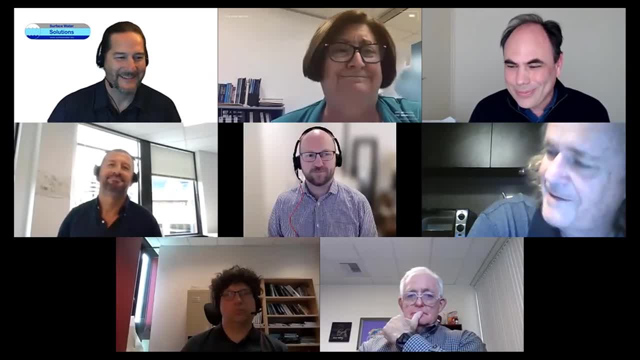 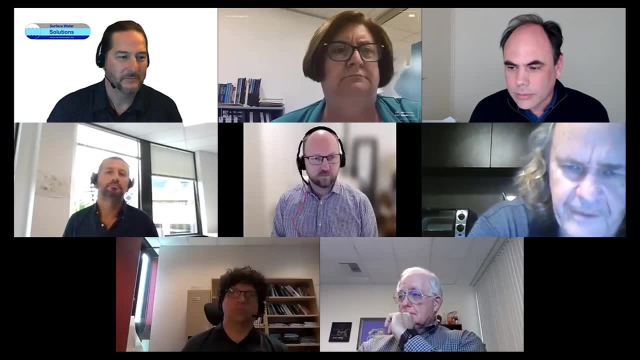 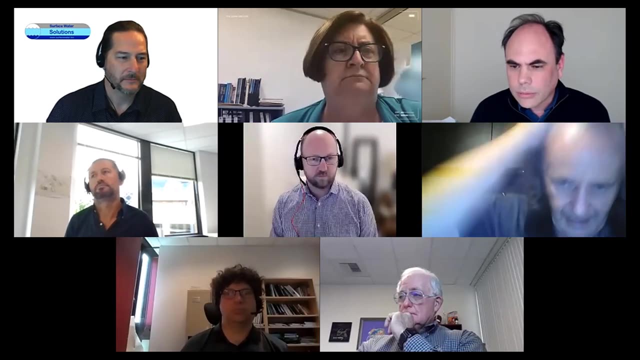 And that might even be a politician. Yeah, I think there are a few others that are quite technical and will take a little bit of effort to answer properly, But I think the last thing in terms of the climate change advice and the Australian Rainfall and Runoff- 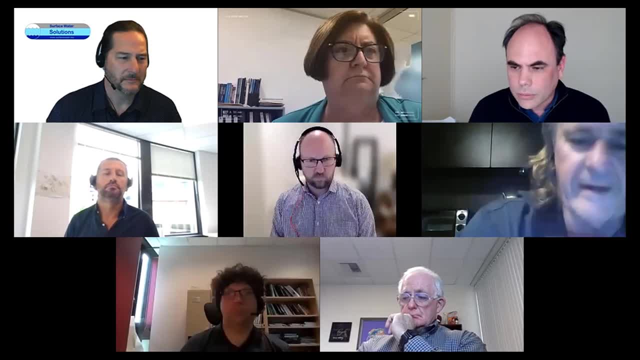 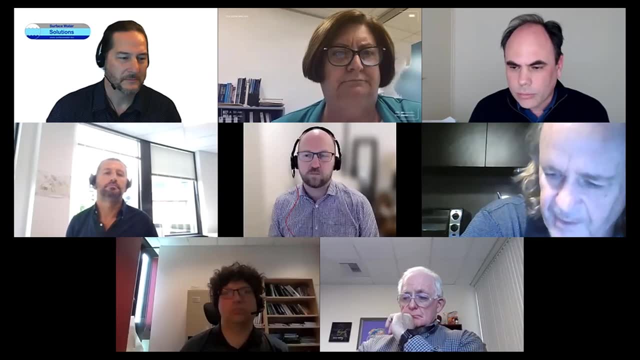 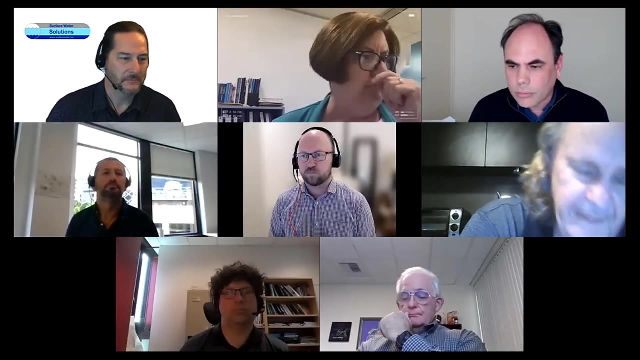 that originally was intended to be an interim document. It's meant to be updated as climate change science progresses. One of the questions was talking about the growth rate being only 5% rather than 7% in the Clausius-Kleppion relation. 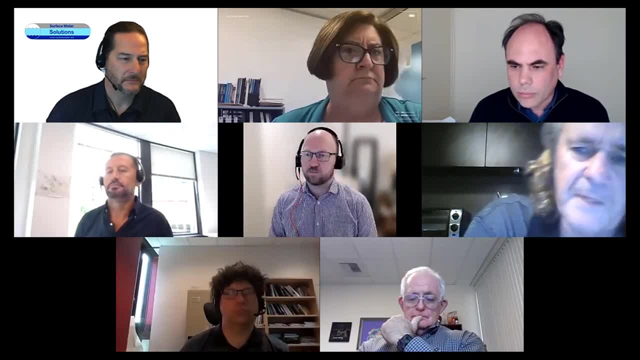 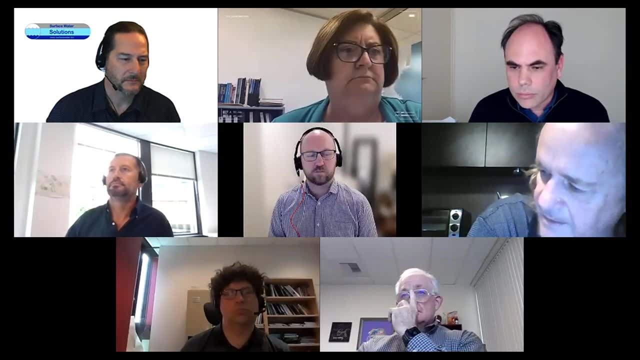 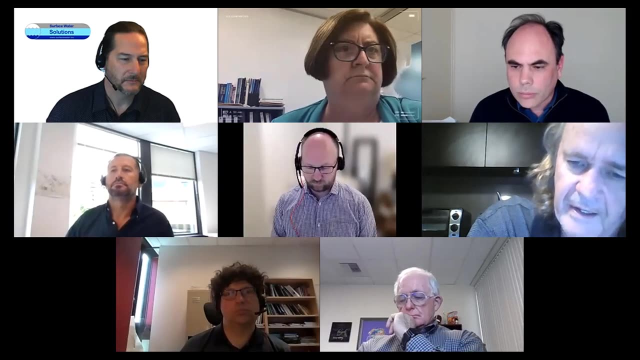 Yes, we decided to use five because at the time there were some papers around indicating seven degrees Kelvin. I think that literature has probably grown And I think at some point that part of AR and R is going to need to be updated. 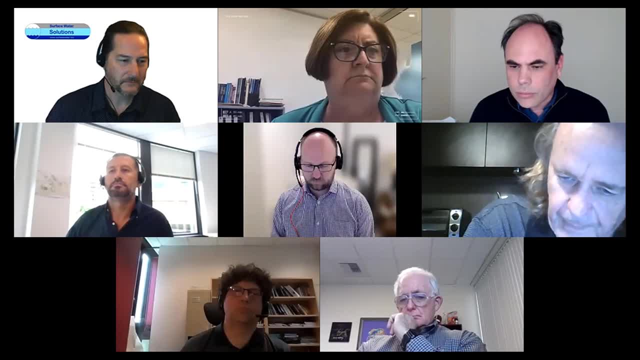 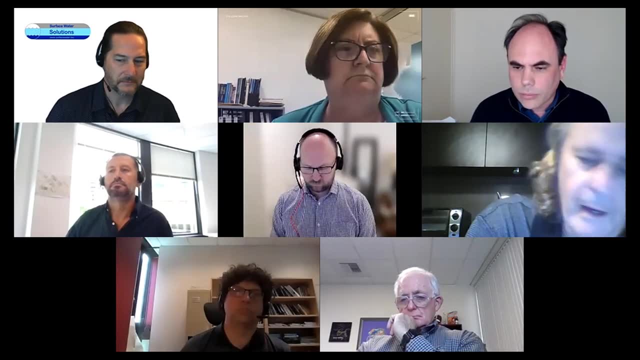 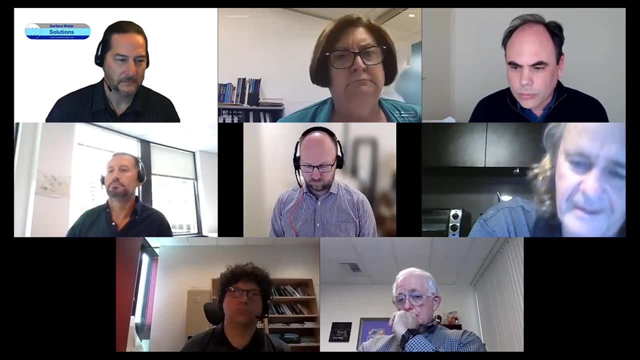 I would also say at the time that equation was the only one really we had any reliability in terms of giving people guidance. I think some of the slides that Jason presented and some of the other slides are going to need to be updated on other factors. 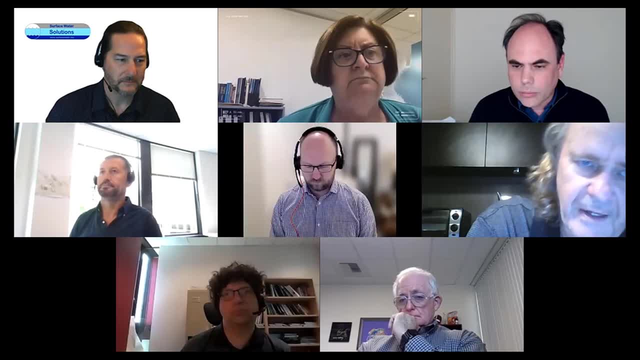 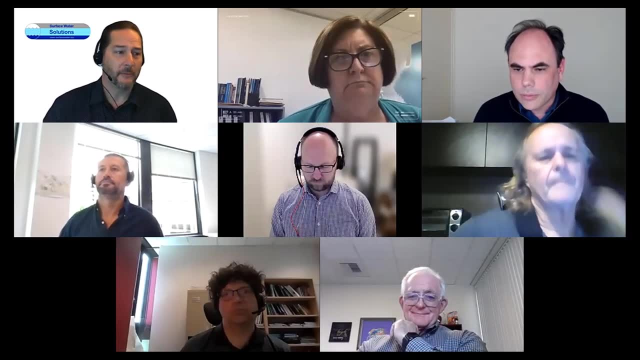 other than just the thermodynamics are going to be important too, But we're going to need more research in that area before we can give engineers more guidance, So I'll stop there. Thanks, And as you mentioned, there are a lot of technical questions here. 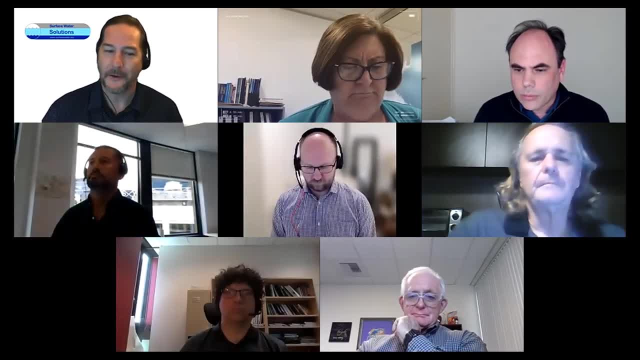 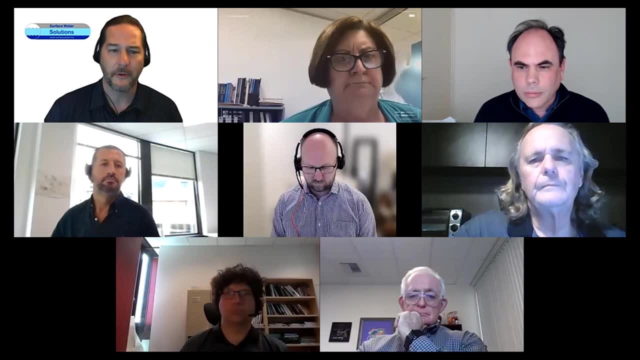 And again, what we'll try to do is compile these, I think, so that those who watch this on YouTube later on don't get deprived of the knowledge base that's gone into answering some of the questions so far. Clinton, if you want to pick one question, 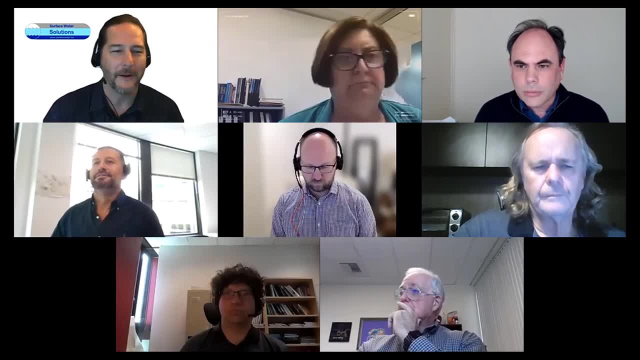 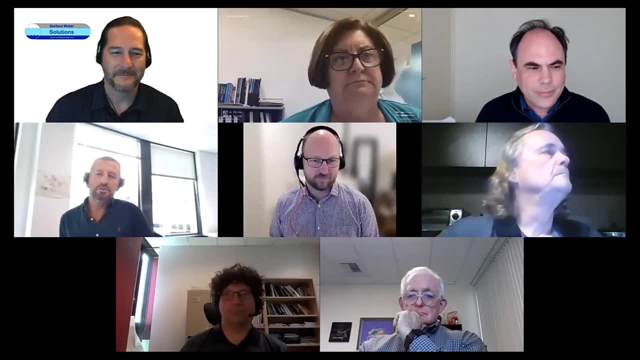 that's been addressed. I've seen you hit a few of these as someone who's transitioned from or transitioning from the public and private sector. Anything you want to highlight there. There was just a question from the Pacific which I think I'll pick up quickly. 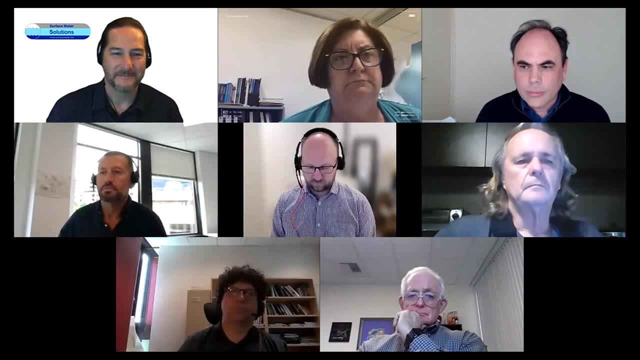 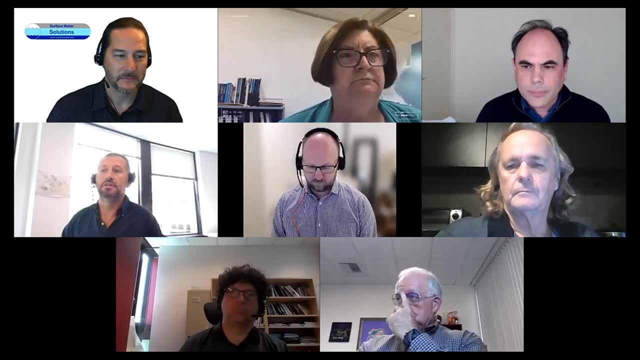 is that there was a question from someone in Fiji and it was around- should they expect more extremes for rainfall? And I'd really refer them to the Bureau of Meteorology and the Pacific Climate Change site, which I'll send through in the links. 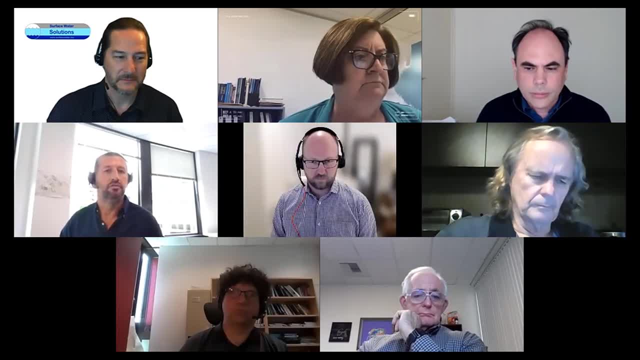 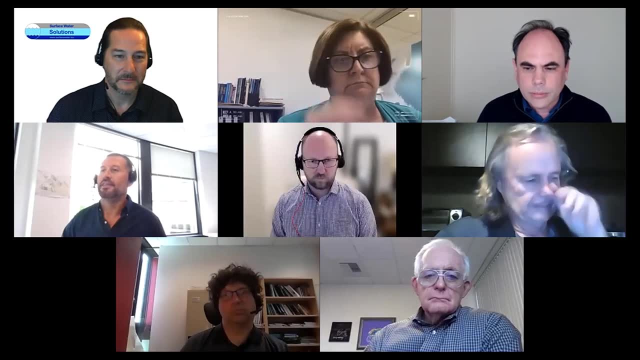 To really get detailed information for each of the different island groups across the Pacific. It's hard to give general advice for locations that are so far spread across the ocean. And then there was another question from Queensland around paleoclimatological evidence. 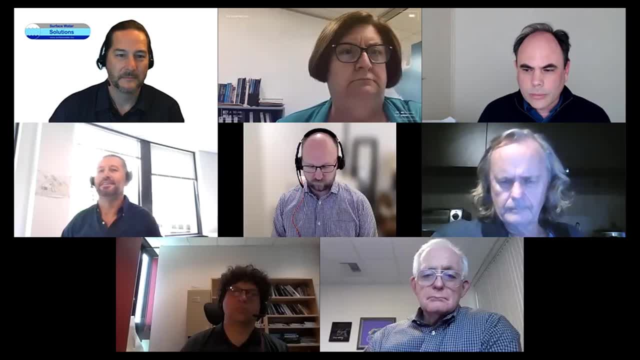 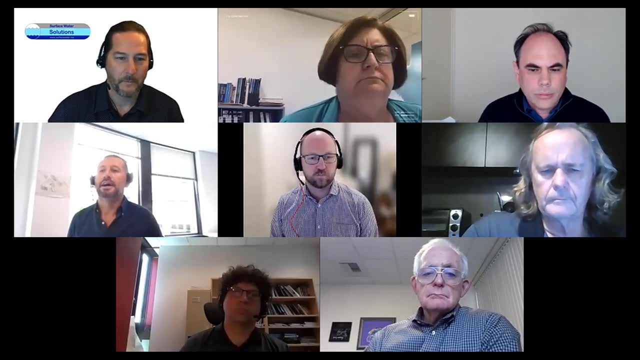 for past data and past extremes, And I know that's very active area research, and so it's really great to do your own literature reviews there, But also if you're depending on how far back you need to go for your purposes. 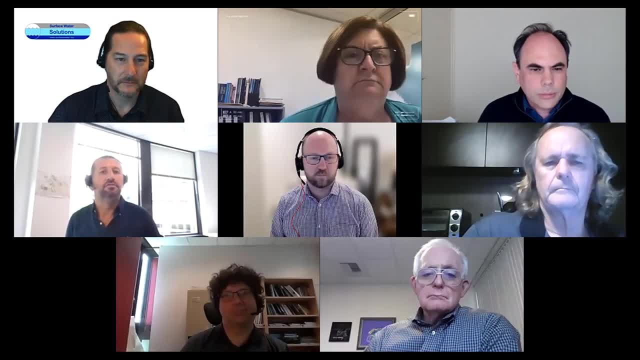 there is greater data coverages across Australia from 1900 for rainfall and there's other data sources within the Bureau to access as well, And I'd really refer everyone to the Climate Change in Australia portal, which is a Bureau-SARO collaboration. 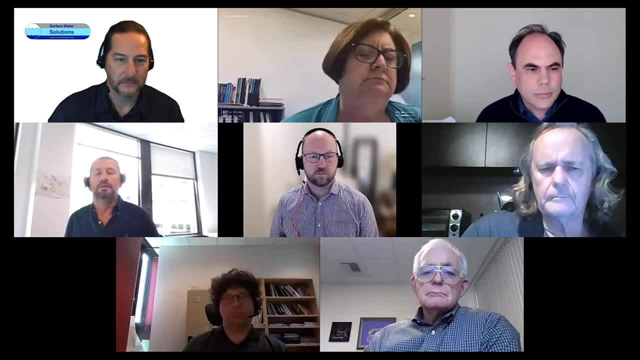 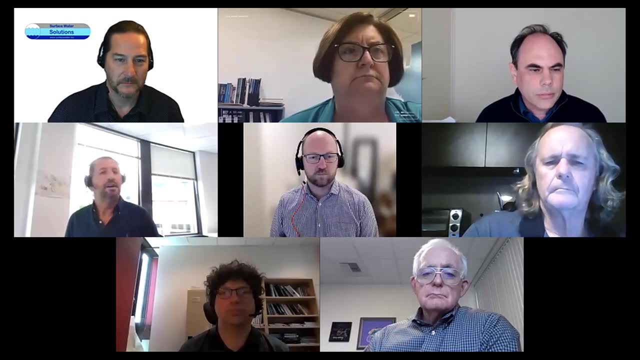 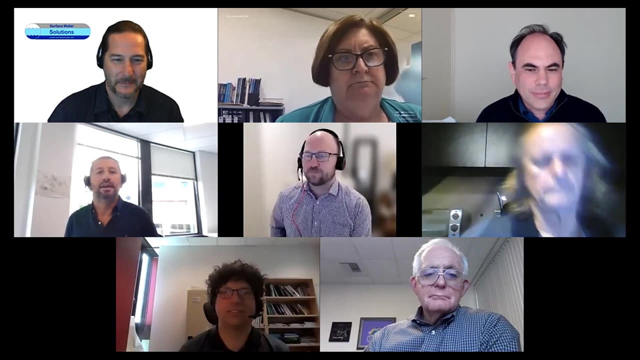 for further data there. There's a lot of information and some good links to literature for both past, climate and future. Can I ask a quick question, Oh, yes, Of the panelists? I would love there to be a discussion around what happened with Hurricane Harvey. and the stalling of the hurricane over Houston. We had a similar circumstance with Dorian stalled over the Bahamas, And I think the same thing kind of happened with Florence stalling over the Carolinas. So three instances of very big synoptic systems. 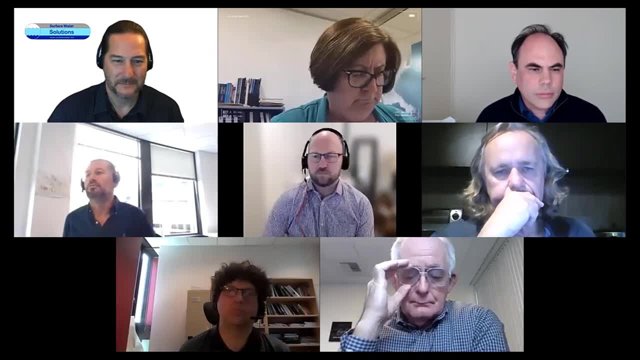 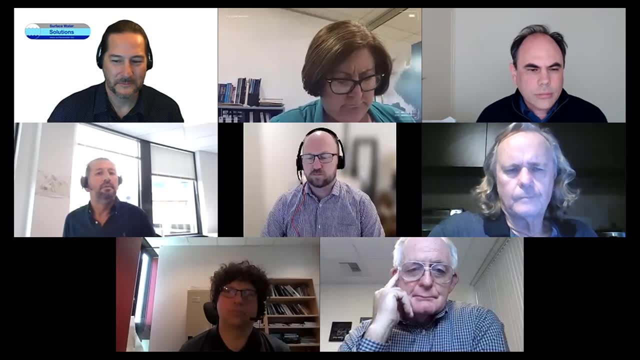 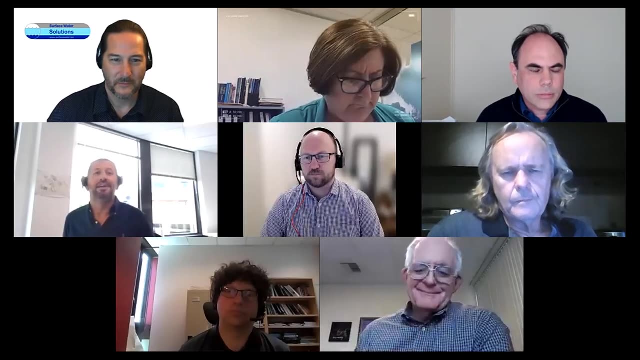 and hurricanes stalling or moving very slowly across areas of the US- And I think this is a relevant question for all areas of the globe, especially tropical and subtropical climates- is that, could that be something we see more of in the future, And what would that mean for PMF and for engineering? 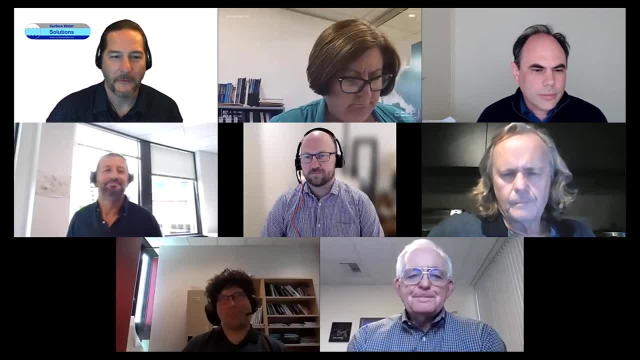 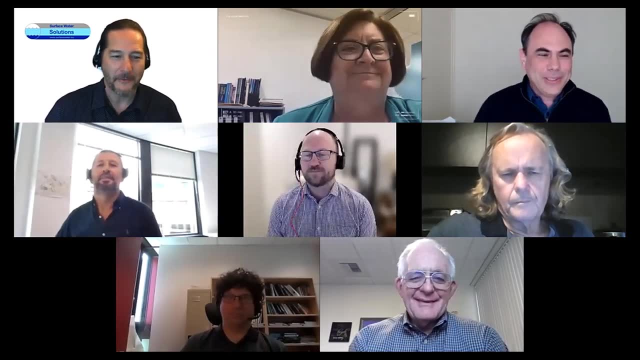 Because that would be a very big impact, I imagine. All right, And having referenced the US, let's maybe have our US attendee here. Despite my accent, I'm still from the other side of the world. here We've got David coming on. 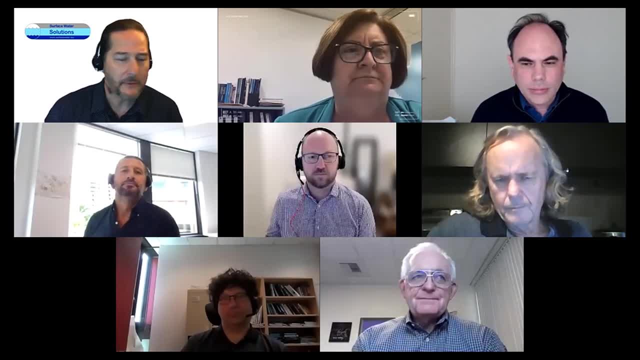 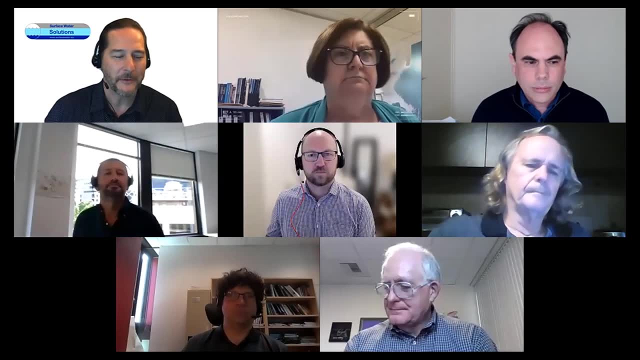 And again we'll just over to the presenters. I think, Janice, we gave you a chance to answer one question. We'll probably close off with this here, David, if you answer that question, and then we'll have Jason. have one last one? 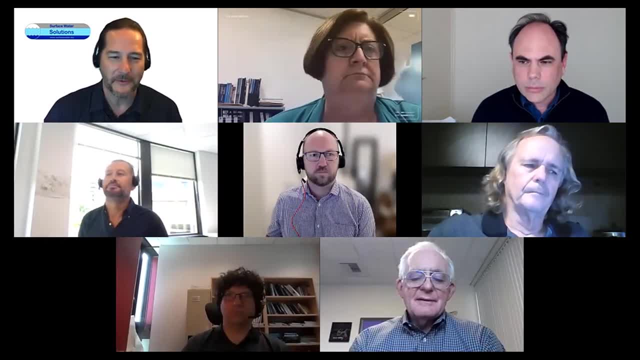 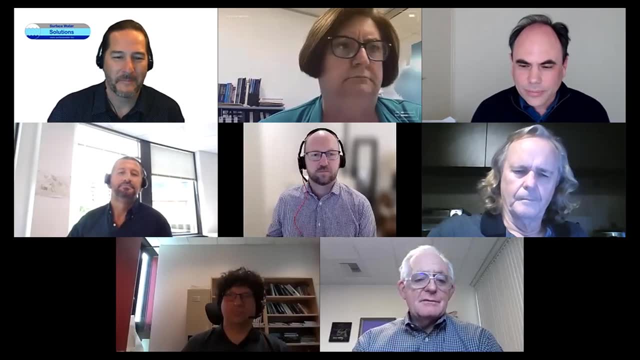 and then we'll probably need to wrap it up from there. So, David, any response to Clinton's question there? Yeah well, I'll take a whack at it. The interesting thing about Harvey relative to the probable maximum precipitation is that kind of the fundamental concept. 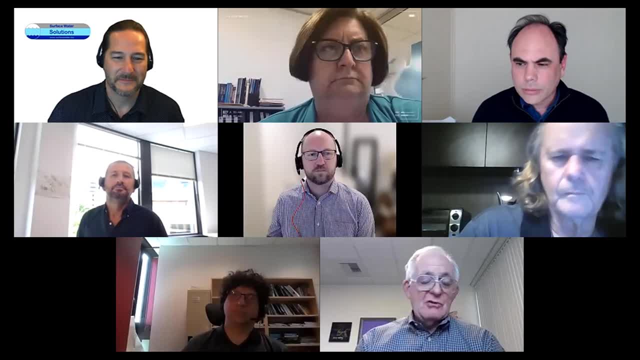 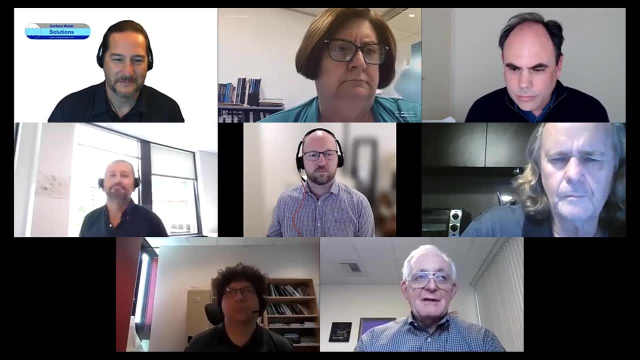 behind the probable maximum precipitation. that number is so large that we'll never ever achieve it. The problem is we did come pretty close in Harvey, And so that's caused a lot of people to completely rethink about you know what's it mean to optimize the parameters? 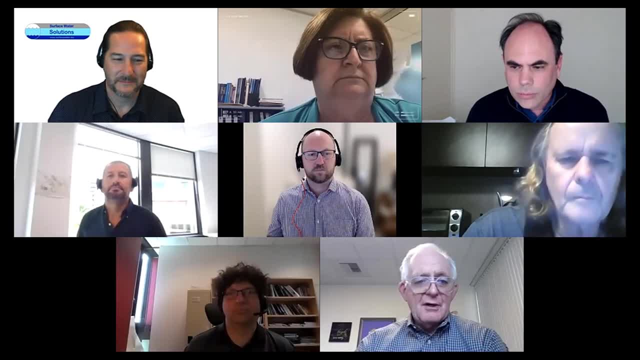 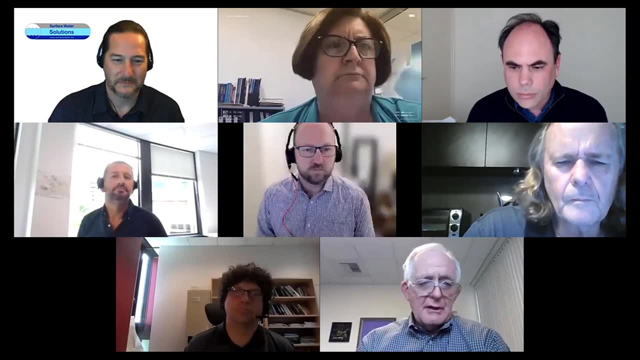 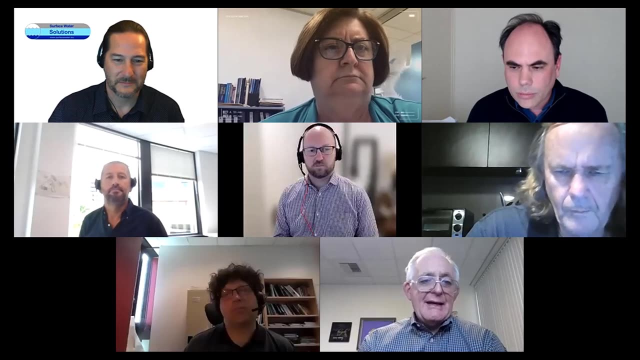 in a meteorological model to generate the rainfall and the amounts that occurred there. Interestingly enough, the short-term stuff wasn't all that high, but it was the accumulation by the fact that the hurricane stalled out, And day after day after day, you've got really high amounts. 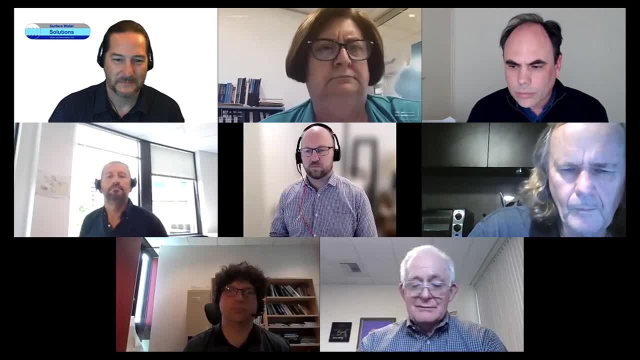 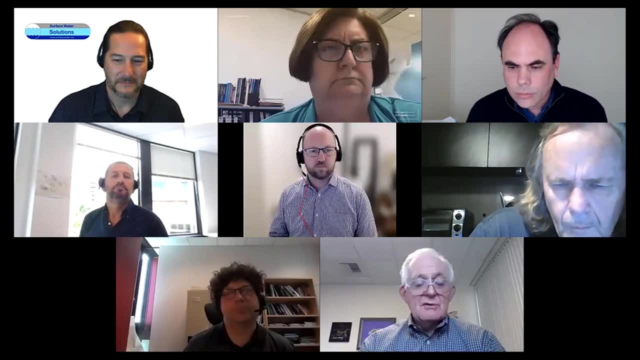 and eventually it accumulated high enough that it caused massive, massive problems. And the evidence that I've seen so far in some of the climate change research relative to tropical cyclones is that they're going to slow down. And if that's the case, 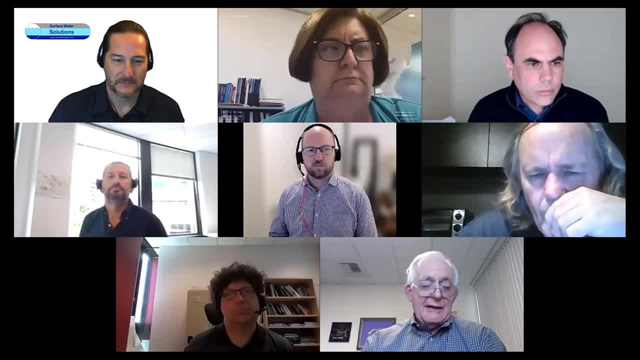 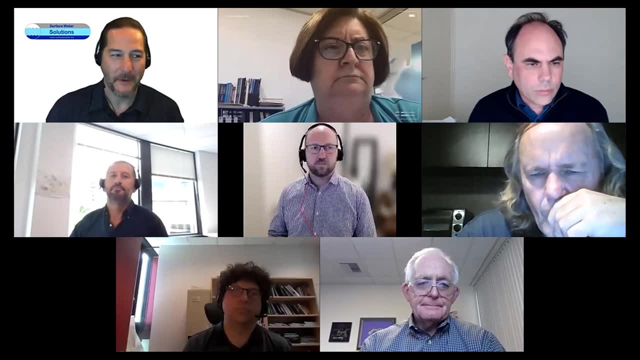 and they maintain any sort of intensity, then we're going to get larger storm totals. That makes sense. That's the yeah, that's the mass balance You've got to get. that that's going to increase in volume over time. 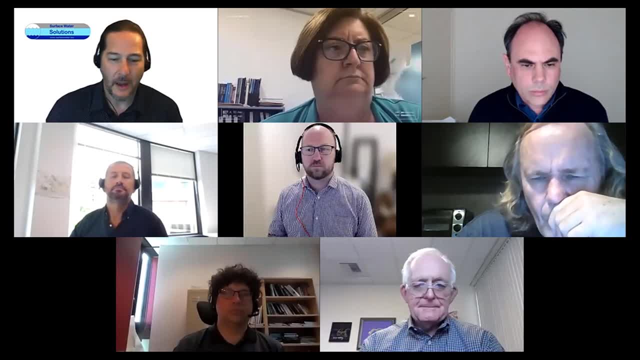 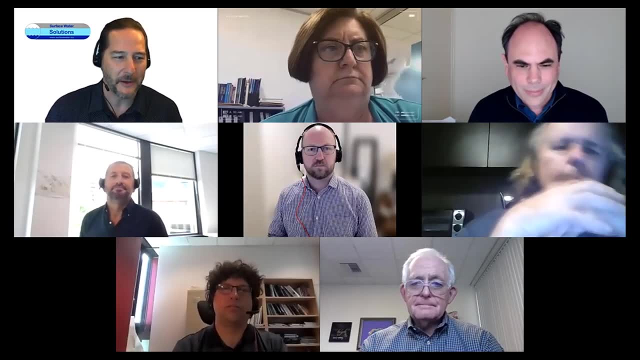 That just makes sense from that standpoint. So thanks for that explanation. Again, thanks for everyone who's answered these questions so far. Jason, we'll have one. we'll give you the chance to close out with one last question and then we'll go on to the housekeeping items. 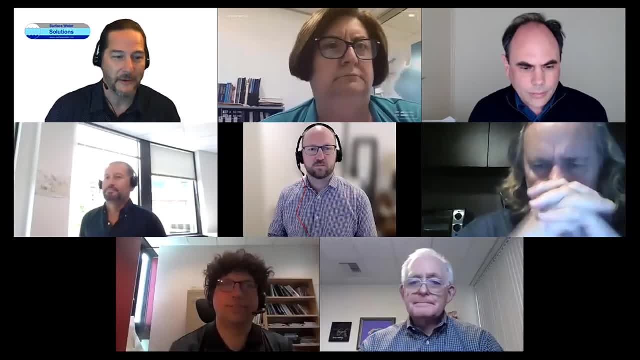 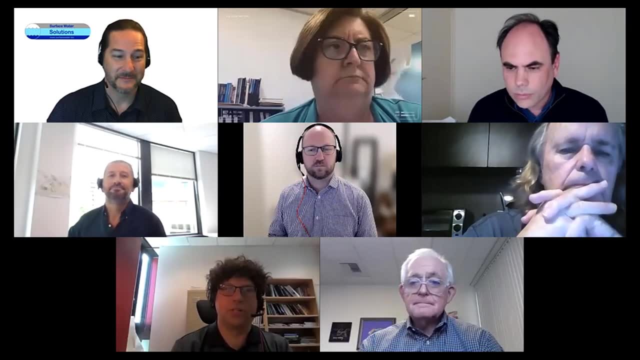 and the courses and webinars that are available to you in the future. So, Jason, anything you've hit that you want to highlight. Well, I thought I might just add to what David's answered for that Clinton's question. there, I think the evidence at the moment. 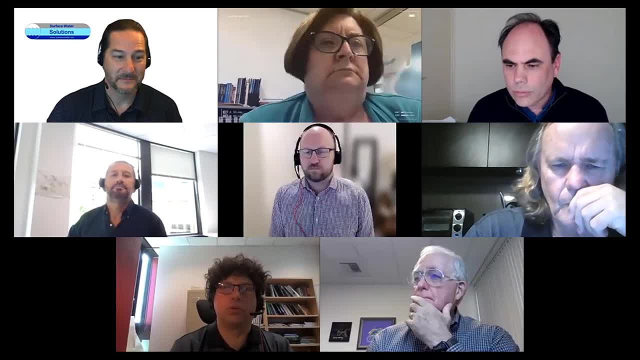 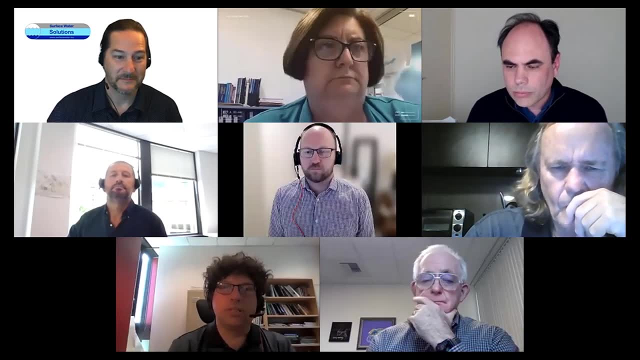 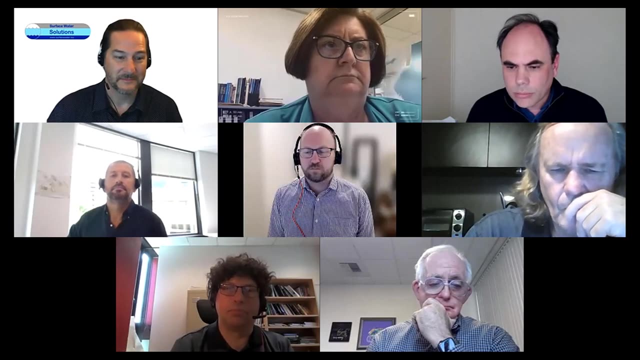 is still a little bit unclear about whether we should expect these sort of blocking situations to be more frequent in the future, But what we do see is with generally more energy in the atmosphere, we get more variability, And that means there is probably going to be more opportunities for stalling to occur. It doesn't mean that all hurricanes will stall or anything like that, but there's probably an increased chance that some will, And if they stall in the right place, like Harvey did, so that the inflow is coming over a really warm water body. 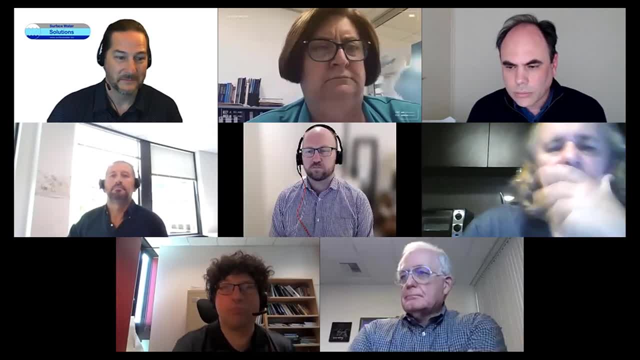 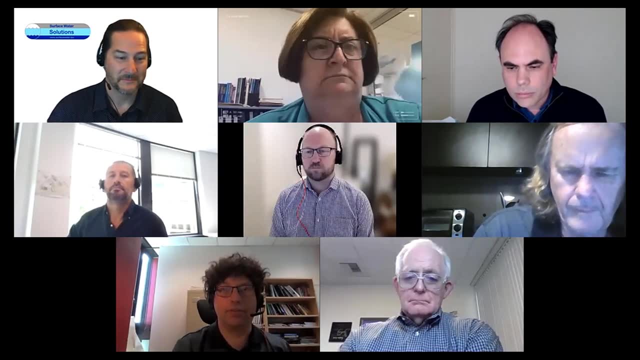 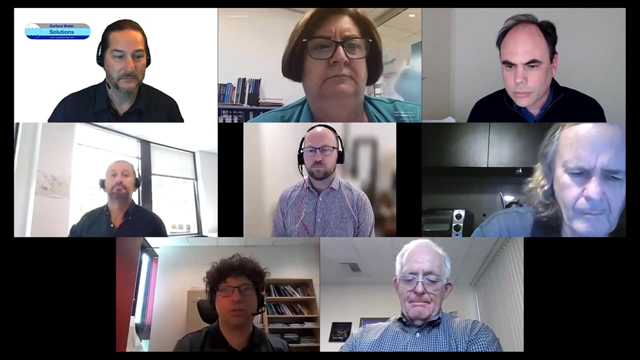 so you're guaranteed to have saturated inflow that can persist for days. then you'll end up with these kinds of situations where you have really heavy rainfall that just keeps going- Excellent, And those warm water bodies are going to be more common in the future. 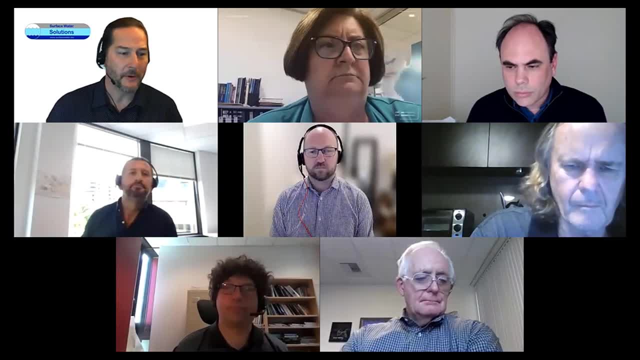 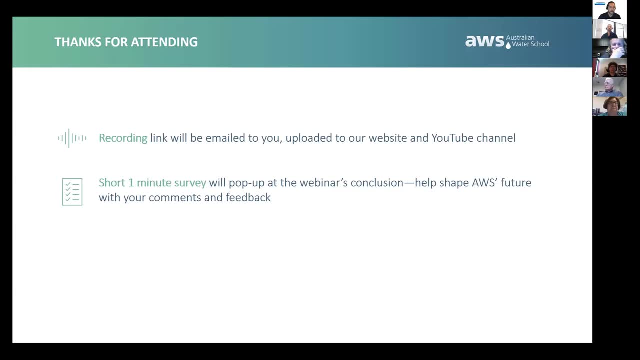 Yes, Well, thanks for that. It's an honor to be part of this panel or to be amongst the experts here. This is again something that some questions that I wanted to get answered for myself. You have got webinars, free webinars. 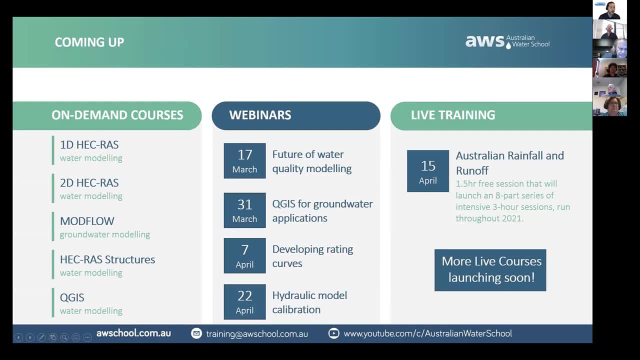 some courses to sign up for. If you see this list here, in modeling and practicing some of these things, putting your model in and, as some of the presenters mentioned, doing a sensitivity analysis, Let's run these models that you can get some help setting up here in our courses. 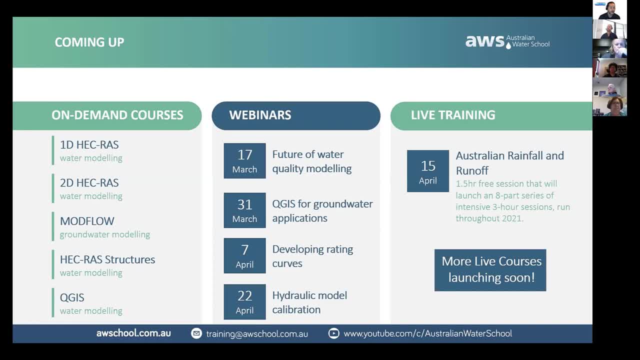 and then let's tweak them and let's see what happens under climate change scenarios. Run these sensitivity analyses. So we've got some exciting webinars coming up as well on water quality running QGIS for groundwater applications, rating curves, taking stage information. 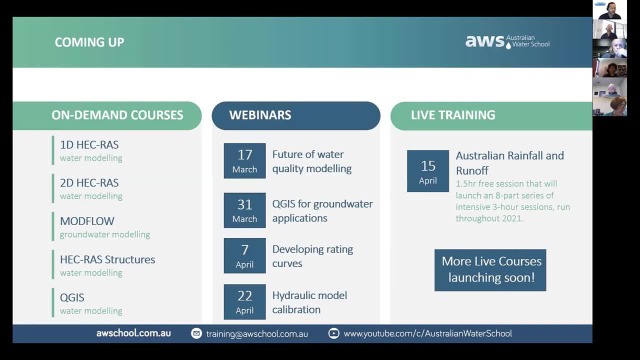 and turning it into discharge and then calibrating your hydraulic model. These are things coming up for practitioners. That's what we put on the agenda. What do you want to hear about? So do fill that out for us on your survey. 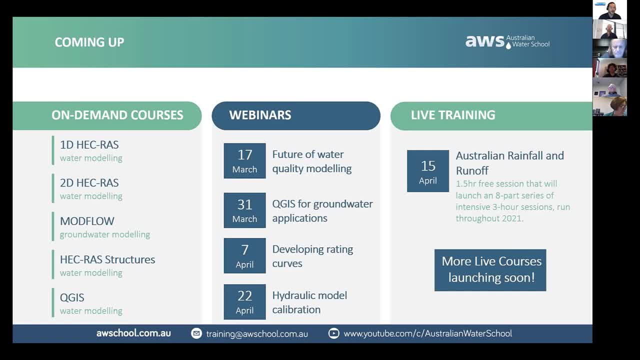 Let us know what you want to hear. We've got Australian rainfall and runoff. Those of you from Australia who want to know how to put these things into practice specifically for Australia, we have got another Australian rainfall and runoff webinar kicking things off. 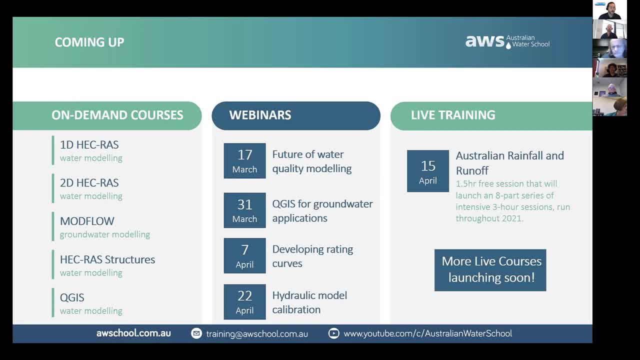 and a series of courses for how you can actually do this yourself. Not just the theoretical bits, but let's implement some of these things in some hands-on workshops. So thank you so much to all of the presenters, the panelists, those in the background answering questions. 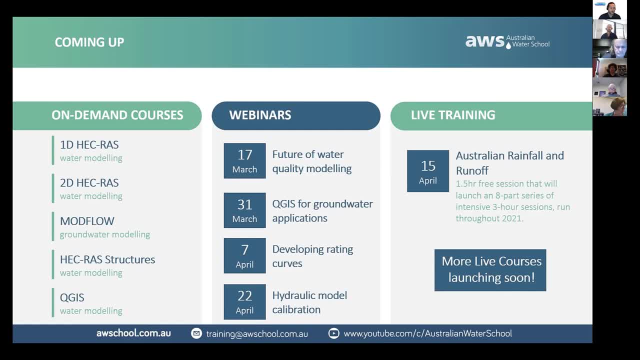 We'll try to get this out to everybody so that you have these resources available to you in the future going forward. So with that we'll sign off here. Thanks so much to all the attendees. We'll see you next time around. Bye-bye. 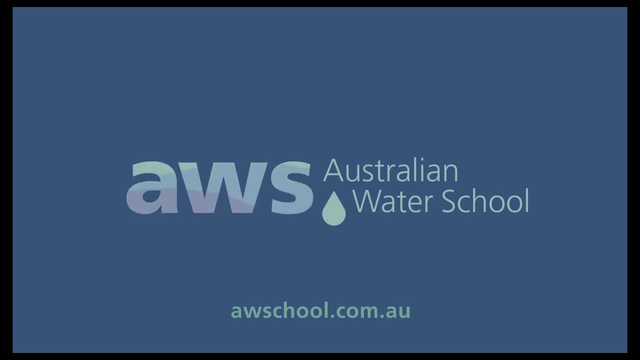 To learn from leading experts in water, visit theaustralianwaterschoolcomau and discover our online training courses, both live and on demand.